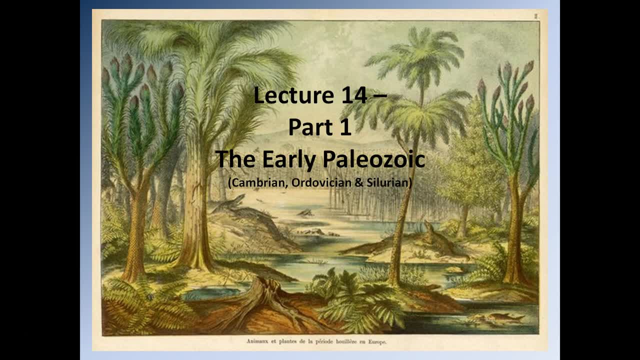 to be looking at the evolution of the continents, with a special focus on what's happening with North America. So we're going to start with the early Paleozoic and that's going to be the Cambrian, Ordovician and Silurian. So okay, so by this point we've made our way all through the 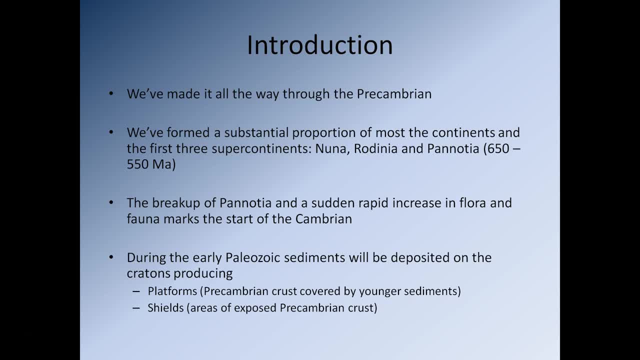 Precambrian and we've formed a substantial portion of the most of the continents, and the first three supercontinents have also formed. So we've had Nuna, Rodinia and Panatea. So Panatea existed between 650 and 550 million years ago and it's the breakup of Panatea that helps to 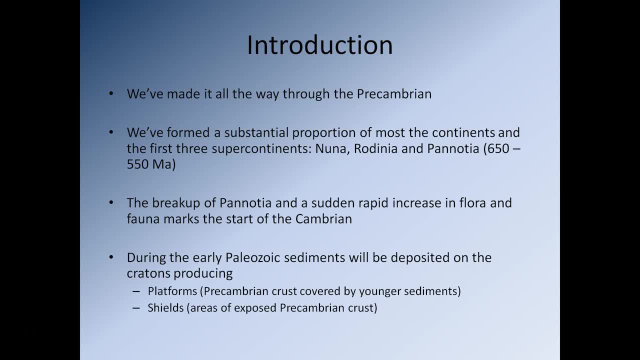 there's one of the reasons that we can mark this transition, So the beginning of the transition between the Protozoic and the Paleozoic, So between the Protozoic and the Cambrian, So the breakup of Panatea and a sudden, rapid increase in flora and 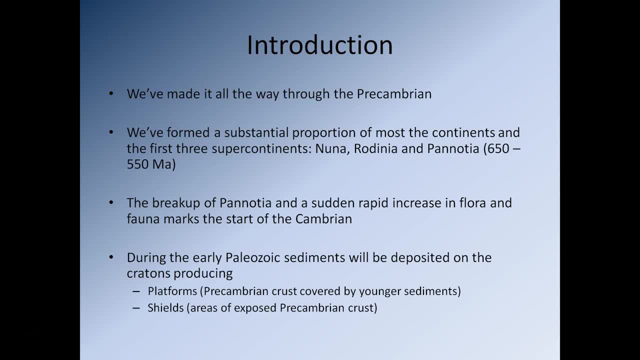 fauna marks this transition. So during the early Paleozoic sediments will be deposited on the cratons, producing platforms. So of course, those are areas where we have Precambrian crust that's covered over by younger sediments And shields. those are areas where we have Precambrian 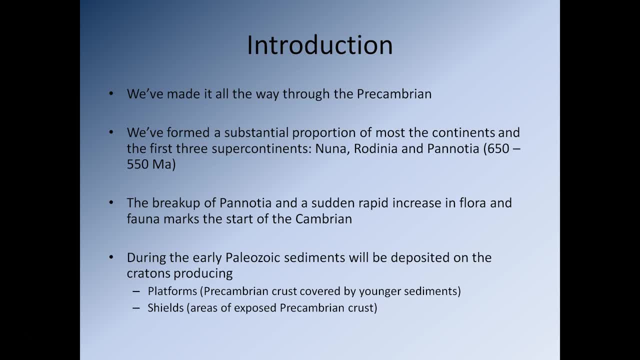 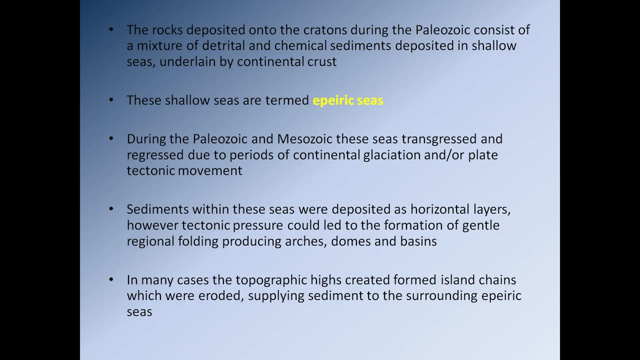 crust that is exposed. so remember that. so we have platforms- that's where the precambrian crust is covered up- and shields where the precambrian crust is exposed, and of course, those two combined is referred to as the craton. so the rocks deposited onto the craton during the paleozoic consist of: 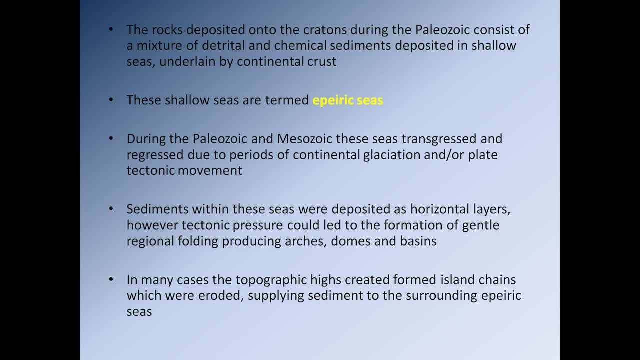 a mixture of detrital and chemical sediments deposited in shallow seas underlain by continental crust. so what we're going to see as we move through the paleozoic is we're going to see on four occasions: a significant portion of North America is going to find itself underwater. the 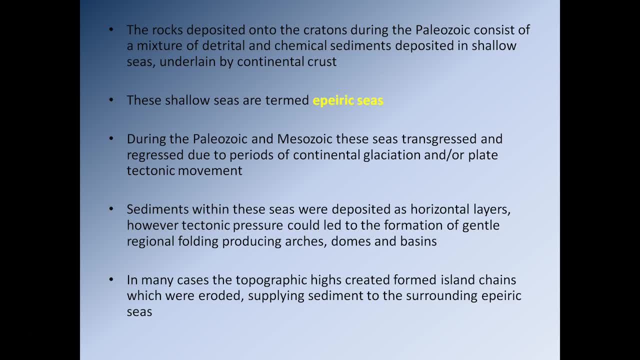 sea level is going to rise and the continental crust is going to be inundated, and this process of inundating the continental crust is going to produce lots of shallow seas, and these shallow seas are called epiric seas. during the paleozoic and the mesozoic, these seas will transgress and 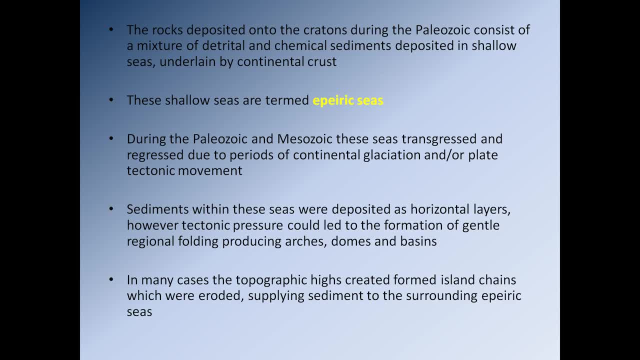 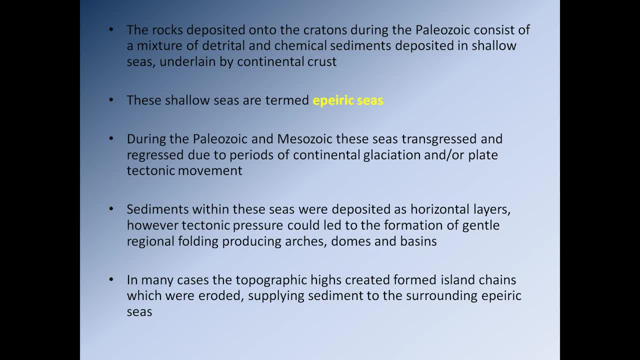 level is going to go up and down during the paleozoic and that's obviously going to have a serious implication for, you know, whether the ocean is kind of moving onto the land or wherever it's retreating back into the ocean basins, so sediments within these seas would 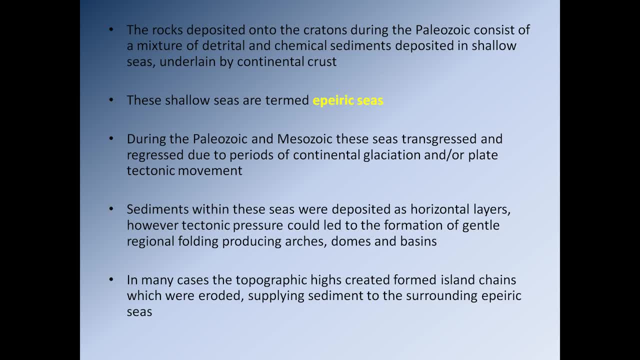 have been, of course, deposited as horizontal layers. however, tectonic pressure could lead to the formation of gentle regional folding produces producing features like arches, domes and basins. so you know, bear in mind, you know it would have been nice horizontal sheets, but of course, 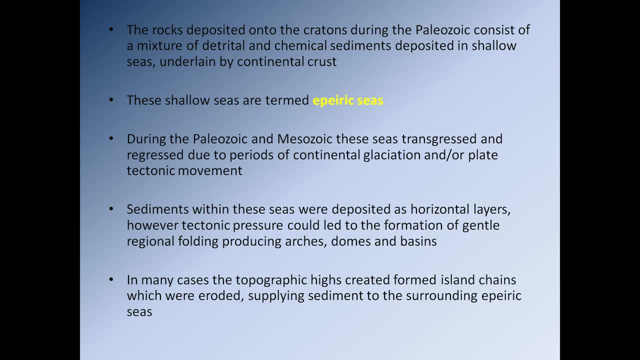 during that time there would have been tectonic forces going on that will have caused these nice horizontal layers to warp. so in many cases the topographic highs created will form little island chains and these would be eroded and they would. that would supply sediment into the surrounding. 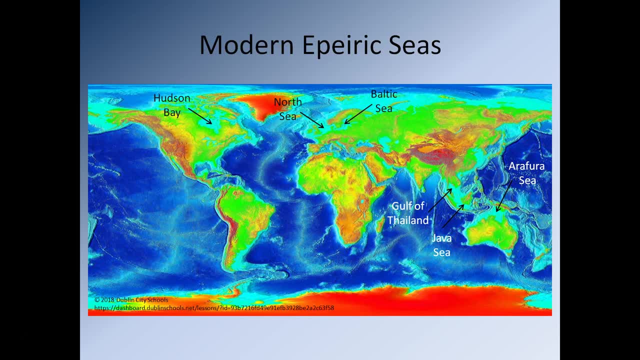 epiric seas. so are there modern epiric seas? well, the answer is yes. so if we look at a few examples, we have the Hudson Bay up here, so it's shallow water underlain by continental crust. we have the North Sea in Europe, we have the Baltic Sea, we have the Gulf of Thailand, we have the Java Sea. 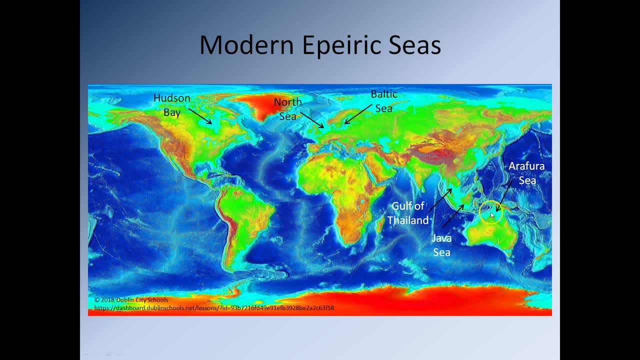 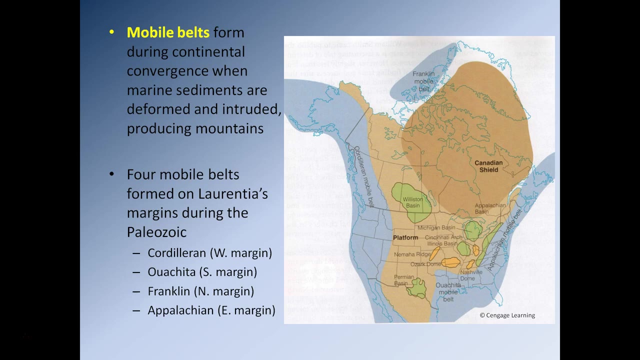 down here and we have the the Athera Sea here between Australia and Papua New Guinea, and so you can see that these areas of continental crust that are inundated still exist even now. now, another thing that we need to remember is the term mobile belt. so mobile belts form during continental convergence, when marine sediments are deformed. 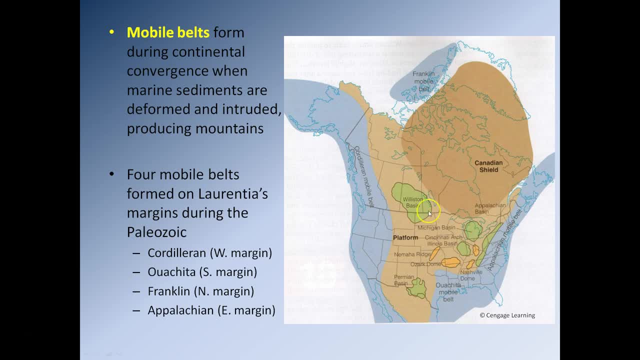 and intruded, producing mountains. so if we look at this map here of North America, what will we see? well, we can see essentially we have four distinct mobile belts that are picked out by this particular diagram. so we have the Appalachian mobile boat running down the eastern seaboard. 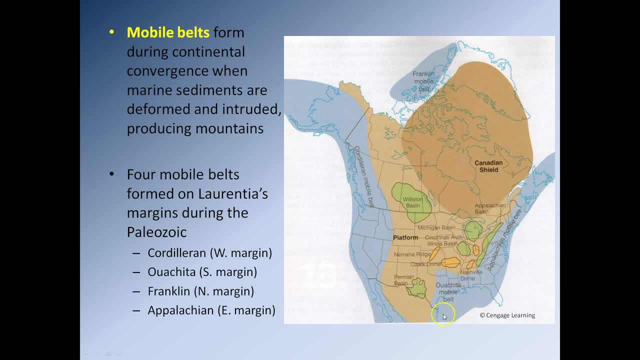 we have the Cheaton mobile belt down here, covering the portions of Texas, Oklahoma and Arkansas. we have the Cordillera mobile belt running up the western seaboard, and up here we have the Franklin mobile belt, also called the Inuitian mobile belt, which is occurring up here along the northern margin of North America, and so these are areas where 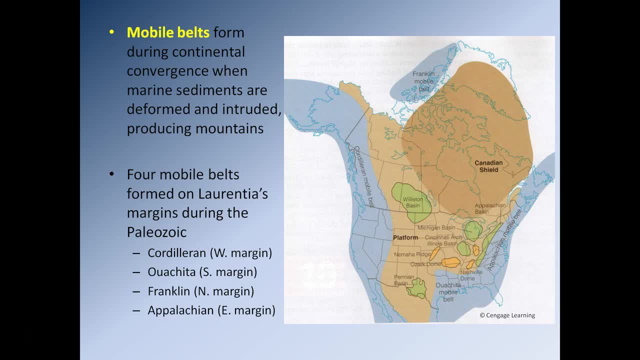 continent-continent collisions or collisions between continents and island arcs have produced, essentially, mountain ranges, and the reason you know they're referred to as mobile belts is, of course, the belts themselves. they shift. the mountain range isn't actually stationary. depending on you know. you know where the, where the, where the impacts occurring, and 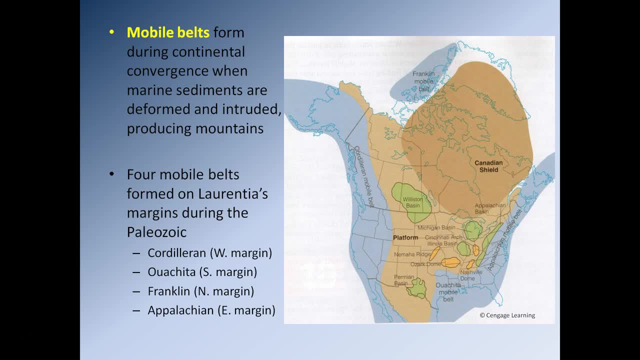 how you know forceful the impact is or whether the impact is waning. essentially, that will control how the mountain belt essentially is the morphology of the mountain belt and so the mobile, the mountain belt itself will shift and will move around to some degree. so we need to bear this in mind, so not only. 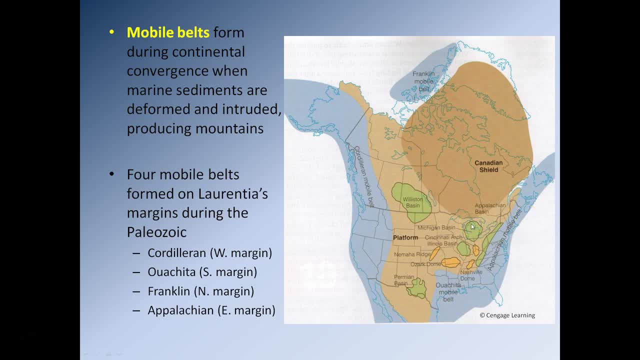 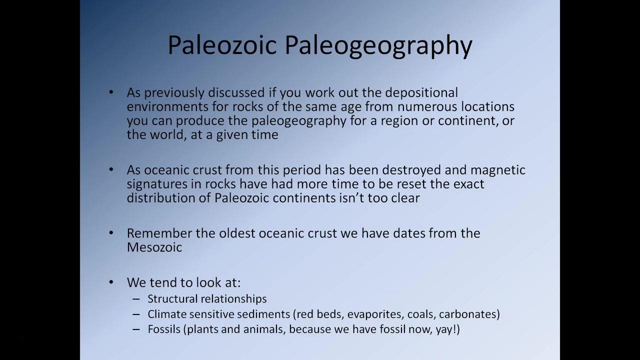 do we have during this time period? we have the deposition of lots of nice horizontally bedded settlements in the shallow seas, covering large portions of North America. we also have the formation of several large mobile belts along the eastern, southern, western and northern margins of the continent during this time period. so it's all going on. so what's happening in terms of? 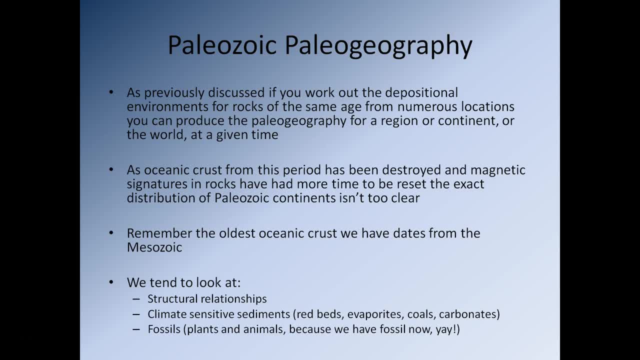 paleogeography. so, as previously discussed, if you work out the spatial environments for rocks of the same age from numerous locations, you can produce a paleo. excuse me, you can produce a paleogeographic map for a region, a continent or even the entire world, given time and sufficient data, so as oceanic crusts from this period has been destroyed and 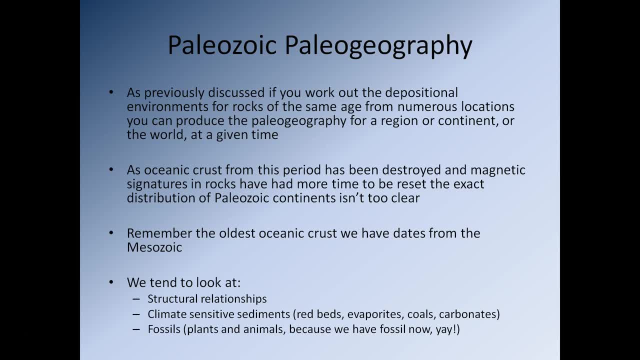 magnetic signatures in rocks have had more time to be reset. the exact distribution of paleozeric continents isn't too clear, so when I show you the diagrams and the paleozeric continents moving around, we have some idea where they are, but we can't be 100 accurate, so we need to remember the oldest. 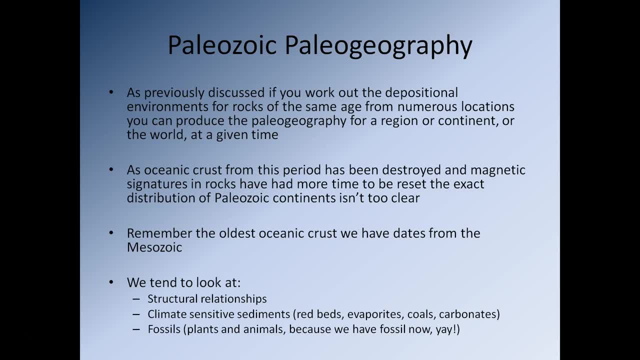 oceanic crust we have dates the mesozoic, so that means any oceanic crust before the mesozoic that's gone, and so that would have been really helpful to have had, because that would have told us which way, you know, the spreading margins were pushing the continents, but unfortunately it's gone. there's. 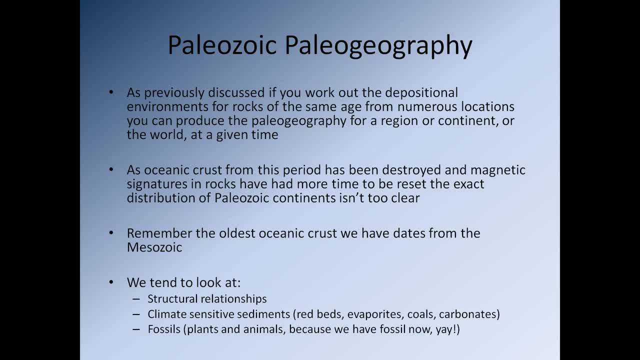 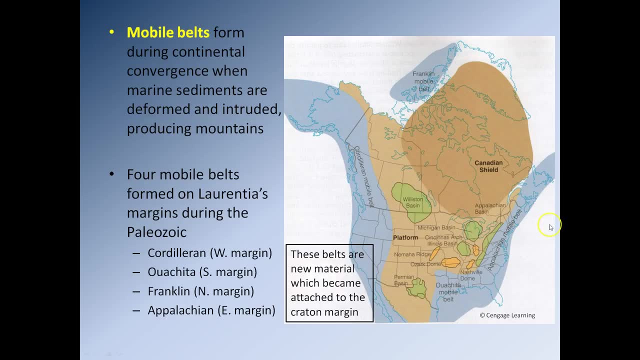 nothing we can do about it. so what do we do? well, we look for structural relationships. so we find out that there are rocks that have been deformed. so, for instance, if we go back to this diagram here, when we think about the uh, the app, the Appalachian mobile belt, we notice that the way the rocks have 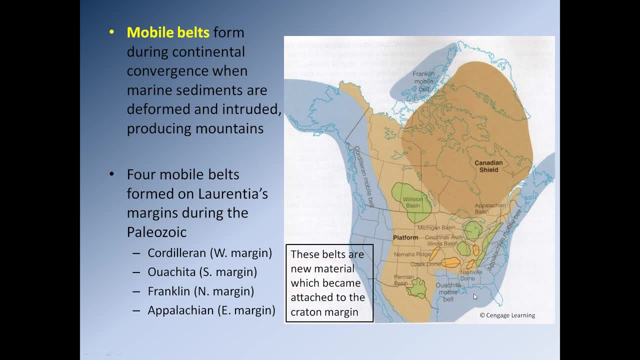 been deformed here is very, very similar to the way that the rocks have been deformed in Northwestern Africa, and that deformation occurred at the same time. so the deformation we see in Northwestern Africa and the deformation we see here along the eastern seaboard occurs at pretty much the 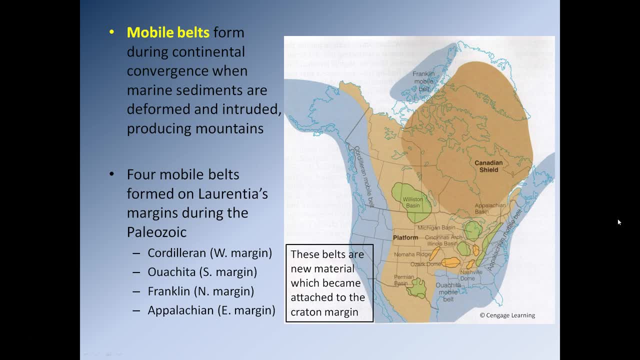 same time, that's a strong indicator that those two pieces of continental crust hit each other. so we can use that kind of relationship to show that right. well clearly, if they're hitting each other, they have to be in close proximity to each other. what else can we do? well, we can look at. 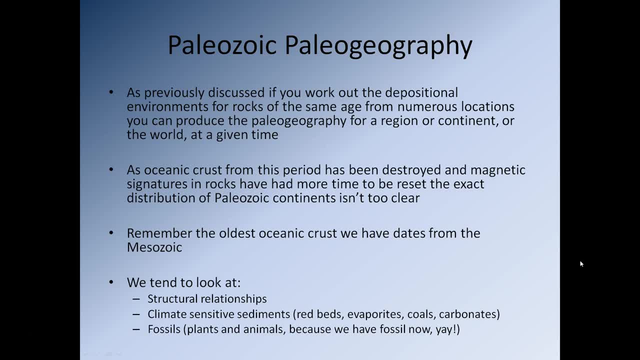 climate sensitive sediments. so there are certain types of sediments, which we've discussed in the past, that can only form under a very strict range of conditions. so red beds: we've discussed how red beds, these red classic sedimentary rocks, tend to be associated strongly with arid to semi-arid. 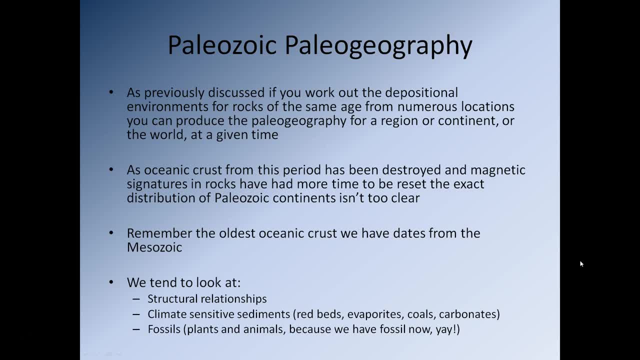 conditions that can only happen, only be produced where you have bodies of water evaporating away once again, where you have layers of evaporites that tends to suggest you are in dry or arid to semi-arid conditions, so that tells you about somewhere where you are on the surface of the 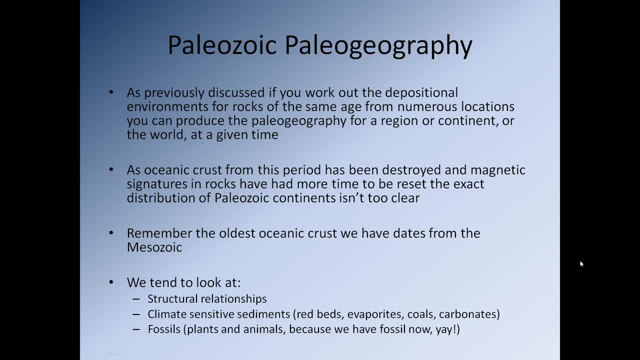 earth. so you know, you know there are only certain regions of the earth where you know, based on circulation of the atmosphere, that will tend to be drier and therefore more likely to have deserts in them, and so you can say: right, chances are the continents were in one of these regions. 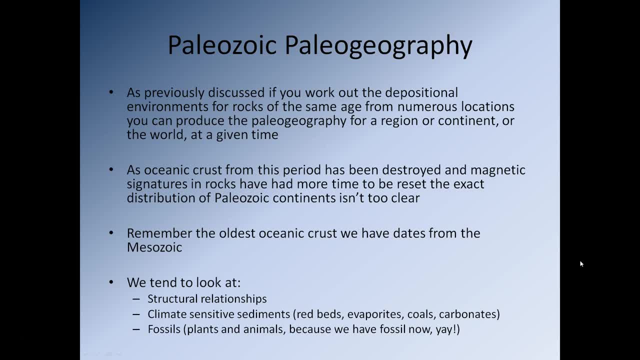 then there's, you know, some sediments like coals. well, coal only will tend to form in swampy environments that have a very, very high amount of organic material. well, that tends to occur in equatorial regions, so typically regions, you know, 30 degrees north or south of the equator. so as soon as you find a, 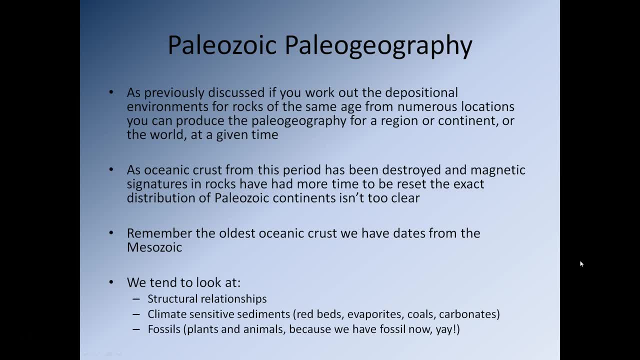 coal layer and you can date that coal layer. you can say, right at this point in Earth history the continent was probably somewhere in one of these regions. and of course there are carbonates. carbonates tend to occur, um in, once again, very relatively warm shallow seas located typically 30 degrees north or south of the equator. 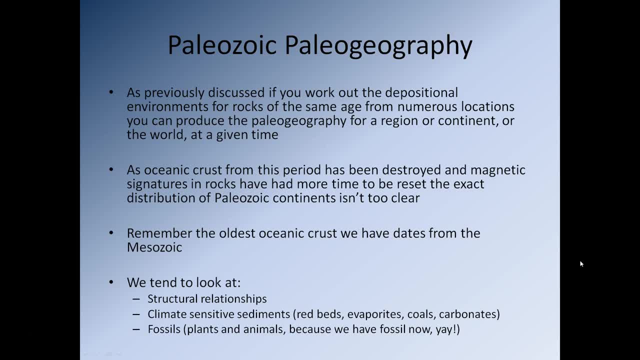 so once again when we start finding carbonates in our rock record that suggest that in all likelihood, at that period of time the continent was located somewhere near the equator. and now, of course, we also have fossils, and some fossils will have very distinct environments in which they like to live. 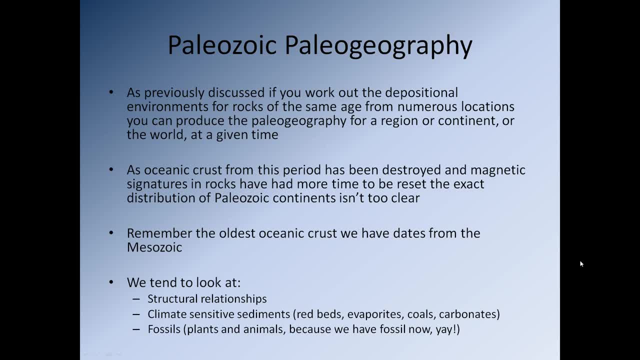 so of course it's going to give you some information. so, for instance, a dinosaur. you know dinosaurs did not live in water. so if you find dinosaur fossils in your sediment, you know you have to be looking at a continental sediment, you know. then there are certain organisms like 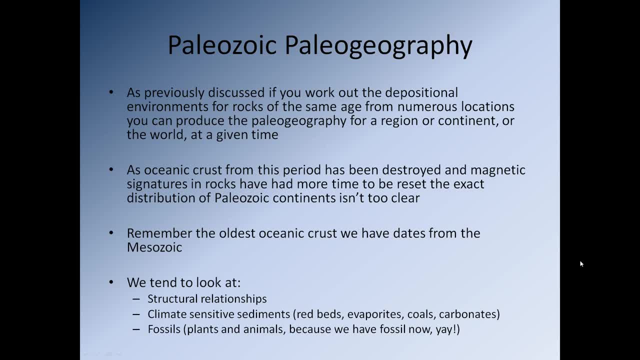 foraminifera that can only exist in. you know the certain species of foraminifera that will only exist in certain water temperatures. you know certain water salinities you know. so that will also help us to gauge where we are on the surface of the earth. so there's lots of information that. 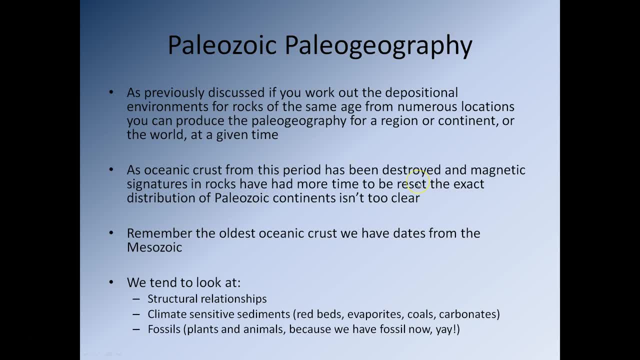 we can work with. you know we can also use paleomagnetism to work out where continental rocks form. that'll also help us a little bit. so using all this information and lumping it together, we can work out with a relative degree of certainty where the continents were on the 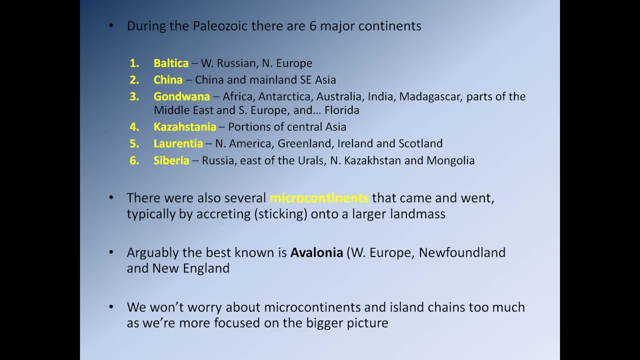 face of the planet at any given time. so during the paleozoic, we know, there were six major continents: baltica. so that's western russia and northern europe, china. that covers an area that includes the gulf of england and the gulf of england and the gulf of england and the gulf of. 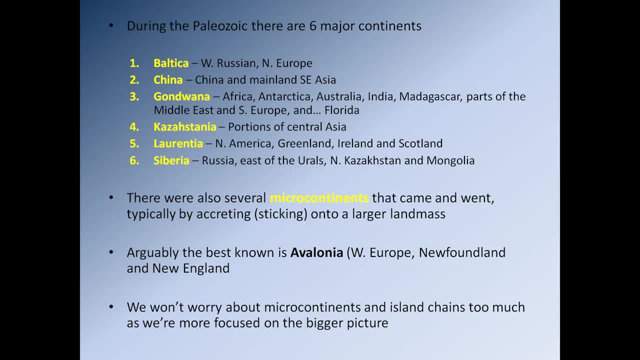 china and mainland south and mainland southeast asia, gondwana, so that's a continent that contains africa, antarctica, australia, india, madagascar, parts of the middle east, parts of southern europe and florida. we have kazakhstania that contains portions of central asia. we have laurentia. 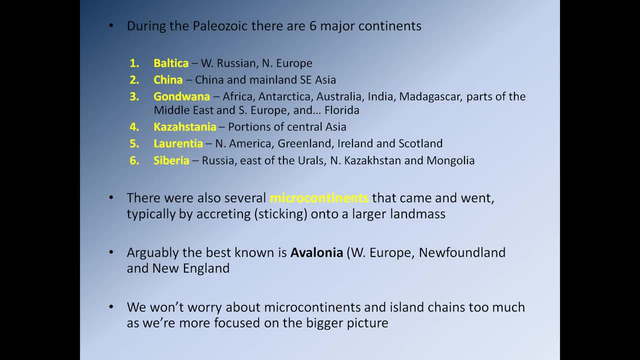 that's north america, greenland, ireland and scotland, and we have siberia, that's russia, east of the urals, bits of northern kazakhstan and mongolia. so you can see there are pretty substantial pieces of crust moving around. there were also several. 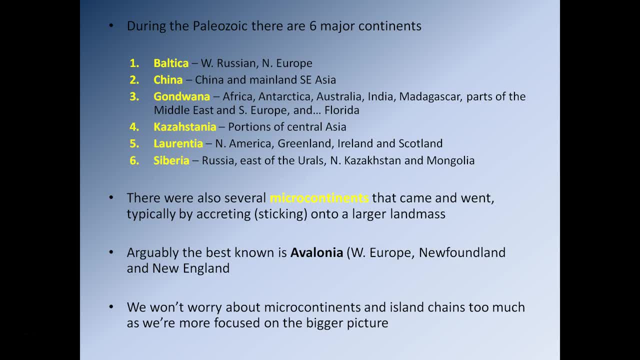 microcontinents that were moving around. now, these microcontinents will have come and gone, depending on whether they're, you know, crashing into the larger continents or not, and, on the whole, we're not really going to worry about them too much. the one we are going to be concerned about, though, is a 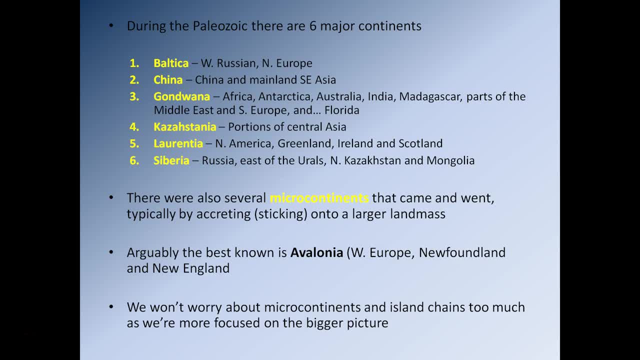 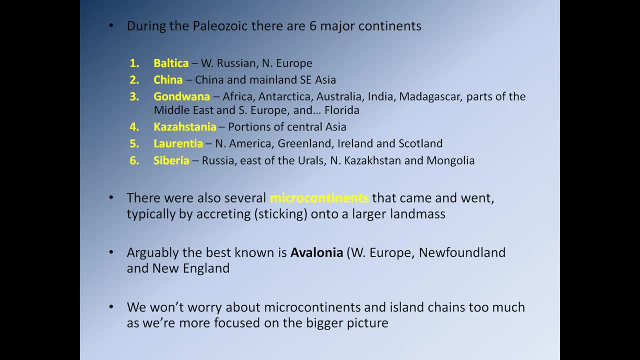 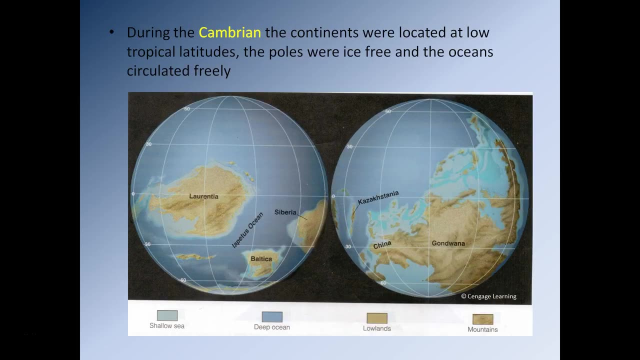 explain some of the stuff that happens along the eastern seaboard of the united states. so we won't worry about the microcontinents too much, as i said, and island chains too much, because we really focus on the bigger picture on the whole. okay, so what's happening? so during the cambrian, the continents, 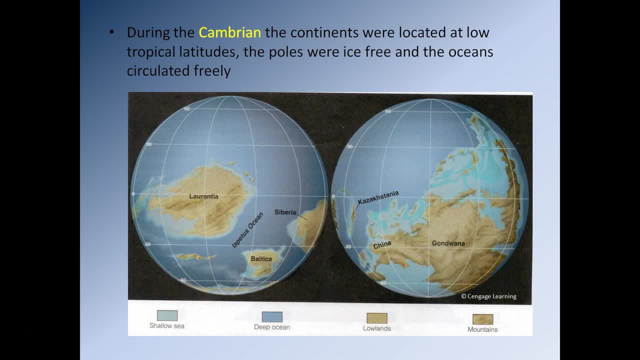 were located at low tropical latitudes, the poles were ice free and the oceans circulated freely. so you know, let's have a look at what's going on. so here's laurentia. so this is now. that's north america. so that's laurentia, which of course consists of north america, greenland. 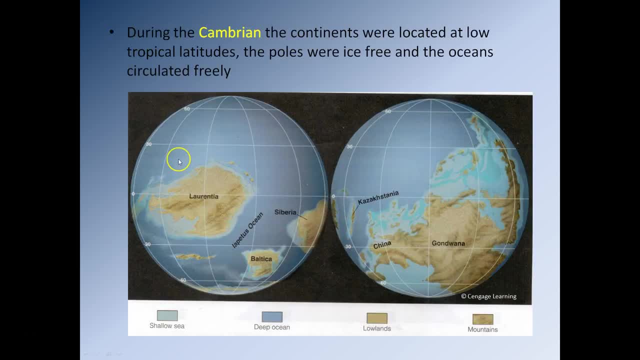 ireland and scotland. so this is where we are, okay, and at that point north america- laurentia is situated on the equator, so we can see we have a few important things gone. so here's avalonia down here, here's baltica over here on the other side. so there's siberia there. we have kazakhstania, here. 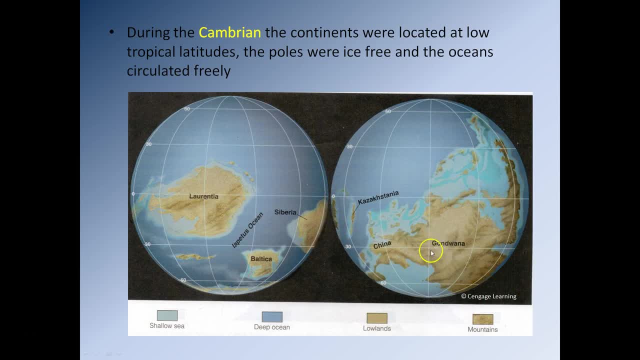 china, and here we have gondwana. okay, and you can see this is a very, very large piece of continental crust here and we can see that it's located essentially in a very high southern latitudes, so you'll notice no ice at either pole. that tends to infer, that tends to 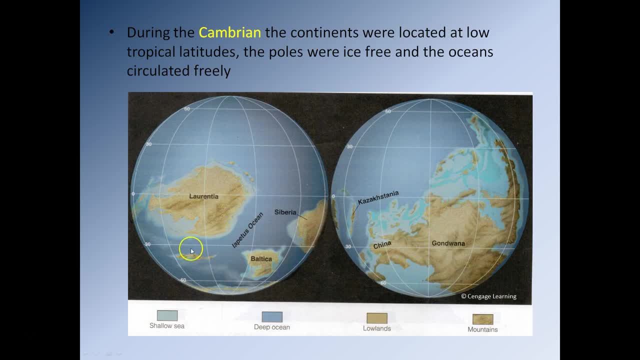 suggest. the global climate was on the whole quite warm, and that will have been helped by the fact that the oceans can circulate freely, so warm water from the equator can move very, very easily towards either pole, and that will help to keep the temperatures towards the poles much, much warmer. 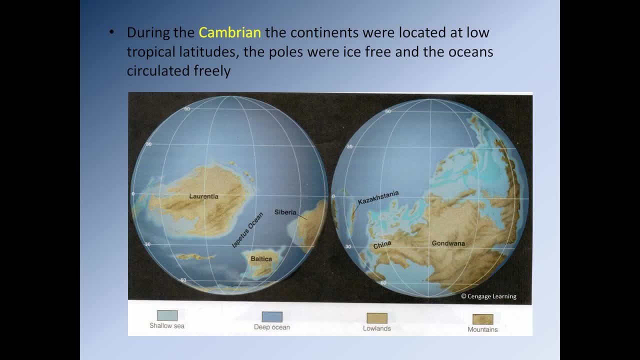 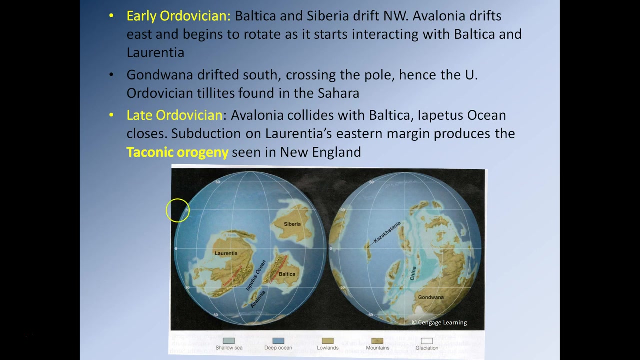 compared to the modern environment where we have lots of continents spread out over the entire surface of the globe that tend to get in the way of ocean circulation and keep the temperatures towards the poles colder. so by the early, or division what's going on there? so by the other. 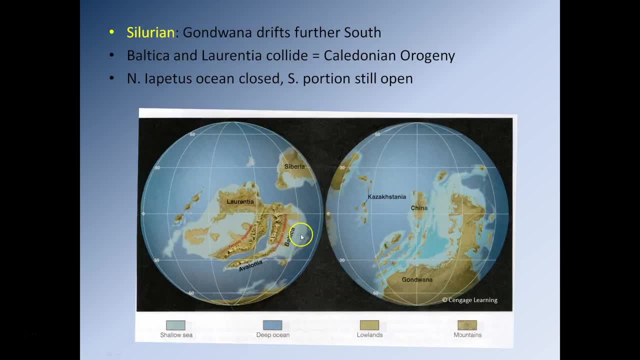 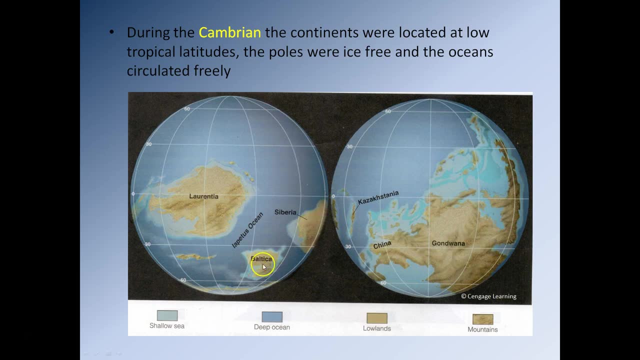 division we have. baltica and siberia have kind of drifted northwestward, so they they're starting off, starting off down here and they're heading in a kind of northwesterly direction. so they're heading this way. baltica is going to come up this way and they're going to come up this way and they're. 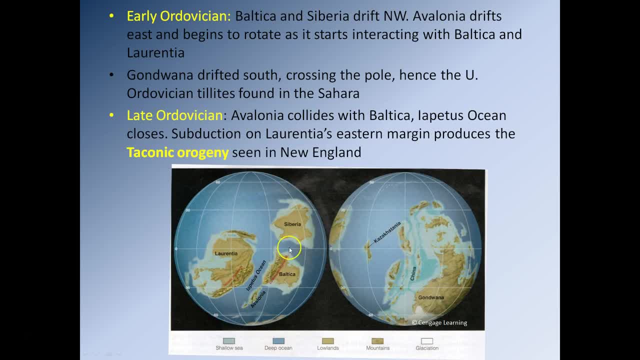 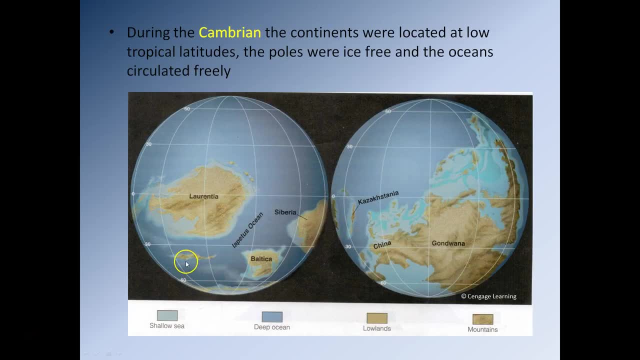 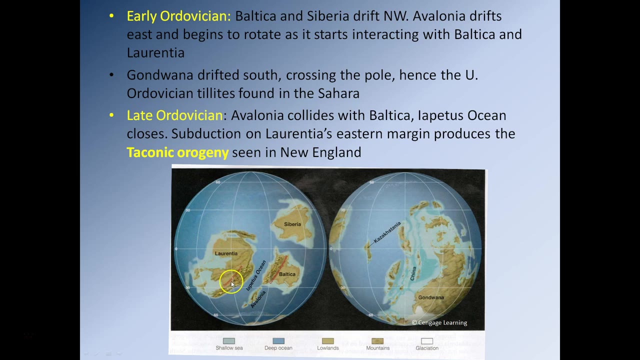 heading this way towards the equator. so here we go. so there's baltica there, so that's moving in a northerly direction. so baltica is coming up this way. avalonia is moving around here like this and is coming up towards baltica as well, and laurentia is staying pretty much where it is it's sitting at. 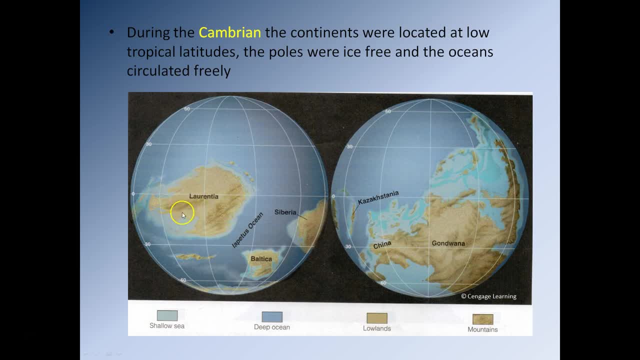 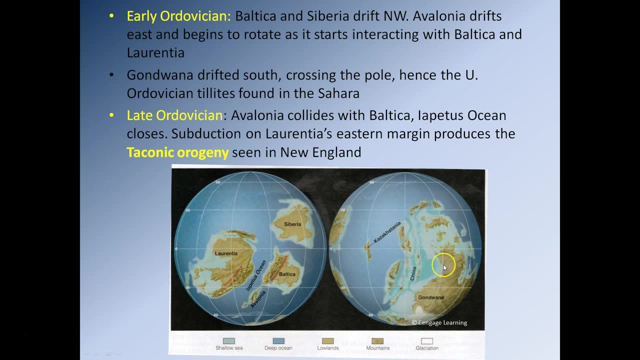 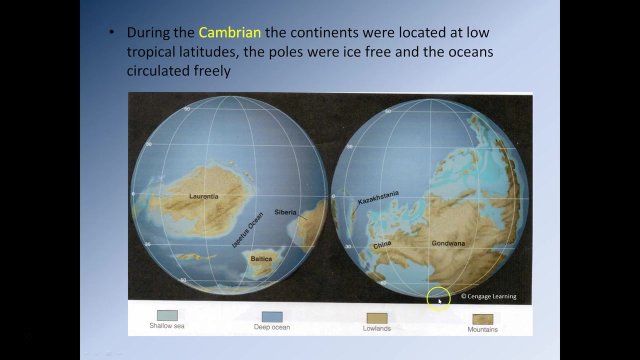 or slightly south of the equator, that's staying, on the whole, mostly stationary. in terms of gondwana, we begin to see gondwana moving down towards the south pole, and what we begin to see is, as gondwana moves down towards the south, 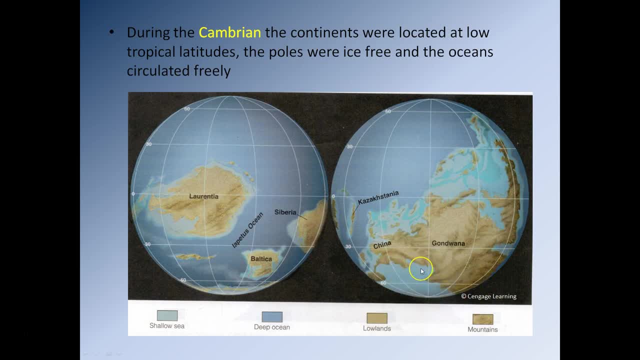 pole, we replace sea. now the nice thing about sea water is it's very, very good at retaining heat. so the sea, the oceans, are far more efficient at retaining solar radiation than the land is. so you know, during the cambrian we had, you know, shallow oceans down across the southern poles. 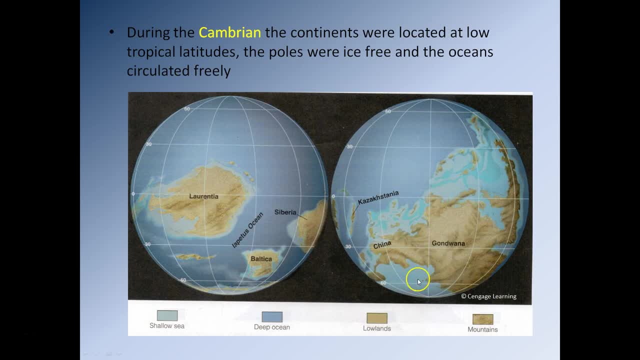 here, and so that will help to keep this area here warm. as you move into the or division, we can see the continental crust starts to drift down. that means less solar radiation is being retained over the southern pole, and so that encourages the formation of ice sheets so we can see glaciers. 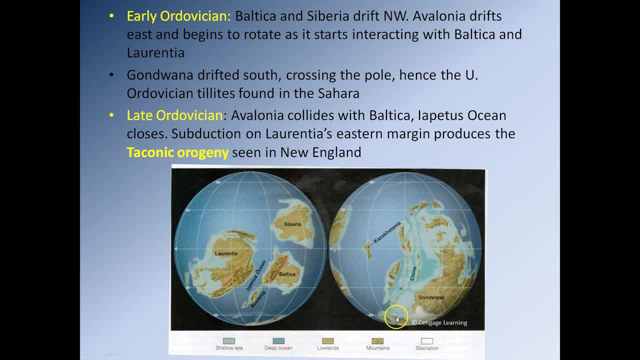 forming, as actually on gondwana, during the order vision. so we see the formation of glacial tills starting. so by the late order vision, we see that avalonia has collided, or is just all about to collide with baltica, forming one landmass, and we can also see that the gondwana is moving in a 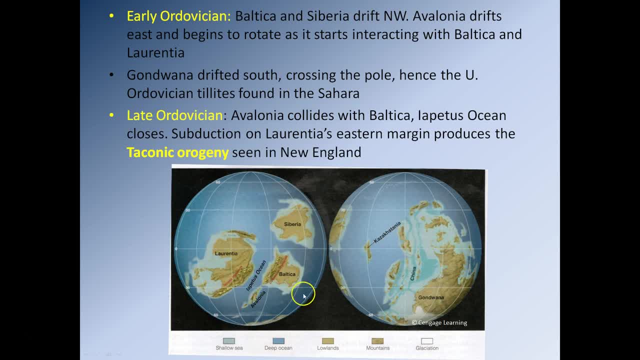 different direction and this body of water here between laurentia and baltica is being destroyed. so the oceanic crust here is being subducted below baltica and laurentia and it's being subducted away, being destroyed, and baltica is moving towards laurentia and laurentia is. 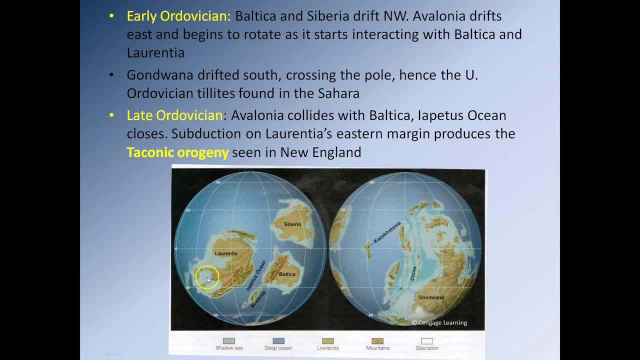 obviously moving toward baltica and there is going to be a big collision and this collision is going to produce a couple of mountain ranges: the caledonian mountain ranges over here on the baltic, on the baltic side, and we have the taconic highlands over here on the laurentian side. 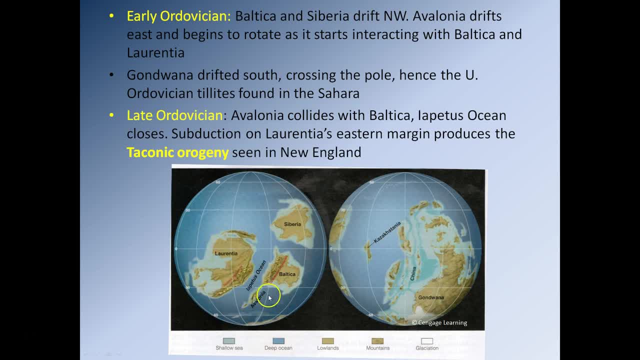 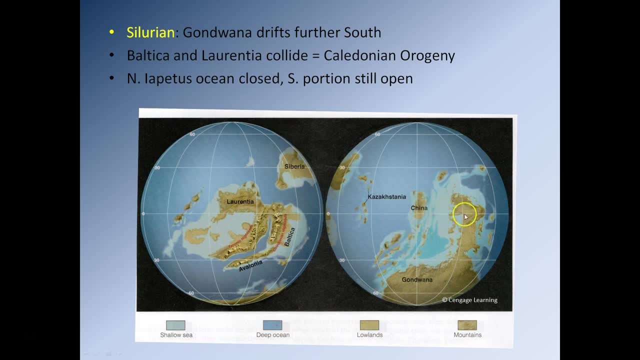 okay, and they're both being produced by this impending collision by the silurian. what's going on? well, siberia's kept moving north. gondwana is still moving south. now we can see we've actually lost the ice cover here, so that would rather imply that global. 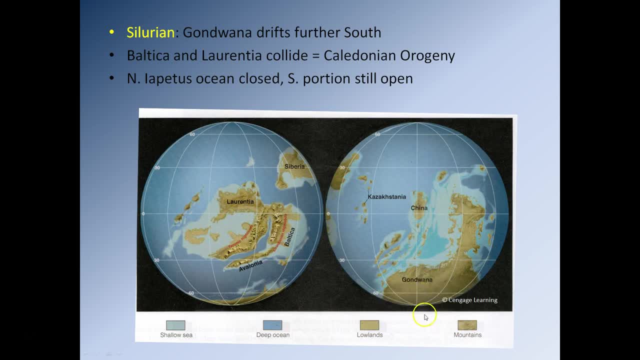 temperatures have increased again, making ice cover along on the south pole difficult to achieve, and we can see by this point the iapetus ocean here between laurentia and baltica. well, that's pretty much gone now. we can see baltica has made contact with avalonia and we have- sorry baltica. 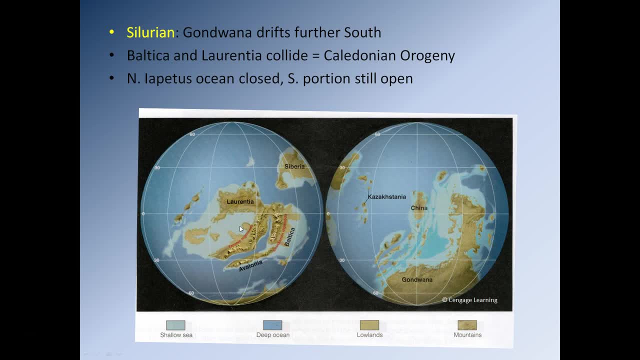 has made contact with laurentia and we have a continent continent collision going on and obviously that's producing the caledonian mountains and the taconic highlands. so that's a general overview of what's going on in terms of the position of the continents and the large 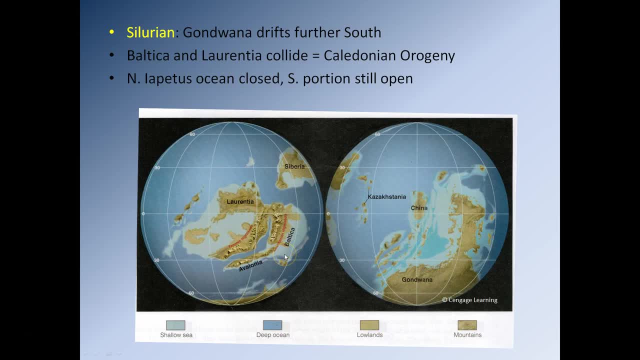 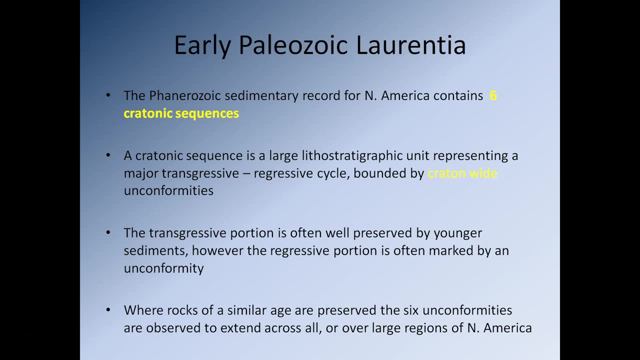 collisions. that's going on especially with reference to laurentia, and laurentia, modern-day north america. so early pay is at laurentia. so the phanerozoic sedimentary record for north america contains six cratonic sequences. so a cratonic sequence is a large lithostratigraphic. 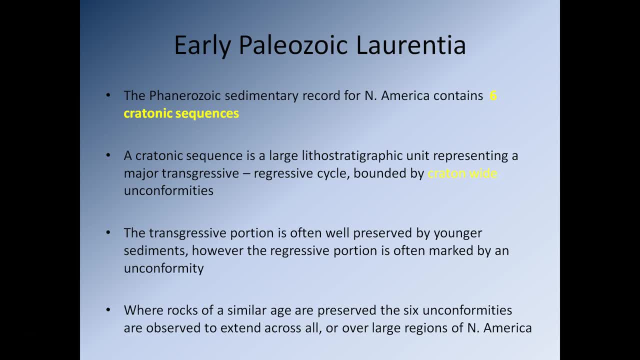 unit representing a major transgressive, regressive cycle bounded by craton-wide unconformities at the top and the bottom. so essentially it's a sequence of rocks that essentially shows a transgression going on: a very large marine transgression followed by a very large marine regression. 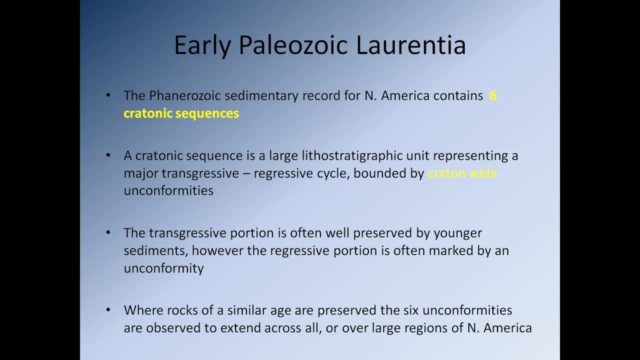 and at the top of that sequence of rocks we have an unconformity, and at the bottom of that sequence of rocks we have an unconformity, and as part of the rock record of north america, we have six of them. so the transgressive portion is often quite well preserved because, obviously, as the oceans 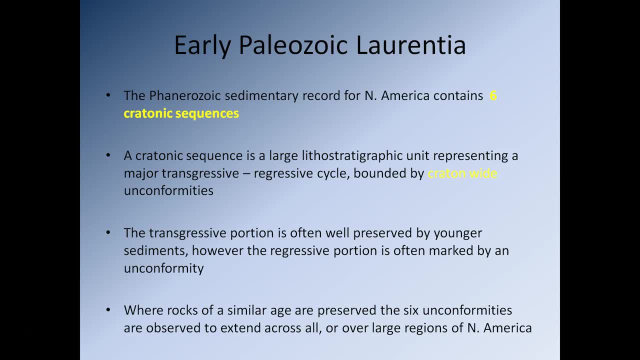 transgress onto the land. well, that's protected by new sediments being deposited on top of that transgressive sequence. now, the regressive sequence, on the other hand, is a sequence of rocks that are preserved at the bottom of the ocean and, on the other hand, that's often partially or in some places. 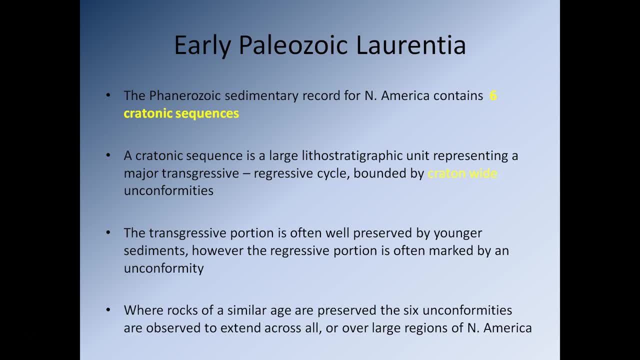 totally missing, because obviously that portion gets exposed to the atmosphere as the sea regresses, and of course, when it's exposed to the atmosphere it will undergo erosion, and so in in some cases it can be completely removed. so where rocks of similar ages are preserved, the six unconformities: 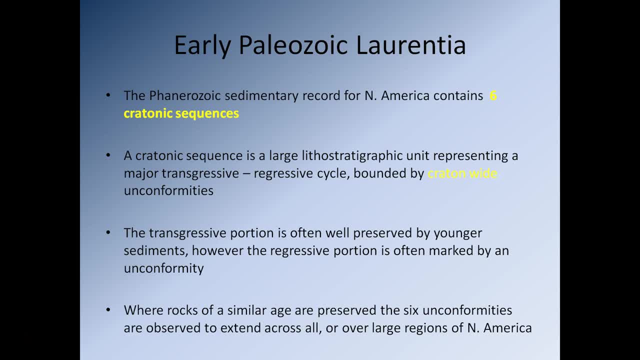 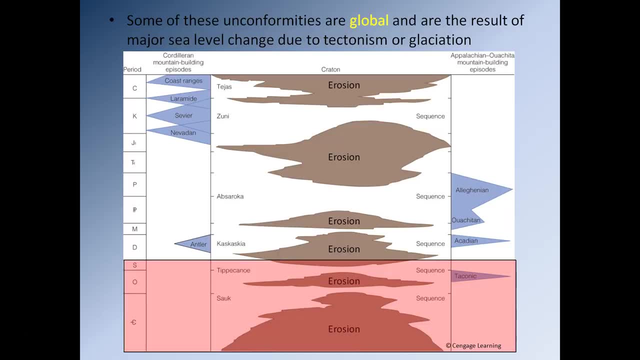 are observed to extend across or over very, very large portions of the ocean, and that's what we're looking for, what we're actually going to be sure, what we're assuming is the isotopic areas of north america, so some of these unconformities that we see are actually global. so 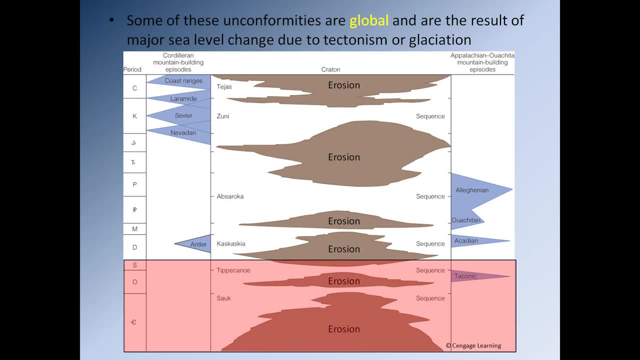 we see uh the same thing, we see these unconformities, with these large areas of uh continental crust being exposed at the same time globally. so these changes are, of course, due to sea level changes, due to tectonism or glaciation. they will obviously have a global implication. so you know if it's if. 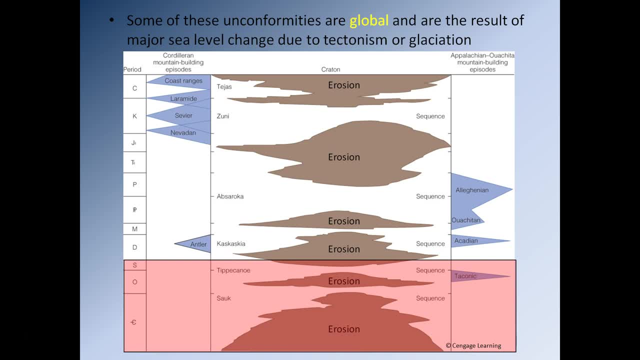 that's going to lock up water. that means sea levels are going to drop, so you're going to see a marine regression, not only in North America, but also in other continents as well. So when we look at this diagram here, what do we actually have? 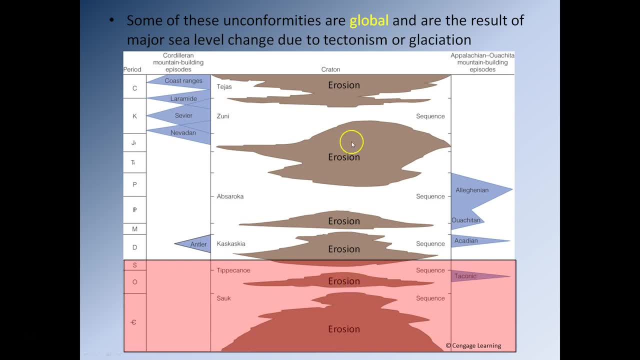 So this diagram here shows you, in brown periods of erosion and in white periods of deposition, where the deposition is taking place. So this side of the diagram represents the east coast of the United States. This side of the diagram represents the west coast of the United States. 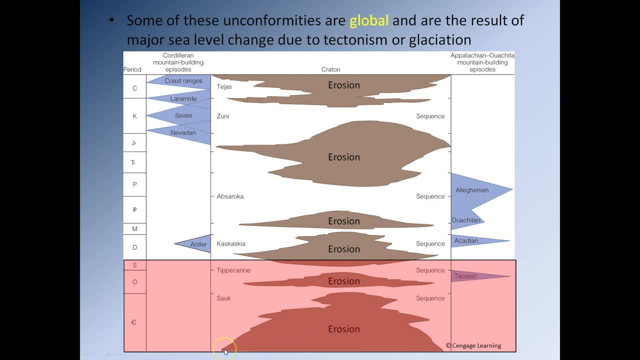 So at the start of the Cenozoic nearly all of Laurentia is exposed, so it's above sea level. So we have erosion going from the west coast all the way over to the east coast. There's nearly near complete erosion across the entire continent. 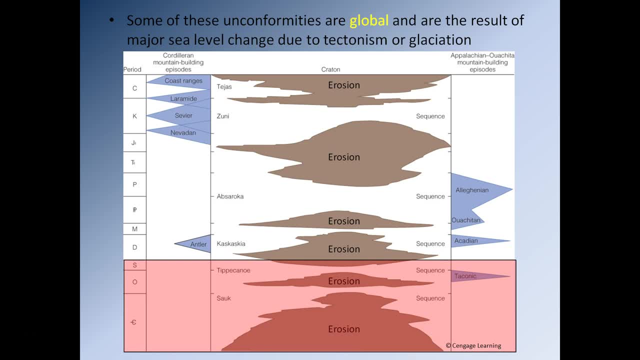 And so this means we're going to have a continent-wide unconformity forming. So what we see as we go through the Cambrian, we see the sea begins to come in to be, it begins to transgress from the west and it begins to transgress from the east. 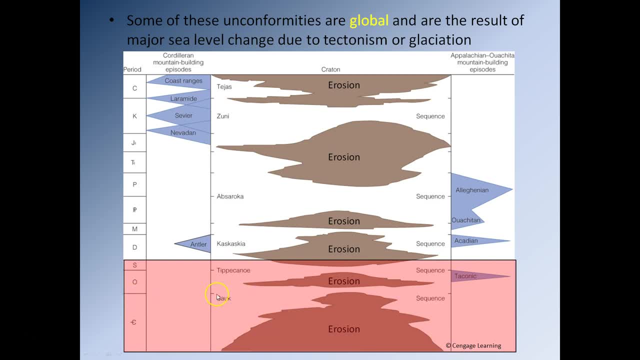 until approximately the Cambrian-Odavician boundary, when a large portion of North America is underwater. So we have essentially a body of water that covers nearly all of North America. so we have a body of water So you could sail essentially from the east coast. 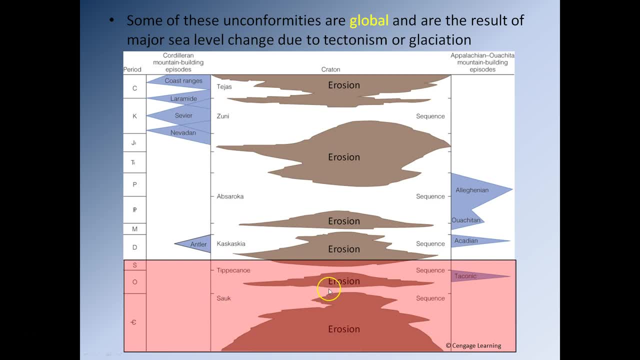 all the way over to the west coast. Now that body of water then begins to regress And we begin to see more and more of the continent becoming exposed, both on the west coast and on the home coast and the east coast. then, during the Ordovician into the early Silurian, we have another marine. 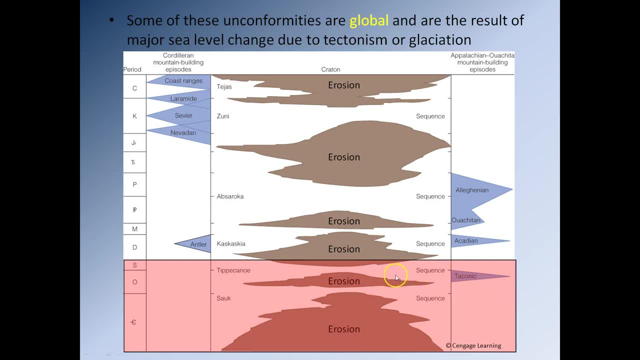 transgression. we see the sea starting to transgress in towards the centre again, once again forming a continuous ocean going from the east coast to the west coast. then, as we move into the mid-Silurian, we see a marine regression taking place. so the sea moves. 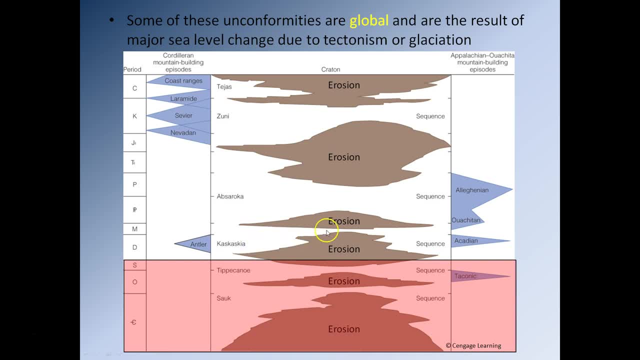 back towards the coast. then there's another marine transgression, regression, big marine transgression, marine regression, another big marine transgression, and then we have a marine regression, transgression, regression. So those are the cycles and this diagram kind of shows you what's going on and you can 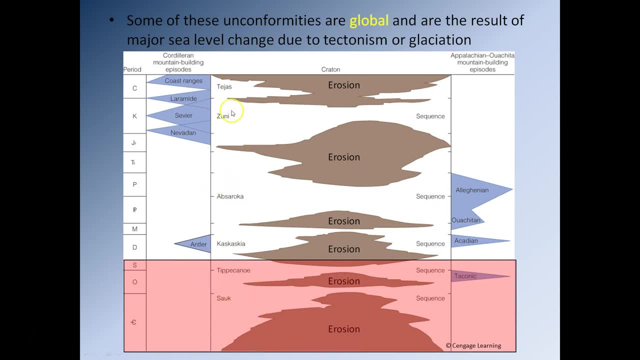 see there are six of them: Nesope, Tippecanoe, Kaskaskia, Absaroka, Zuni and Tejas- And we can also see marked in this diagram. we have the major orogenies, the major mountain building events that take place, and they're split into those that occur on the east coast. 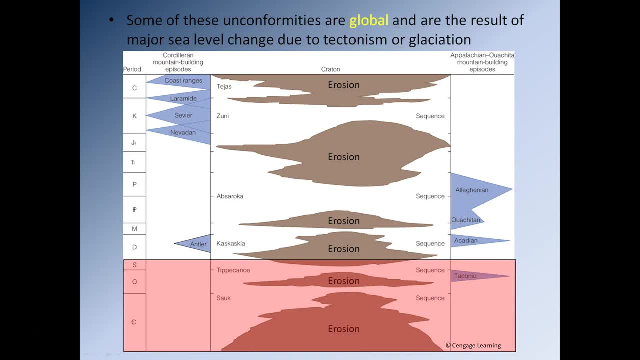 and southern portions Of Laurentia and those that occur along what is now the modern-day west coast of Laurentia, And so on the east coast we have the Taconic, the Acadian, the Achetan and the Elagahenian. 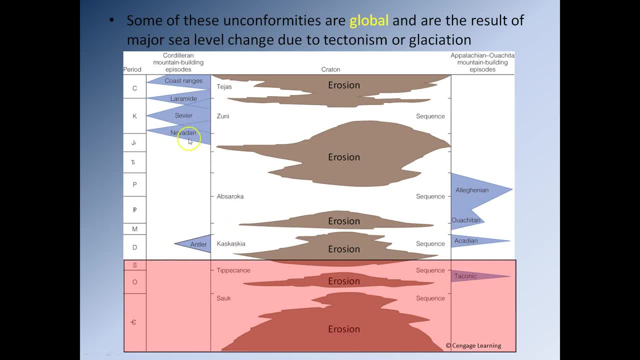 And on the west coast we have the Antler, Navardian, Sevier, Laramide, and then at the top here we have the coastal ranges, but we're not really going to discuss those too much. Okay, so the identification of grittonic sequences. 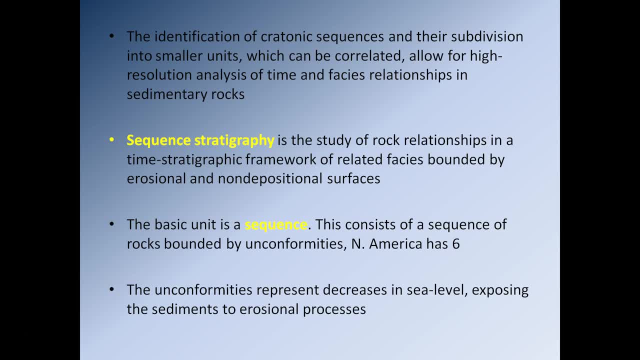 We'll be left until we've had a break. So, all right, this is a good moment. Let's pause the presentation, get up, have a walk around, go and get a glass of water and please come back in a few minutes. 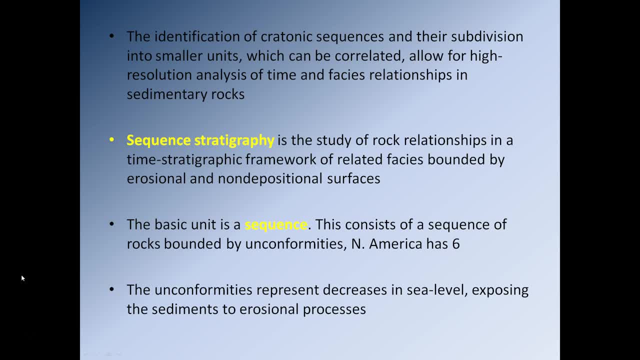 So okay, so these grittonic sequences, as I said, are bounded by large unconformities at the. Okay, that's me not turning off my iPad. There we go. Serves me, right. I apologise for that. Anyway, where were we? 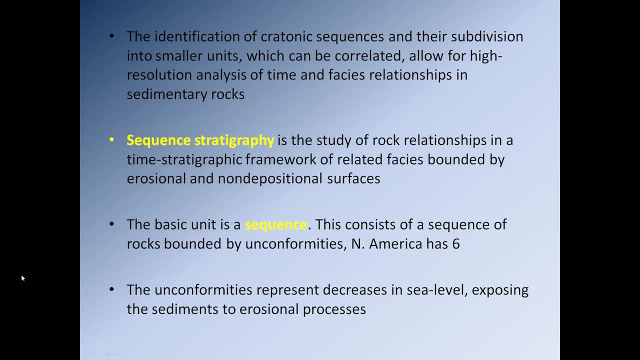 So the identification of grittonic sequences is based on your ability to spot the larger conformities that occur at the upper and lower margins of the sequence. So these conformities allow us to correlate essentially across the continent. So if we go back to the previous diagram here you can see, based on the unconformity, that's 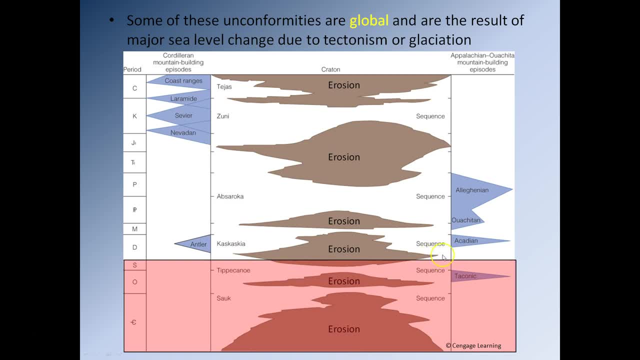 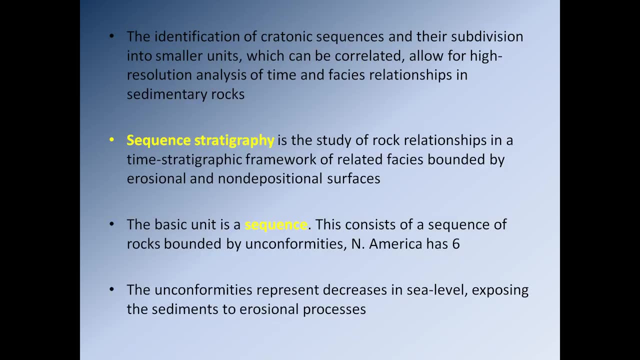 forming here during the period of erosion. we can correlate rocks on the east coast to rocks on the west coast relatively efficiently, So this allows for very, very high resolution analysis in terms of rocks and, of course, in geology, rocks represent time. 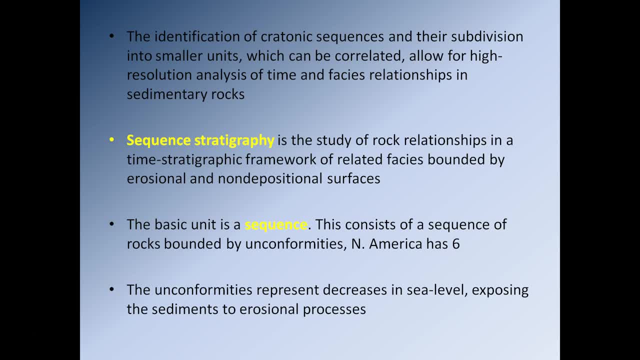 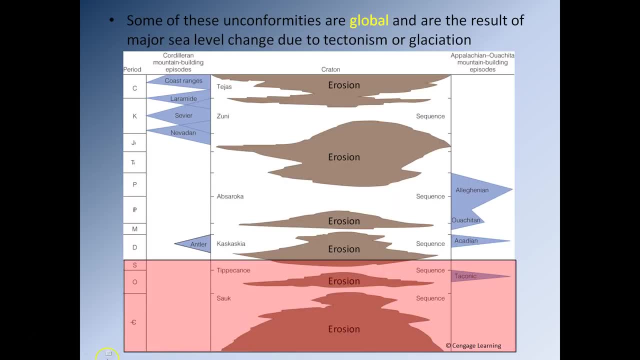 And it also allows us to do Fasci's analysis of the relationships by using the sedimentary rocks. So we can see, essentially, as we come across the continent we can, We'll see changes in Fasci's and we can date these changes in Fasci's based on what's going on in terms. 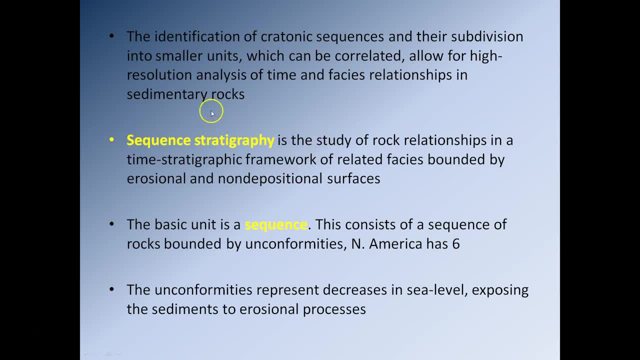 of the stratigraphic sequence. So we use these packages of rocks to do what we refer to as sequence stratigraphy, And it's the study of rock relationships in a time stratigraphic framework of related Fasci's bounded by erosional and non-depositional surfaces. 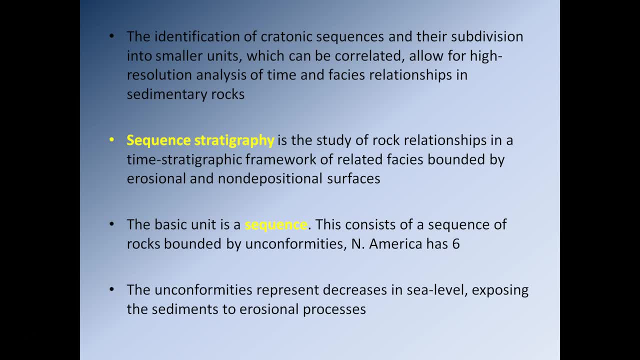 So, essentially within these, within the rock record, we have these six sequences, the ones we spoke about: The Soke, Tippecanoe, Kaskaskia, Absaroka, Zuni and Tejas, And then we have these six sequences, the ones we spoke about. 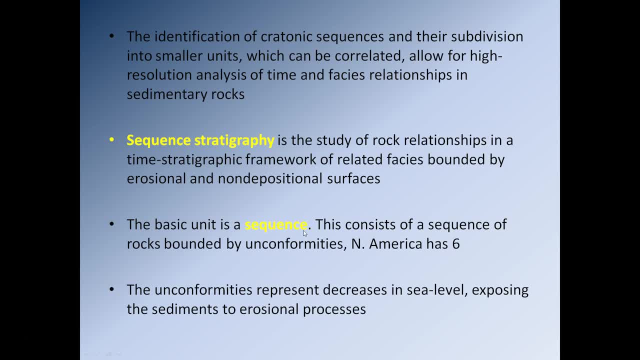 The Soke, Tippecanoe, Kaskaskia, Absaroka, Zuni and Tejas, And then we have these six sequences, the ones we spoke about, And within them there are obviously going to be smaller cycles, which will also have 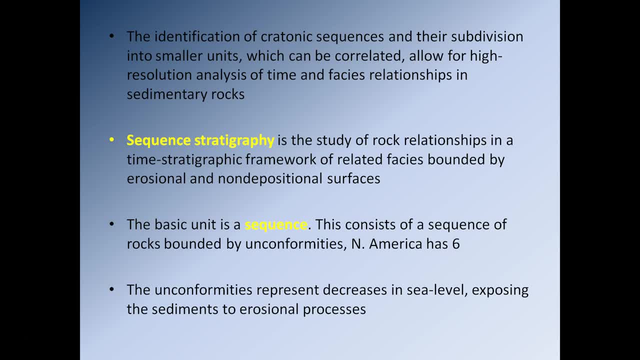 erosional boundaries at the top and the bottom and we'll use those as well And essentially we use these units, these formations, essentially to allow us to do sequence stratigraphy that in some cases can allow us to tie up rocks on the east coast to rocks. 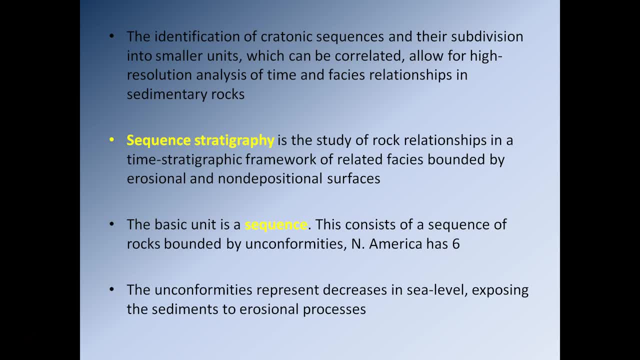 on the west coast And of course we need to always bear in mind unconformities represent periods of When we have decreases in sea level leading to the exposure of continental rocks And the process of erosion, which obviously creates the unconformity because erosion causes. 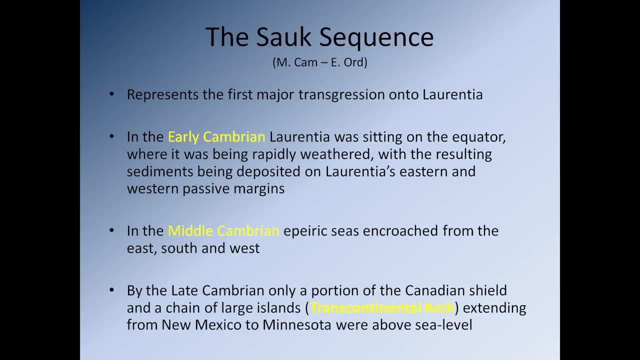 us to lose rock and therefore we lose time. All right, so let's start with the Soke sequence. So that makes its appearance in the middle Cambrian and it goes through to the early Ordovician, So it represents the first major transgression onto Laurentia. 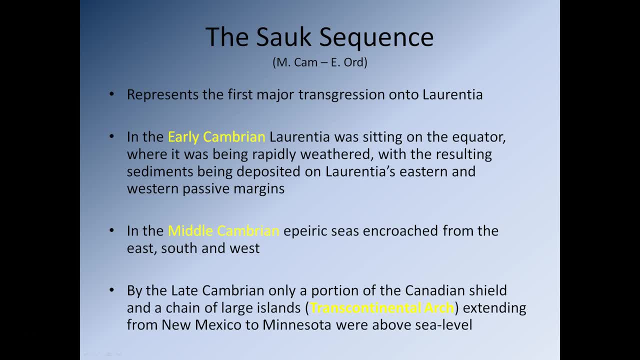 So in the early Cambrian, Laurentia was sitting approximately on the equator, where it was being rapidly weathered, With the resulting sediment being deposited along the eastern and western passive margins. So you had huge rivers cutting across the continent, dumping sediment on the east and 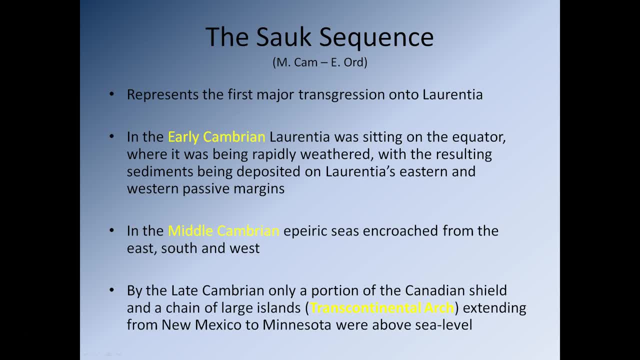 western coasts. So in the middle Cambrian we see the encroachment of an Epiric Sea from the east, south and west. We have a very large marine transgression going on. So by the late Cambrian only a portion of the Canadian Shield and a chain of large islands. 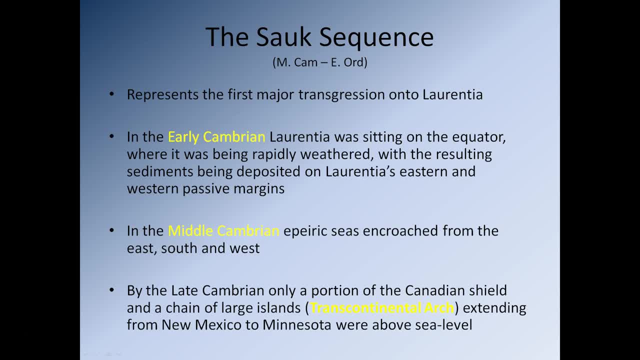 called the Translucent. So this is the Chaldean Sea, which is the largest marine transgression in the world. So you can see that the sea level is quite high. when it comes to the Transcontinental Arch, which extended from New Mexico to Minnesota, where above sea level 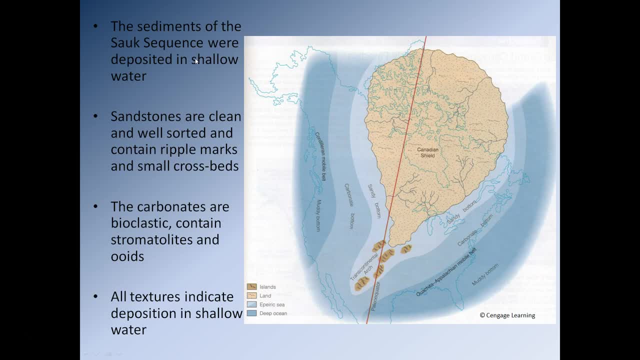 So the sediments of the Soke sequence were deposited in shallow water And we see the sandstones are clean and well sorted, contain ripple marks and small cross beds, So that would suggest that they're being deposited into a shallow sea where the sandy sediment 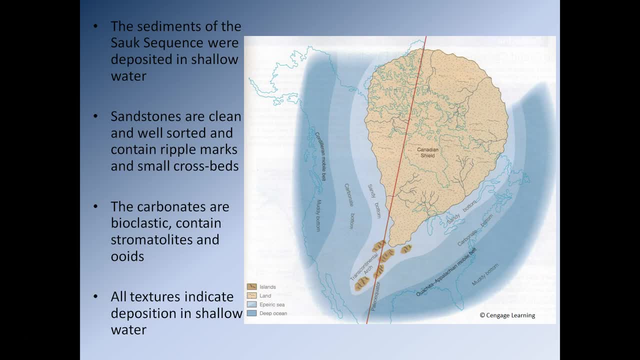 is being churned up by typically wave action. We also see there are lots of carbonates forming, We've seen a lot of rock. They have a lot of sediment and they contain stromatolites and ooids- Once again, a very, very strong indicator that you're dealing with a very shallow water environment. 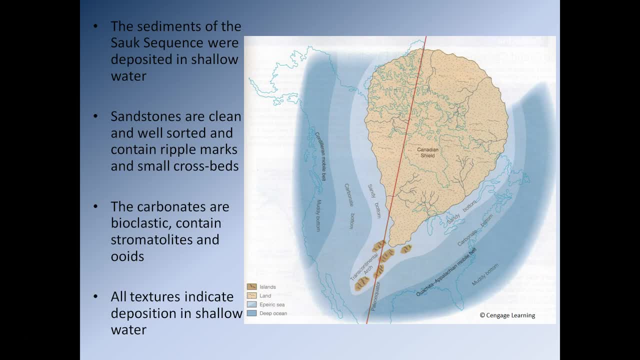 because stromatolites need shallow water to exist. you know, the water depth can't be too deep. Same with ooids: In order to form ooids, you need to have the water being constantly churned up by the action of waves. 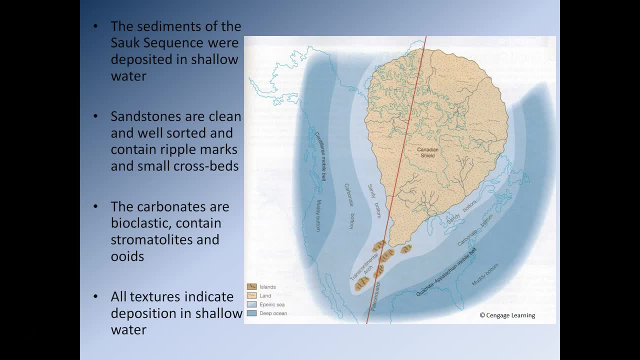 so you can't have ooids in deep water. So this diagram here kind of gives you an idea of what we're basically looking at. So you can kind of just about see the outline of North America here in blue, and this is obviously Laurentia here, and you can see the portion along the margin of Laurentia. 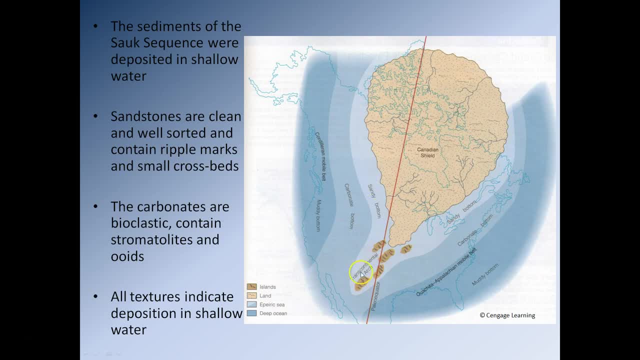 well, that's referred to as the sandy bottom, and that's because this area here is a shallow Epiric Sea where we have lots and lots of detrital sediment being deposited by these very, very large rivers, So we have lots of sandy sediment in this area, so that's where we're getting these sandstones. 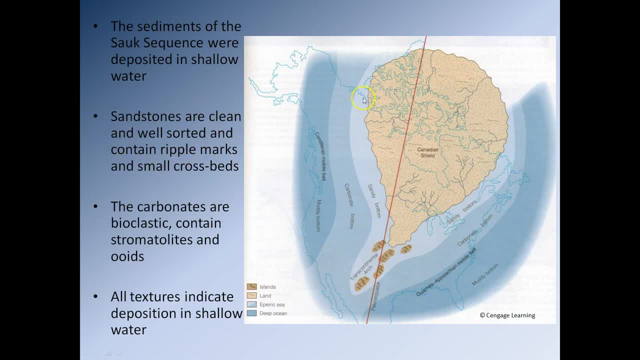 They're clean, well-sorted and they contain lots of ripple marks and small crossbeds. Now then, as we head out into slightly deeper water, the water becomes clearer. it's still shallow, it's warm because we're at the equator, but it has very little detrital sediment suspended in it. 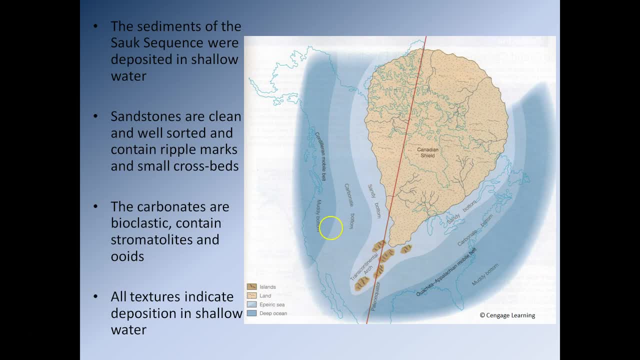 so we have nice clear water and so this is where we get carbonates forming, so we get large-scale limestone formation in this region coming all the way around here, And then as we go out, we head out into deeper water and then we head out into the muddy bottom. 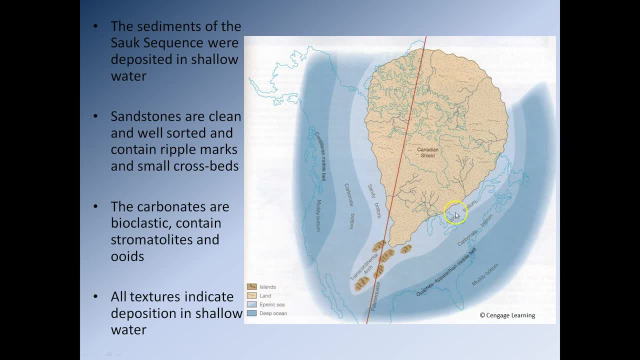 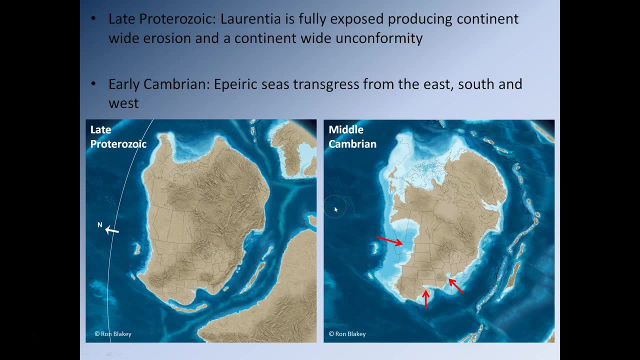 that's where we're getting these deeper marine sediments forming. So the deeper marine sediments obviously tend to be quite fine-grained and dominated by silt and clay, So by the late Proterozoic. this diagram here kind of shows you. so this is the late Proterozoic here. 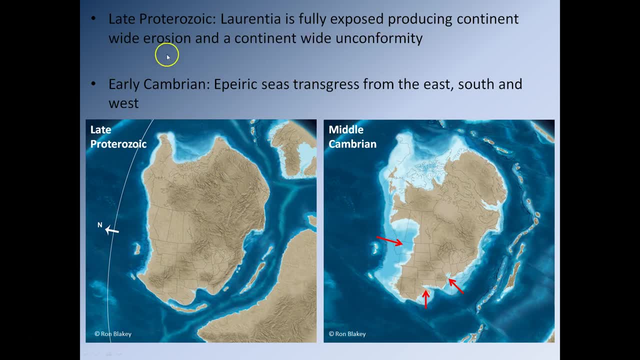 we have Laurentia fully exposed, producing a continental-wide erosion which leads to a continent-wide unconformity. So we have essentially what would be considered the modern-day west coast of Laurentia, and here's the east coast and you can see it's exposed from all the way, from the west coast. 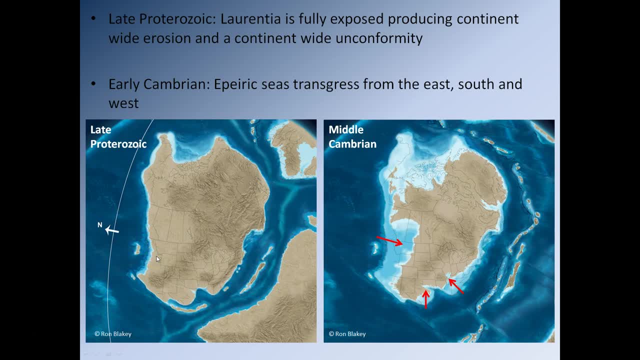 over to the east coast. You could have walked from one side to the other relatively easily. Now in the early Cambrian, as I said, we begin to see the seas begin to make their move. so the seas begin to transgress from the north, the west, the south and the east. 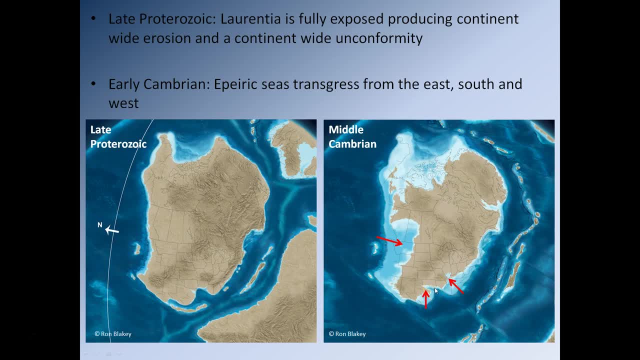 I should point out: when I'm using north, west, south and east, I'm using them in the modern context. You'll notice, here there's the north arrow there. so you'll notice that what is now the modern-day west coast. 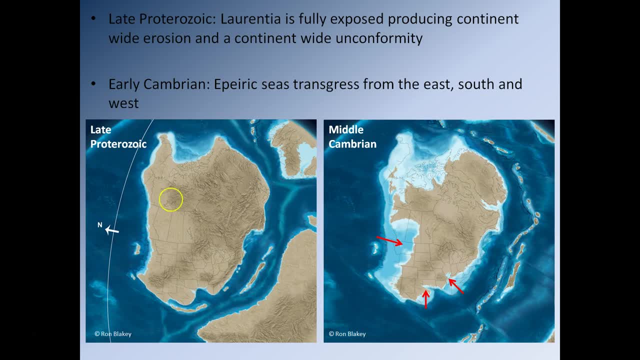 was in fact facing in a northwards direction during the Proterozoic and also in the Cambrian as well. so please bear that in mind. So anyway, so in the middle Cambrian we have, the sea begins to transgress from the west, the south, the east and the north. 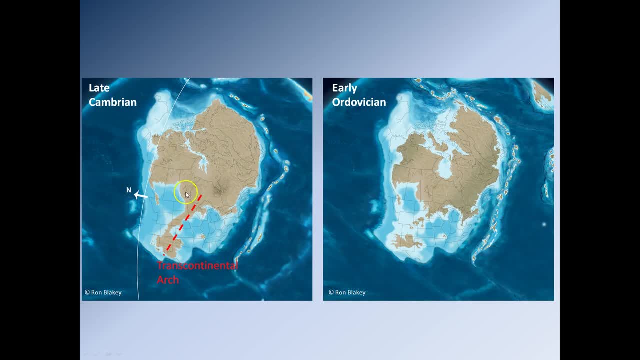 and so as we move into the late Cambrian we can see that we have a very extensive body of water. so we have our transcontinental arch here we have nearly the centre and eastern portions of the states are covered are underwater. the western states are underwater. a significant proportion of Canada is also underwater. 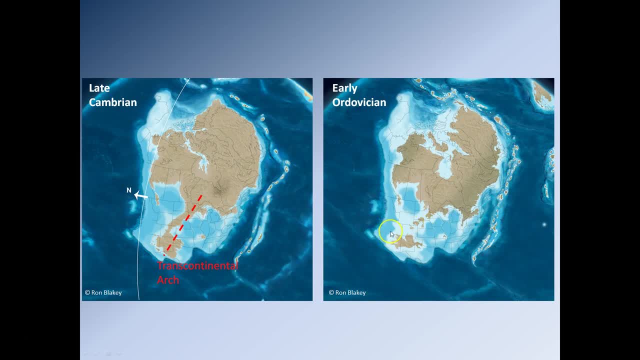 and by the early Ordovician you can see, we have a body of water, an empiric sea, a shallow empiric sea that extends all the way from what is the west coast over here, all the way over to what is the east coast over here. 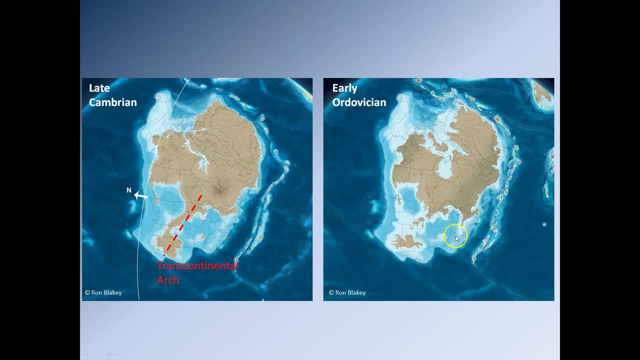 so we have a continuous body of water going from one side of the United States to the other, And what we have is a region marked out here by the slightly more white colour. that's going to be a region that's dominated mostly by sandy sediments. 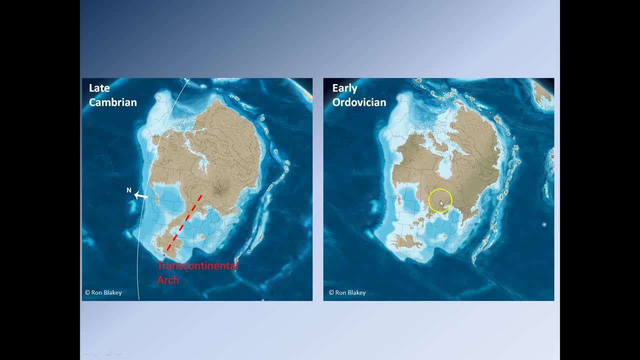 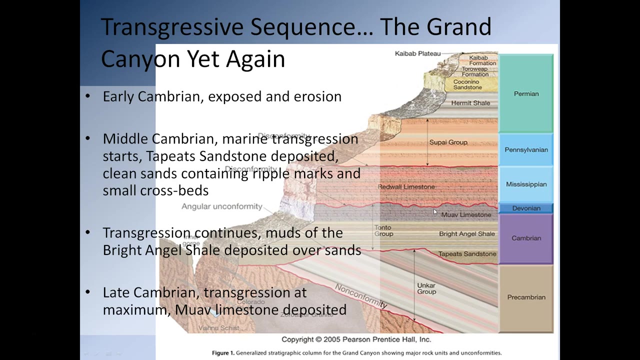 so that's material being eroded off the exposed crust here, being transported by rivers, deposited along the coast here, this slightly darker blue area here, this is the area where we're going to get large-scale carbonate deposition taking place. So what about this transgressive sequence? what kind of evidence do we have that it took place? 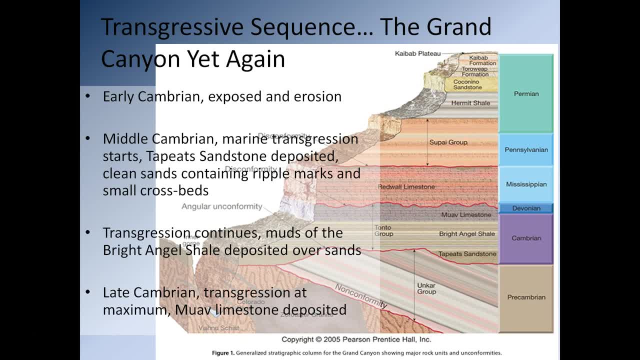 Well, once again we're actually going back to the Grand Canyon. I know it's come up a couple of times, but here we are again. So at the Grand Canyon we see we have early Cambrian rocks that are exposed and eroded. 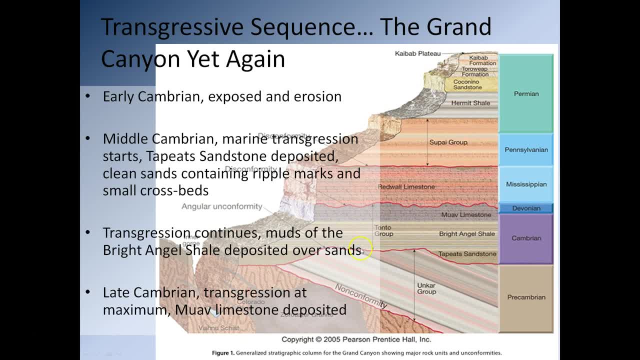 so here we go. so here are the Cambrian rocks. down here they form the Tonto Group. So by the middle of Cambrian we have a marine transgression. we see the deposition of the Tapit Sandstone. okay, the Tapit Sandstone is a clean sandstone containing ripple marks and small crossbeds. 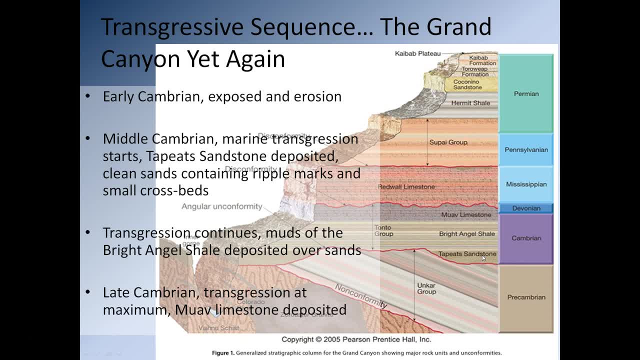 that's essentially a shallow marine coastal sandstone. We then see over the top of the Tapit Sandstone we have the Bright Angel Shale being deposited, so the water depth is increasing. and then over the top of the Bright Angel Shale we have the Limestone being deposited, and that represents we're in shallow, clear water. 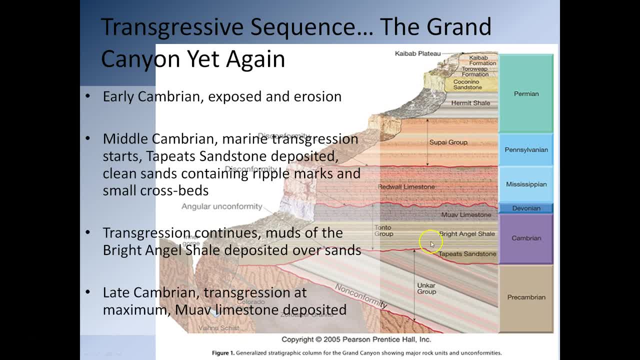 So as we head from the Cambrian, as we head through the Cambrian, we go sandstone, mudstone, limestone, So essentially we are heading into. we've got a marine transgressive sequence. the water depth is steadily getting deeper as the ocean gets. well, there's more and more as the ocean transgresses. 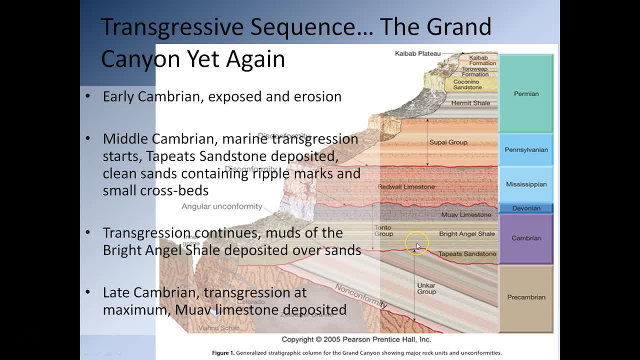 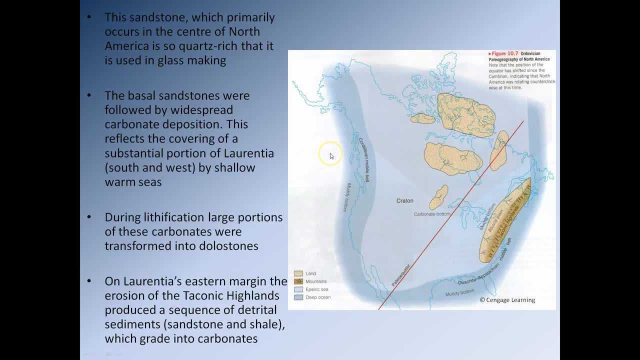 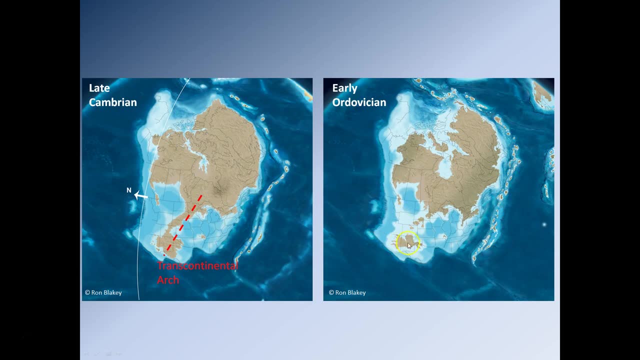 further and further across North America, or should I say Laurentia. So there the Tonto Group is part of the soak sequence. so, of course, if we go back to the, if we go back to the diagram here, obviously we are going to be down in this area, here. that's where the Tonto Group is going to be forming. 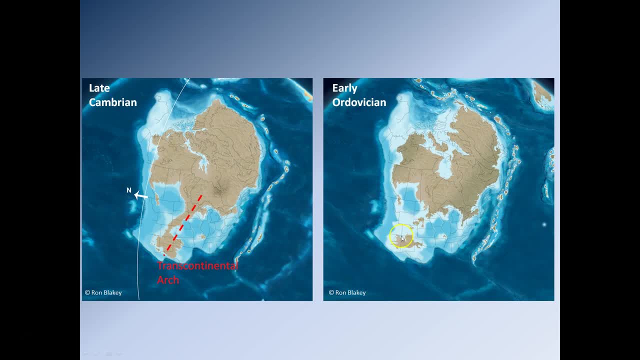 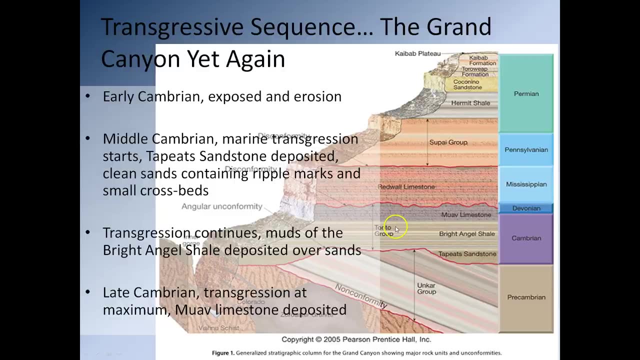 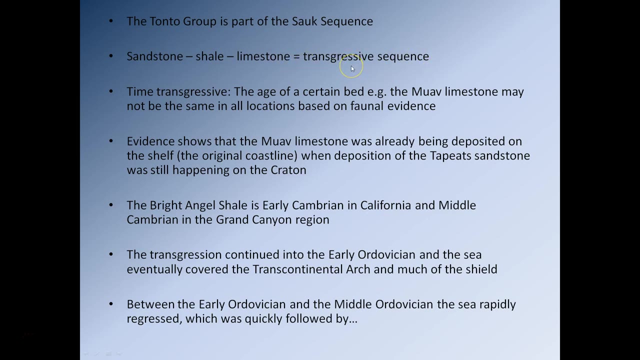 So, as the water depth gets higher and higher and higher, this area is initially dominated by sandy sediments, then it gets covered over by muddy sediments, then eventually it gets covered over by carbonate sediments. So obviously, as I said, it has this sandstone, shell, limestone, transgressive sequence that tells the water depth is increasing. 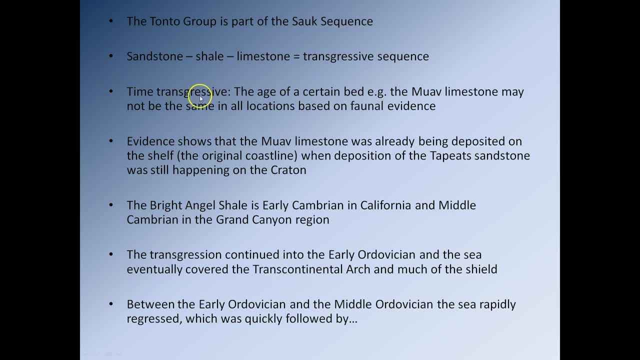 And the sequence itself is time transgressive. So the ages of certain beds, eg the Mojave limestone, may not be the same in all locations, based on the faunal evidence. So evidence shows that the Mojave limestone was already being deposited on the shelf. that's the original coastline. 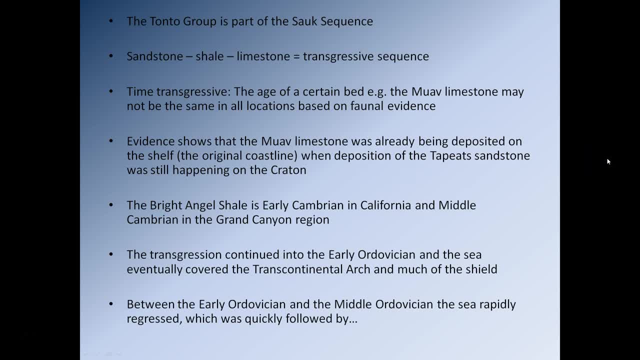 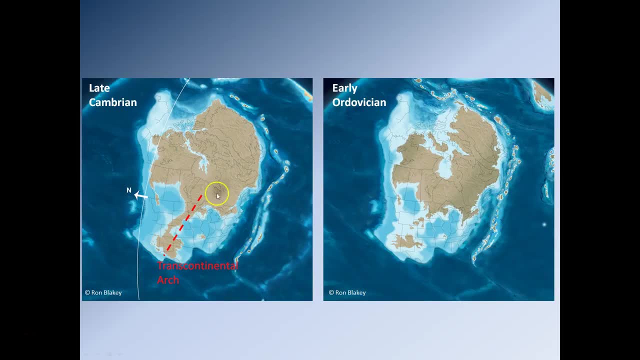 when the deposition of the Tapit sandstone was still happening on the Kraton. So what this means is, if we think about this model here, we had the Mojave limestone being deposited here, but as we come this way, we have the Tapit sandstone being deposited over here. 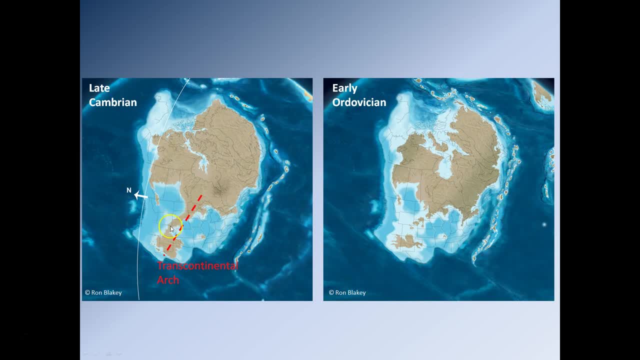 in the coastal region. Now, what's going to happen over time is this coastal region is then going to get covered over by deeper water that's going to give us the Bright Angel Shale, and then eventually, even deeper water that's going to give us the deposition of the Mojave limestone. 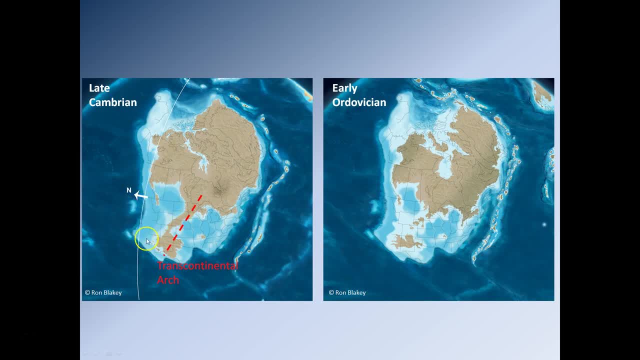 So the most important thing to realise is that at the same time, we have the limestone deposition going on over here and we have the Tapit sandstone deposition going on over here, and so we have a time transgressive sequence. essentially, We have essentially rocks that are the same age here and here, but those rocks are different. 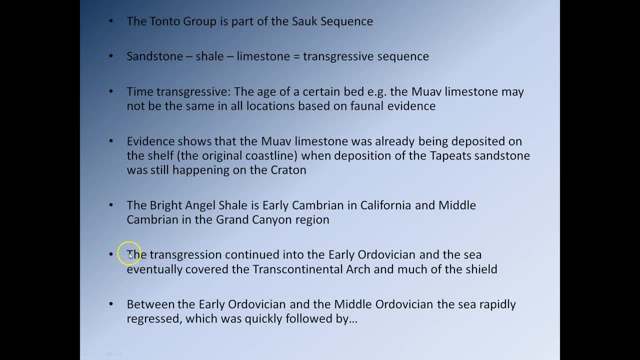 And so what we're going to see is that the Bright Angel Shale, essentially in the early Cambrian, is in California and by the middle Cambrian it's in the Grand Canyon region. So, essentially, as the sea levels begin to rise, we see these fashies begin to shift inland. 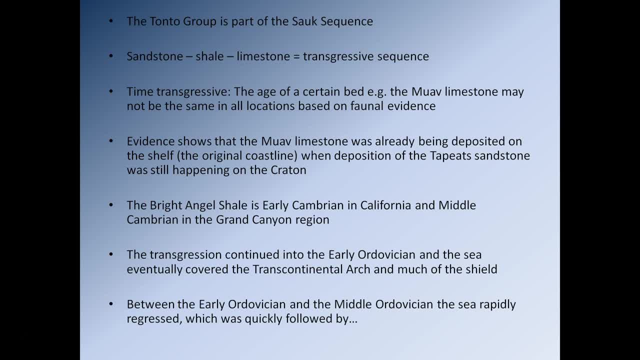 So if you follow the same layer of rock along, so let's say you start off on the west coast in California- what is now modern day California- and you head towards the centre of the United States, and you follow the same layer of rock as you head towards the centre of the United States- 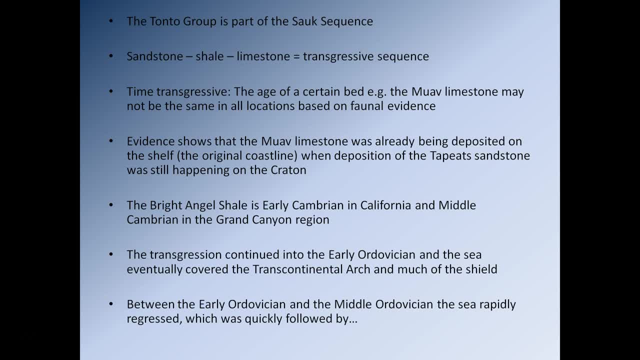 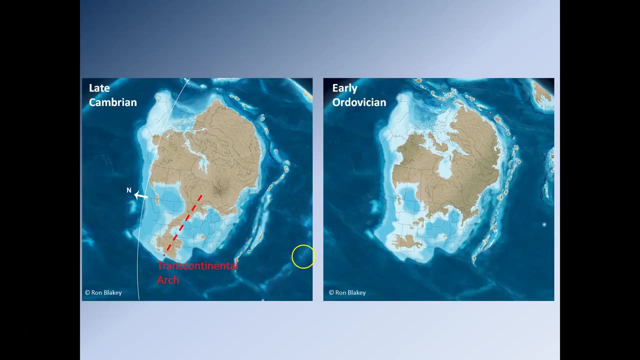 that same layer of rock you're following is going to be getting younger, So the transgression continued into the early Ordovician and the sea eventually covered the transcontinental arch and much of the shield. So by the early Ordovician you can see that a significant portion of North America is underwater. 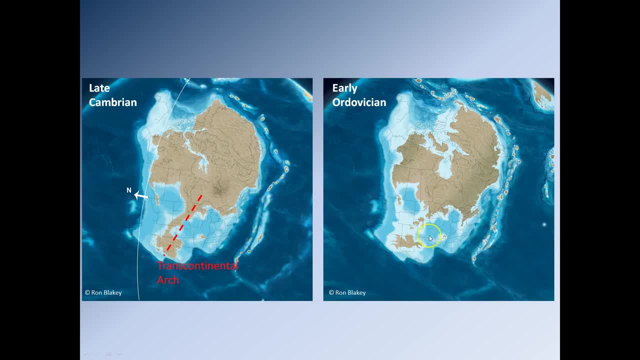 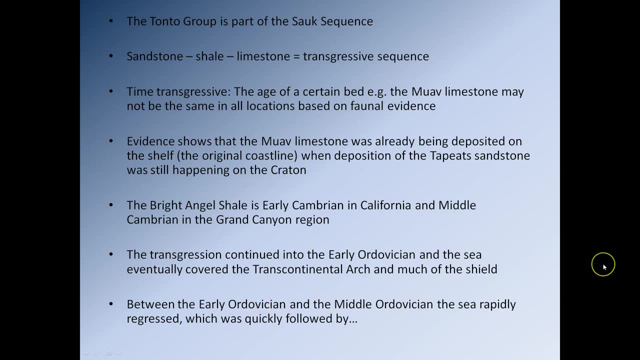 and especially the United States. The United States is nearly completely underwater at this point. So between the early Ordovician and the middle Ordovician we see a marine regression taking place. There's a very rapid retreat, which then leaves Laurentia exposed. 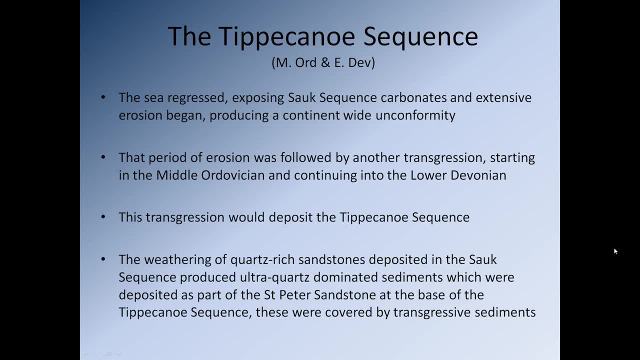 Now, this exposure doesn't last very long. Now remember, though, once Laurentia is exposed, obviously erosion takes place, and erosion means lost rock, which means lost time. So, essentially, we have an unconformity forming Now. what we begin to see then is we see the sea regress in the early Ordovician. 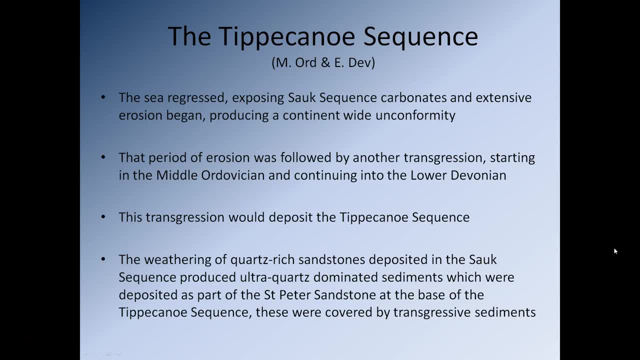 and then we see a very, very quick turnaround and we then see the start of the Tippecanoe sequence. So the period of erosion in the early Ordovician was followed by another marine transgression, and that started in the middle Ordovician. 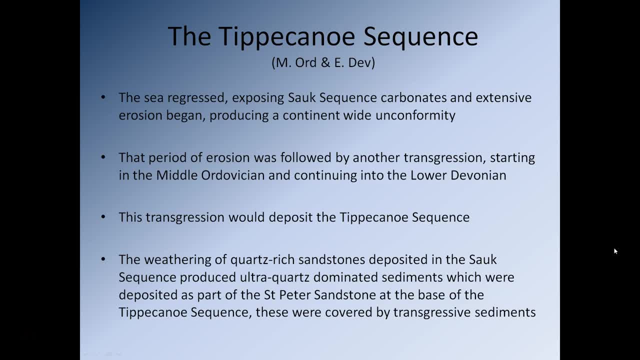 and it continued all the way through to the lower Ordovician- Lower Ordovician, sorry, I do apologize. Lower Devonian. So the weathering of the quartz-rich sandstones deposited in the Soak sequence produced an ultra-quartz-dominated sandstone. 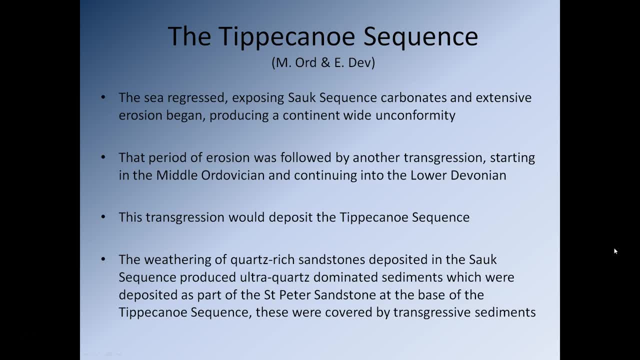 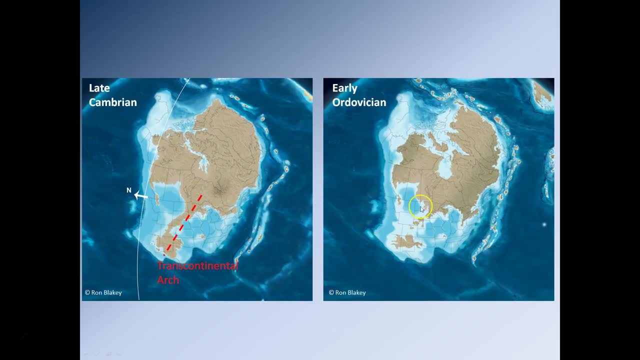 sandstone-dominated sandstone Sandstones which were deposited as part of what's referred to as the St Peter sandstone at the base of the Tippecanoe sequence. So the exposure of the sediments deposited essentially in these regions, especially these very, very clean sandstones deposited in these coastal regions. 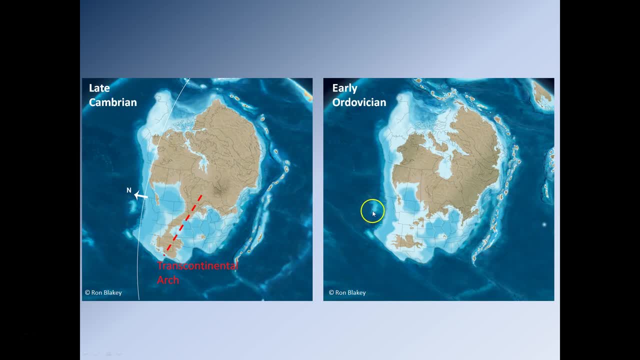 well, when they become exposed to the atmosphere, when the sea regresses, they are eroded and they are further transported, which means that they lose even more of the very, very small portion of feldspar, for instance, is in them, and by the time we make, 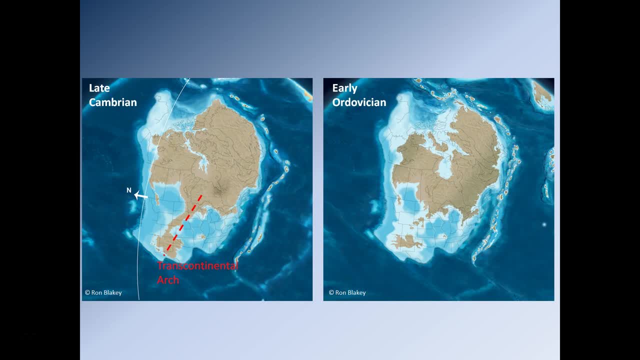 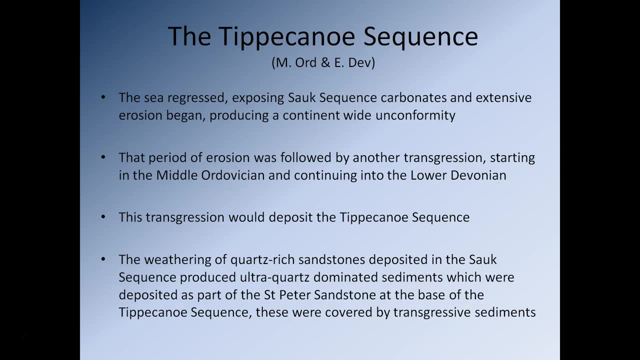 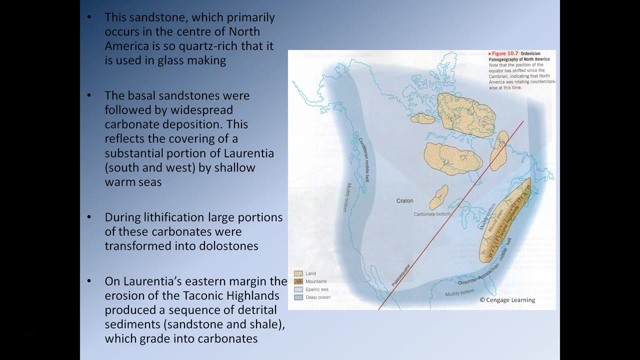 into the Tippecanoe sequence. these sandstones that are right at the base of the Tippecanoe sequence are ultra-pure sandstones, And so they're very, very important when it comes to glassmaking. So the basal sandstones were followed by widespread carbonate deposition. 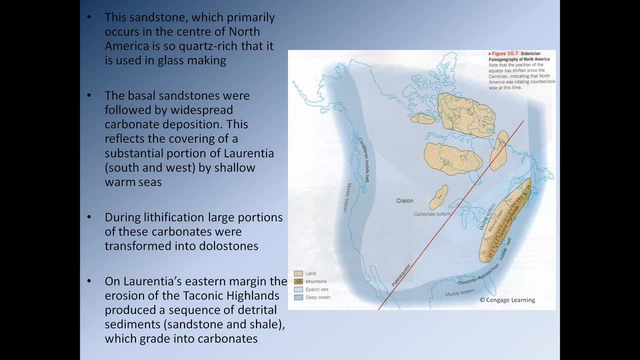 and this reflects the covering of a substantial portion of Laurentia by shallow warm seas. So right, what's happening in the case of the Soak sequence? Well, the Tippecanoe sequence differs slightly from the Soak, Why? 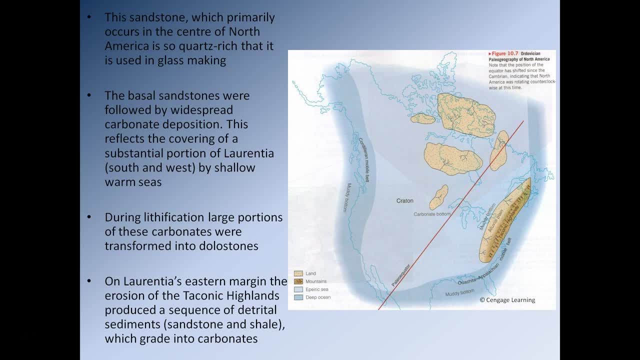 Well, it differs because an even larger portion of Laurentia finds itself underwater. Now, if your continental crust is underwater, it cannot be eroded. If it's not being eroded, you're not producing detrital sediment. If you're not producing detrital sediment, then when that sediment gets deposited into the oceans, 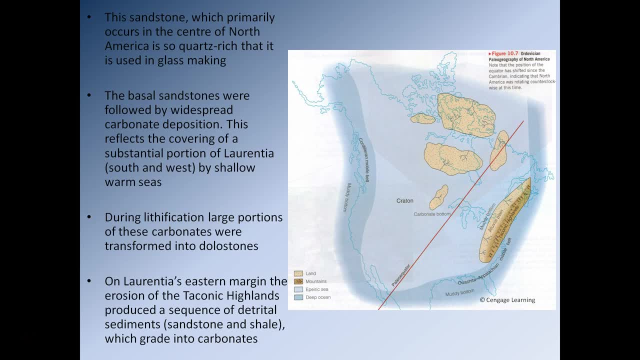 only a relatively small portion of it is being eroded. So if you're not producing detrital sediment, then when that sediment gets deposited into the oceans, well, only a very small amount is being deposited into the oceans, and so it doesn't really affect the water quality that much. 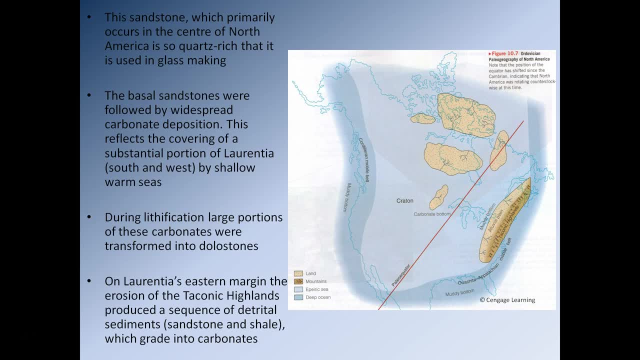 And so what that means is, is you, during the Tippecanoe sequence, you have a shallow, warm, empiric sea which is essentially sitting right on the equator, and it has very little detrital sediment being deposited into it. 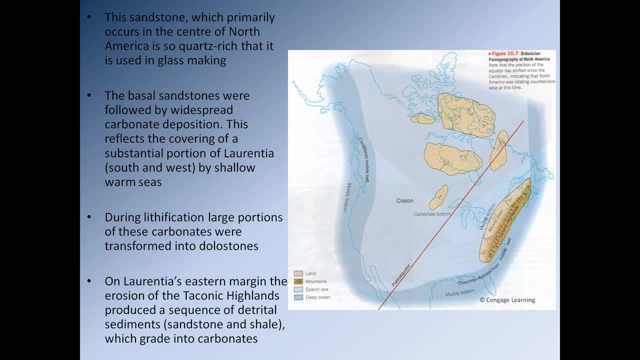 which means the water quality is spectacular- So think of the clear blue seas of the Caribbean here- And that means that what you're going to get is you are going to get massive, absolutely massive carbonate deposition. So essentially, the entirety of North America becomes one massive carbonate shelf. 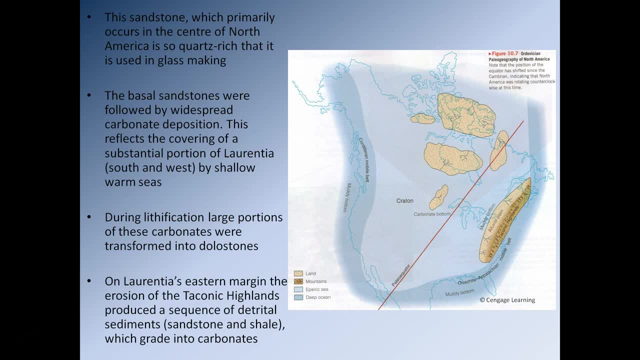 with huge, huge quantities of carbonate being formed and deposited. So during the lithification of these carbonates, a lot of them got transformed into dollostones. So, if you remember, during the lithification process, if a magnesium-bearing fluid moves through the carbonate that's being lithified. 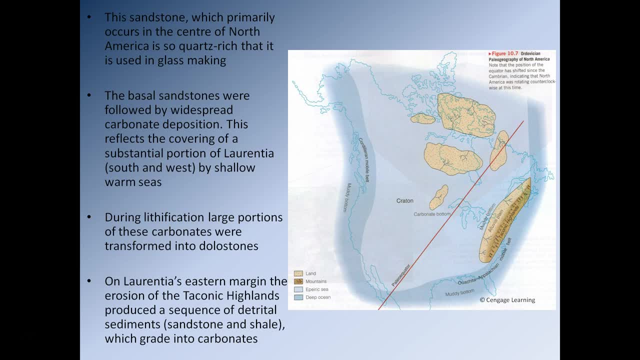 the calcite will alter to give dolomite, And we also, at this point, have an important event taking place Along the eastern seaboard. we have the formation of the Taconic Highlands, And this is the result of the destruction of the Iapetus Ocean. 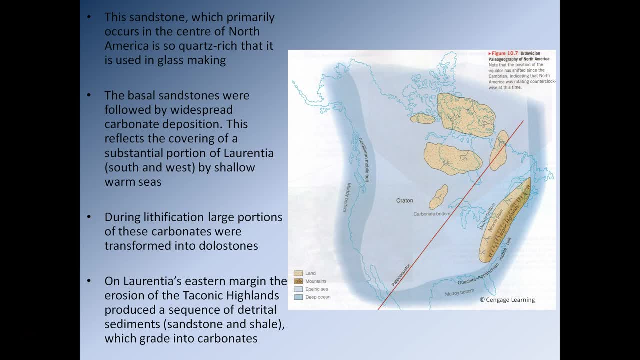 and the movement of Baltica and Avalonia towards the east coast, what is now the modern-day east coast of North America. Now, the sequence associated with the Taconic Highlands is dominated by sandstones and shales, which eventually grade into carbonates. 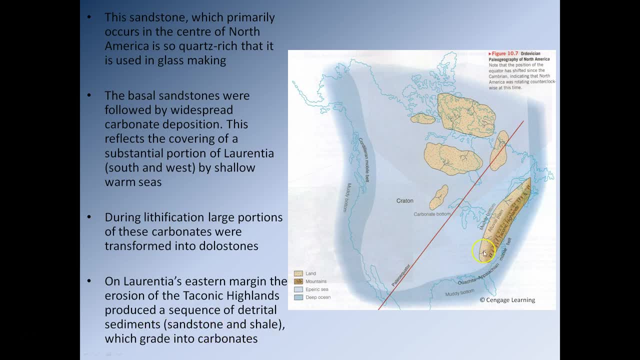 That's because, obviously, you have an area of high ground forming. That area of high ground is exposed to the atmosphere, and so it can be eroded, producing detrital sediment, And so the area around the Taconic Highlands is going to be dominated by clastic sediment. 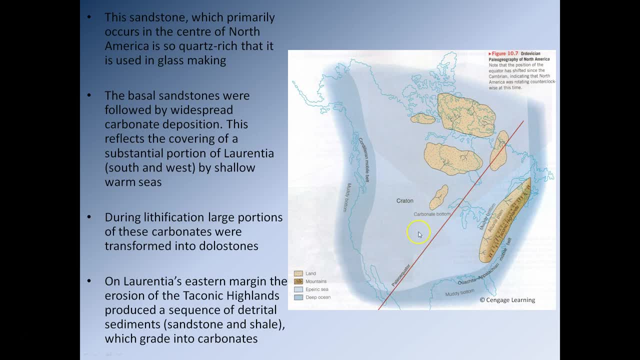 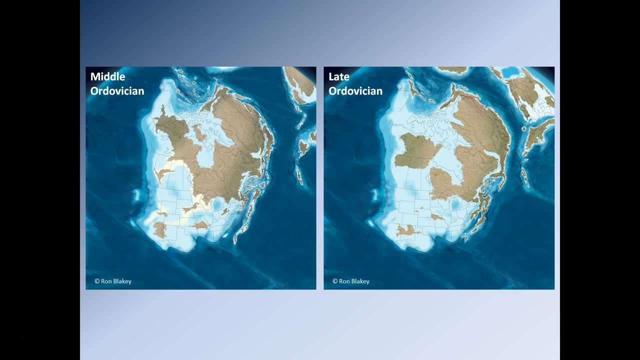 but as soon as you move away from that area you're going to be heading back onto the carbonate shelf. So okay, so this is our situation. So by the middle Ordovician you can quite clearly see that we're pretty much back to the kind of situation we had during the soak. 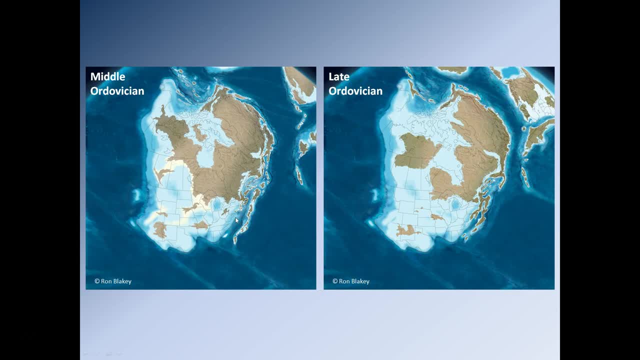 So you'll notice that a very, very significant portion of North America is underwater: nearly the entirety of the United States and a very, very large portion of Canada. By the time we're into the late Ordovician, we can see that nearly all of the United States is underwater. 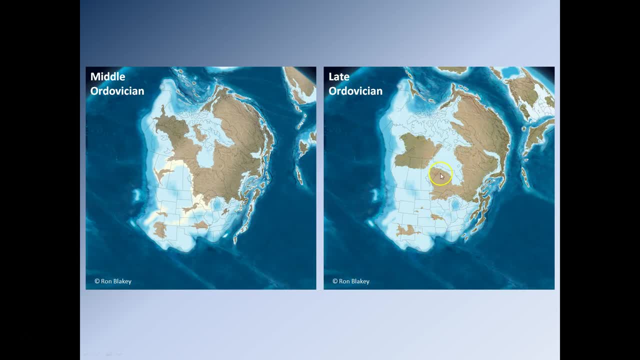 and even more of Canada is now underwater. This means that there is very little detrital sediment actually being produced. So this water here, this water quality in this region here, is going to be spectacular Okay, and that's going to be great for carbonate formation. 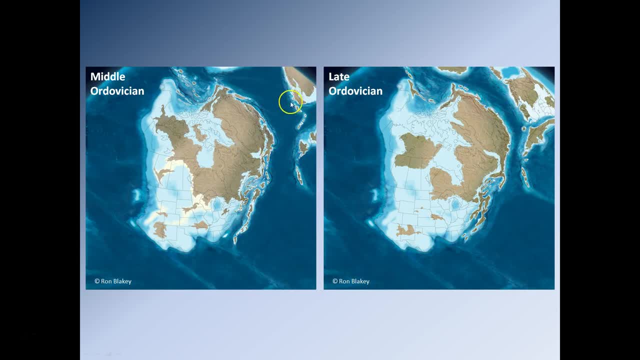 You'll also notice. if you look towards the top right of the image, you will see the impending collision. Here comes Baltica and here comes Avalonia. down here The collision is on the way. You can see as we move into later Ordovician. 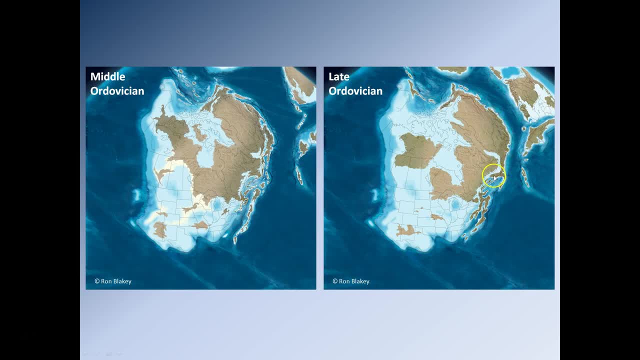 they're getting steadily closer and you can see the crust here is beginning to deform in response to the impending deformation. You can see the formation of what would be the Caledonian Highlands up here And Taconic Highlands starting to form down here. 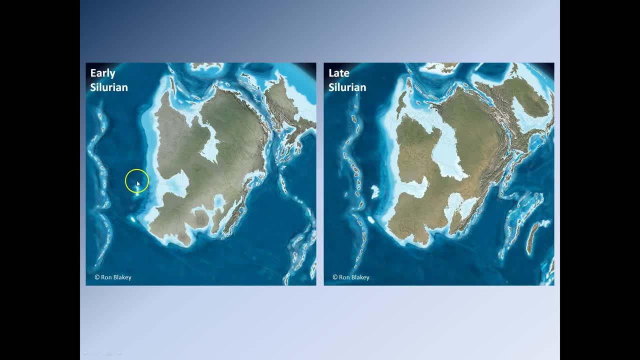 By the early Silurian. we have a regression going on, So a lot of the water retreats off the continent. You'll notice, by this point Baltica is now nearly in contact with North America, So here we have the Caledonian Highlands, here. 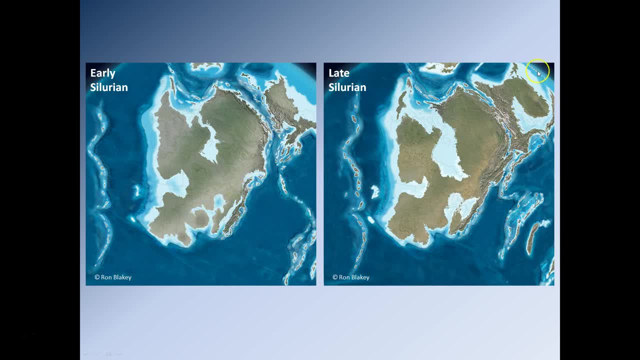 the Taconic Highlands down here And by the late Silurian. we can see that Baltica has crashed completely into Laurentia, producing the Caledonian Highlands here And obviously we have the Taconic Highlands forming down here And by the early Devonian. 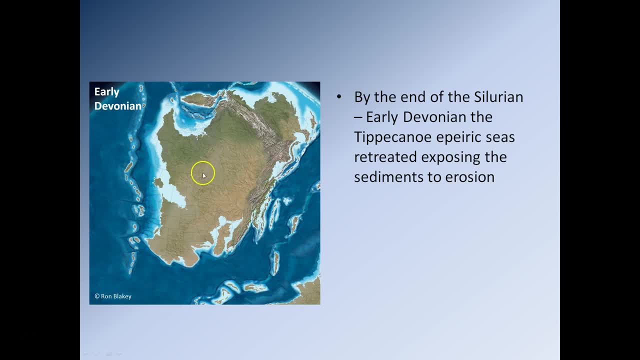 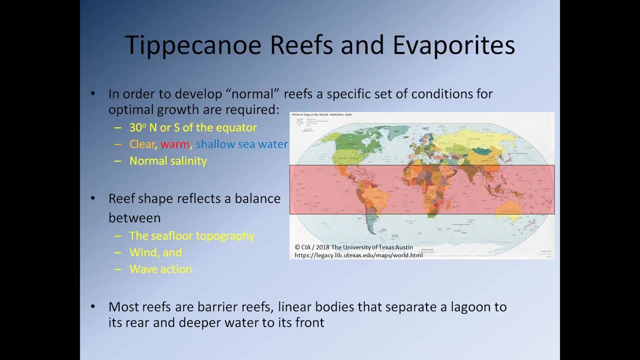 we have a full marine regression going on And once again, North America, or should I say Laurentia, is now exposed and massive erosion starts to take place, forming a continent-wide unconformity. So let's just take a second just to make sure we know the conditions required. 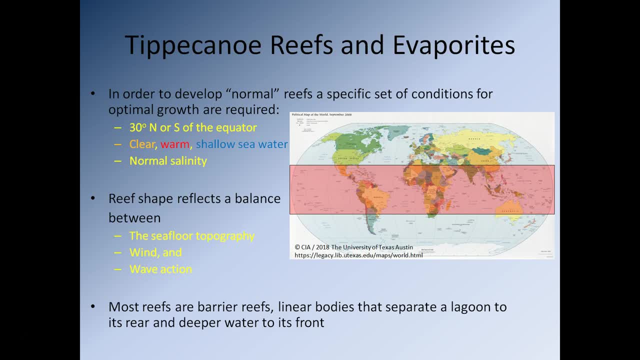 for optimal reef development. So if you want to form a reef, you really need to meet five criteria. The first situation is you typically need to be 30 degrees north or south of the equator. That means you're going to have water that's going to be of sufficient warmth. 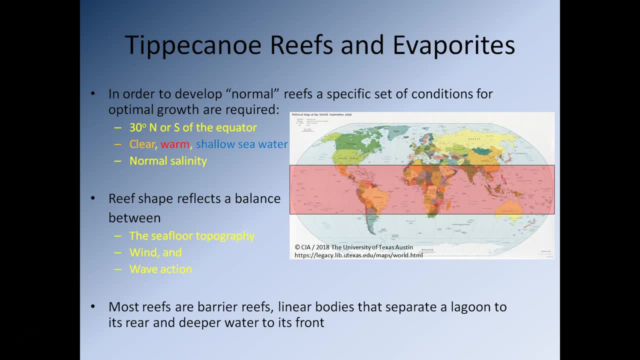 to allow large-scale coral formation. And coral formation is important because coral reefs form carbonate barriers and carbonate barriers protect the carbonate shelf carbonate lagoons that form behind them. You also need clear water, you need warm water and you need shallow water. 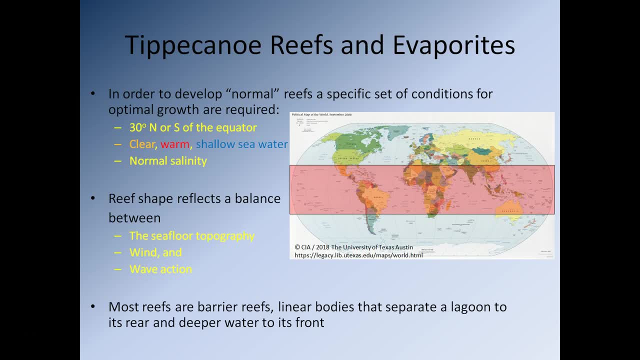 So that's water depths between 0 and 200 metres And of course you need the salinity to be normal. So the shape of the reef that forms will obviously be a reflection of the seafloor topography, And then obviously it will be also affected. 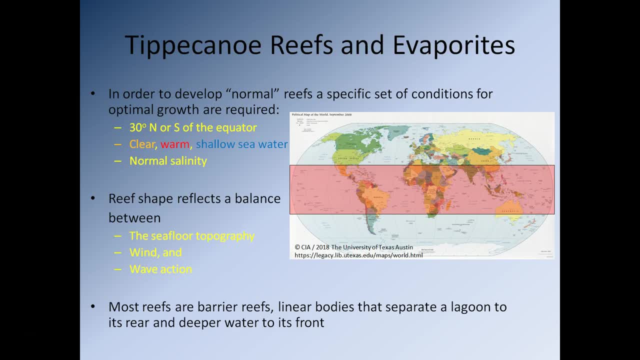 by wind direction, and wind direction obviously leads to waves, So the reef will also be shaped by wave action. And then, of course, the reef will also be shaped by waves, And most reefs that tend to form are what are referred to as barrier reefs. 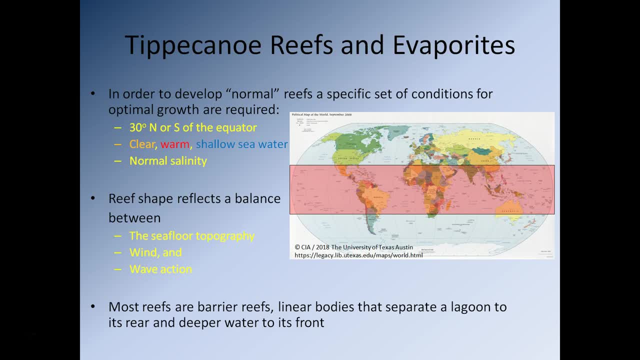 They are linear bodies and these barrier reefs will separate a lagoon, a carbonate lagoon behind the reef, from the deeper ocean in front of the reef. So the reef is all important to protecting the carbonate shelf behind it And that's why reef formation is key. 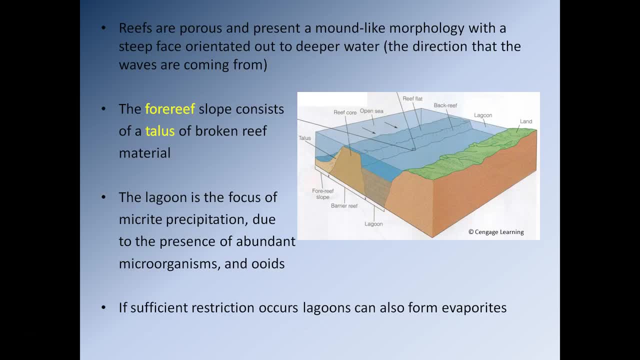 to the large-scale formation of carbonates. So you can kind of see it here in this diagram here. So here's our linear reef And you can see our linear reef is forming a natural barrier. So here we've got the open sea on this side. 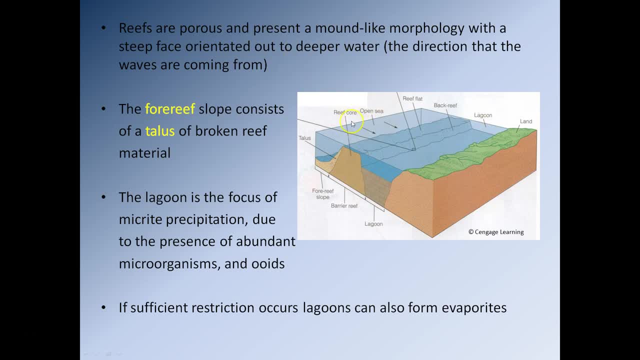 and the open sea is going to be pushing waves towards the reef, but the reef is going to act as a barrier and it's going to help to protect the carbonate lagoon behind it, And so it's in the carbonate lagoon where we're going to get large quantities. 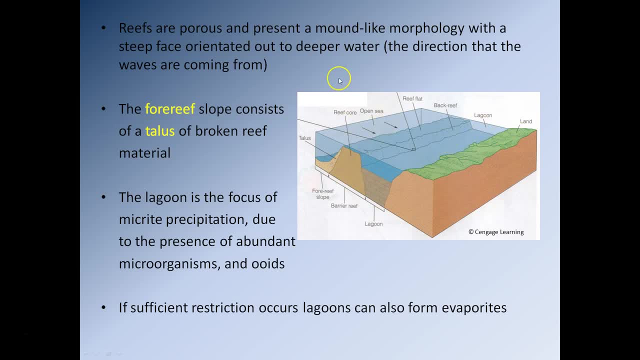 of carbonate forming. Now the reef itself is relatively porous and it presents a mound-like lithology with a steeply orientated face facing deeper water. And that steeply orientated because, of course, that's the site that's being hit by wave action. 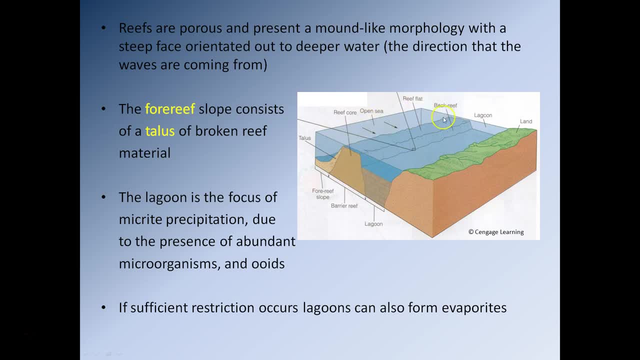 So that side is constantly being eroded and loose material is falling off this seaward face and it collects at the bottom, forming what we refer to as the talus. So the talus forms essentially in the fore reef, which is the area directly in front of the reef. 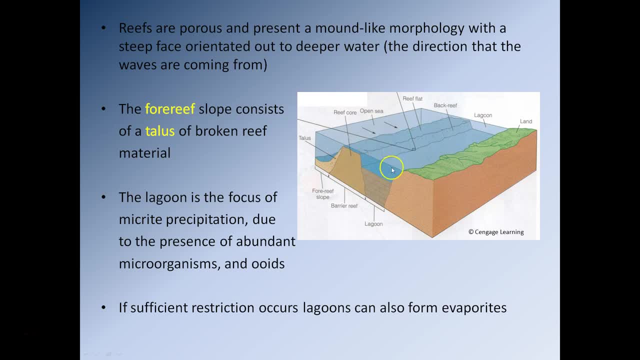 Okay. So that's why reef formation is all important, because we want to have these carbonate lagoons, because that's where we're going to form large quantities of limestones, And a lot of the limestones that form are dominated by micrite. 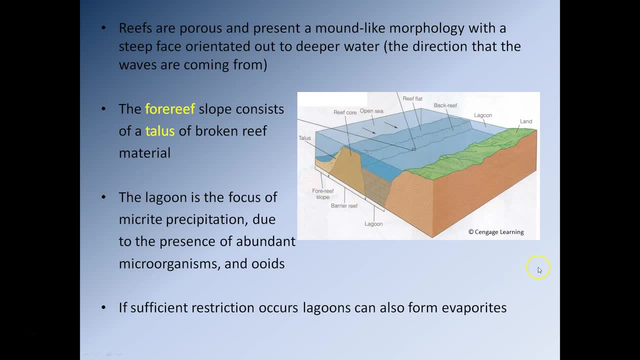 If you remember, micrite stands for microcrystalline calcite, so it's very, very fine-grained calcite. We're also going to get abundant microorganisms. we're going to get lots of photosynthesising blue-green algae in here. 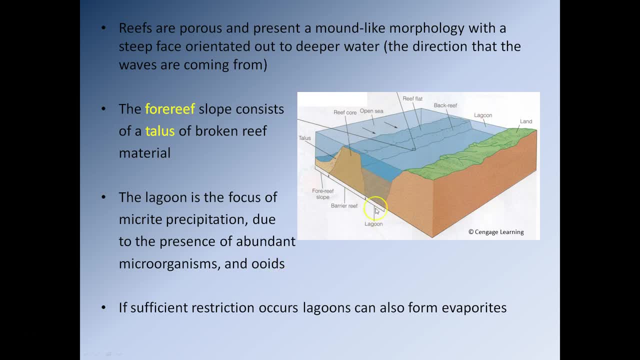 and we're also going to get lots of ooid formation in here as well, And obviously, if sufficient restriction occurs, this lagoon can evaporate away, producing layers of evaporites mixed in with the carbonates. So reef formation in the Cambrian. 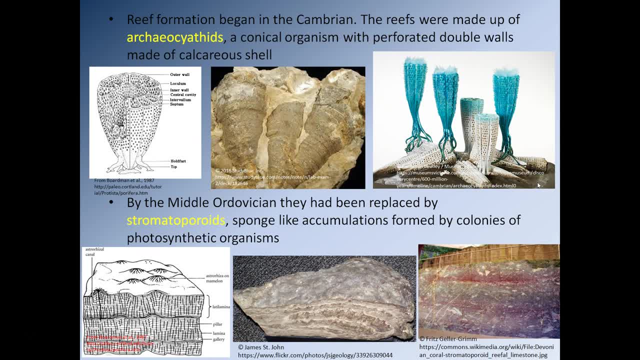 was dominated by one type of organism, that's the archaeocytids, which I probably pronounced massively incorrectly, And they are conical-shaped organisms. they had perforated walls and they had shells made of calcium carbonate. You can kind of see them here. 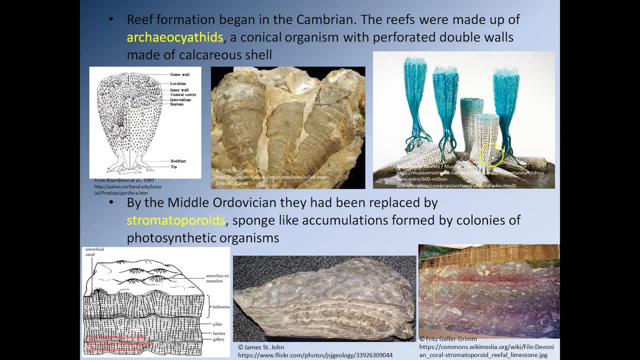 that's a general sketch of one. Here's a fossil and you can kind of see this is a model showing you how they would have grown. Now, the archaeocytids didn't actually make it out of the Cambrian, So by the time we make it into the Ordovician, 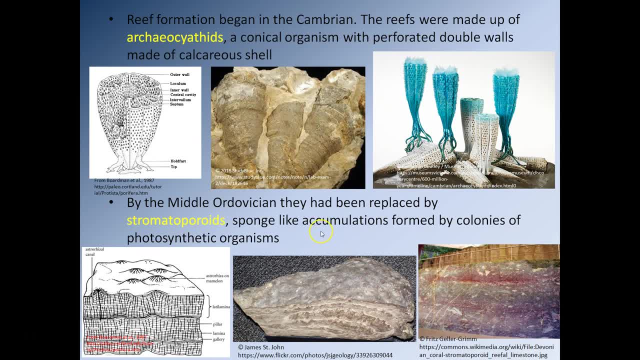 the archaeocytids are gone and they're replaced by the stromatopoids, Or should I say stromatopoids, And they are sponge-like accumulations formed by colonies of photosynthetic organisms. So essentially just kind of imagine. 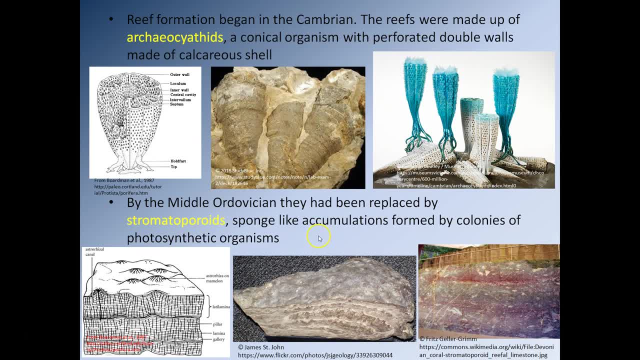 a giant stromatolite, almost a giant linear stromatolite, or giant mounds of stromatolites forming the barrier here, forming the reef, And so you can see this is a diagram of them. 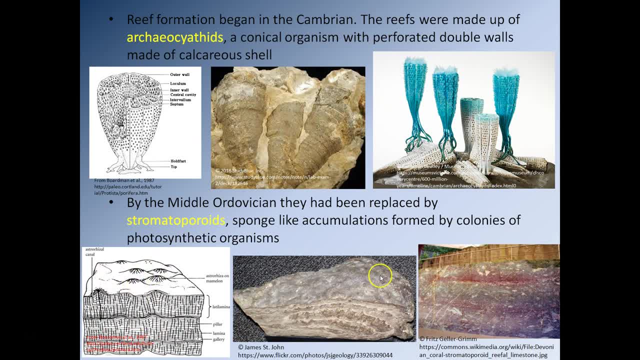 you can see they form layer after layer after layer. they have this very distinctive lumpy appearance on the top. you can kind of see on the fossil here how it looks rather lumpy on the top there and you can see the layering underneath. 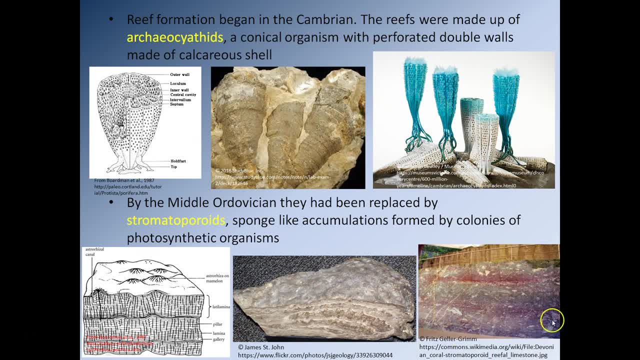 And this kind of shows you here a section through one of these stromatopoids- stromatopoid reefs- you can see that it consists of lots of broken up pieces of stromatopoids mixed in with lots of these nicely layered stromatopoids. 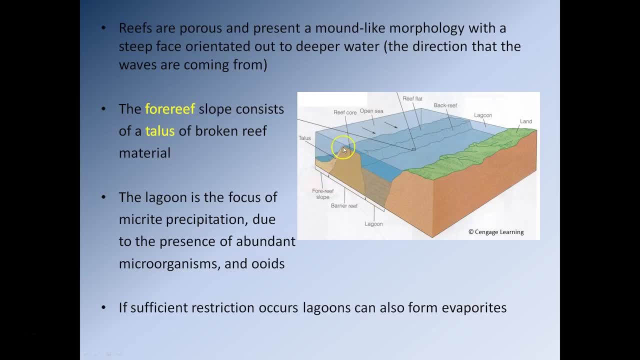 So this area here, this diagram here, probably represents more of this kind of four-reef environment with bits of falling off the reef. Now, in the case of the archaeocytids, the reefs that were forming were linear, They were long. 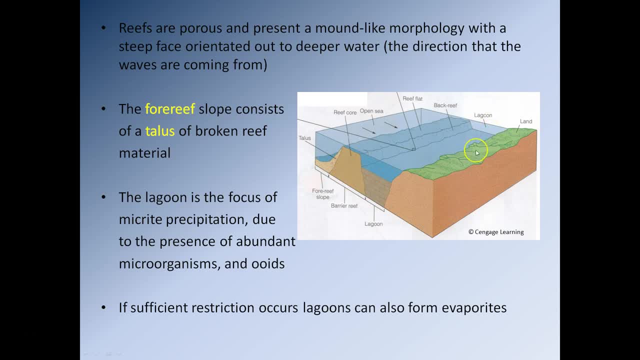 they were long, linear, continuous bodies. In the case of the stromatopoids, they would have been arguably referred to as patch or mound reefs. So it wouldn't have been a linear body, it would have been lots and lots of mounds, essentially. 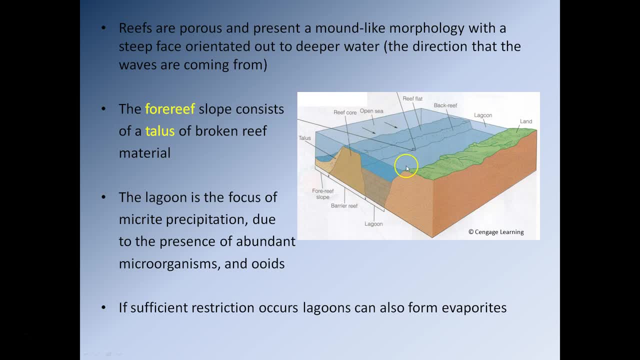 all in the same kind of area, acting as a barrier. You know, if you get enough mounds close enough to each other, they will obviously form a linear barrier. well, a linear-like barrier that will offer protection to the lagoon. 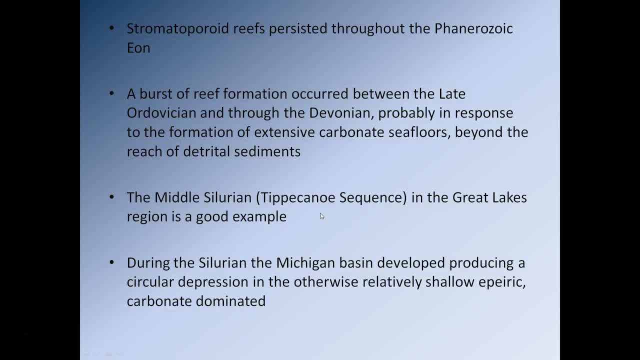 from the open ocean. So the stromatopoids reefs persisted throughout the Phanerozoic. so you know they make their appearance in the Ordovician. they continue all the way through the Phanerozoic. 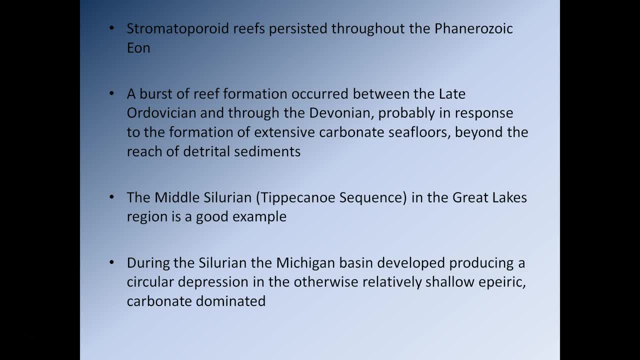 and we get a burst of reef formation occurring between the late Ordovician and through to the Devonian and that's probably in response to the formation of these nice shallow seas as part of the Tippecanoe marine transgression And obviously because you know. 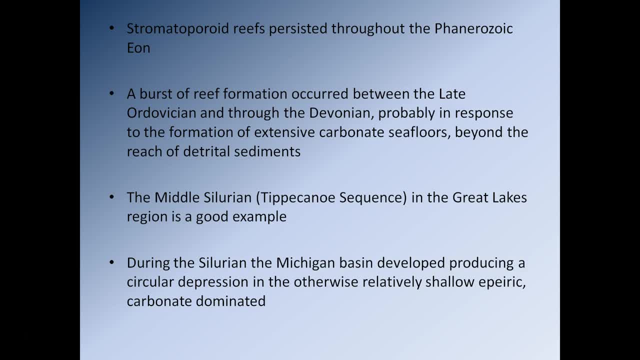 Tippecanoe marine transgression covers over such large areas, such large quantities of Laurentia, it obviously causes the amount of detrital sediment being deposited into the oceans to drop off significantly, producing very, very good water quality, which is great for reef formation. 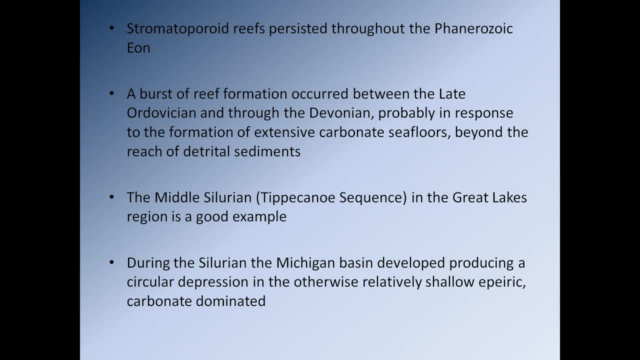 So the Middle Silurian we have the Great Lakes region is a really good example of what's going on. So during the Silurian, the Michigan Basin developed, producing a circular depression on what was an relative otherwise a relatively shallow Epiric carbonate-dominated sea. 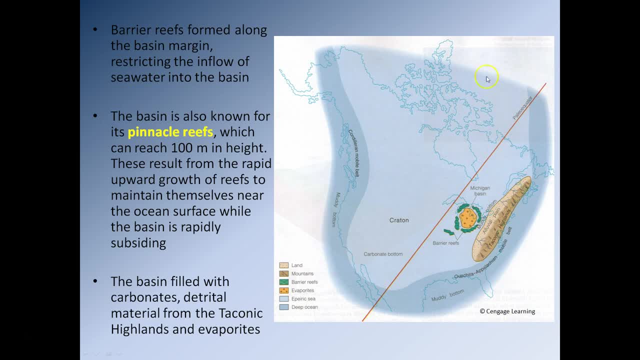 So here we go. So this is the situation. So here we have the Tippecanoe transgression. Most of North America, Laurentia, is underwater, The sea is relatively shallow, relatively detrital, sediment-free, and so we have the formation. 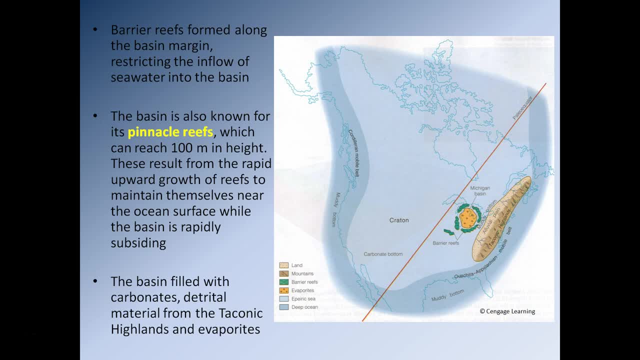 of a very, very large carbonate shelf producing huge quantities of carbonate. Now, on this carbonate shelf, we have the formation of a depression on the sea floor and that depression begins to fill with sediment. Now, along the margins of this depression, 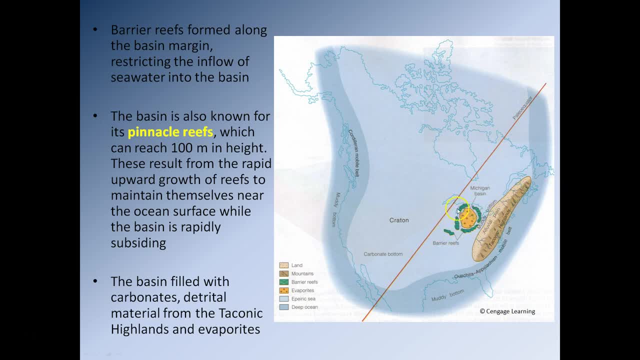 we get the formation of lots and lots of reefs, And so the reefs build up along the margin of the basin that's forming the Michigan Basin and eventually those reefs start to link up, and those reefs slowly link up and they form a continuous circle. 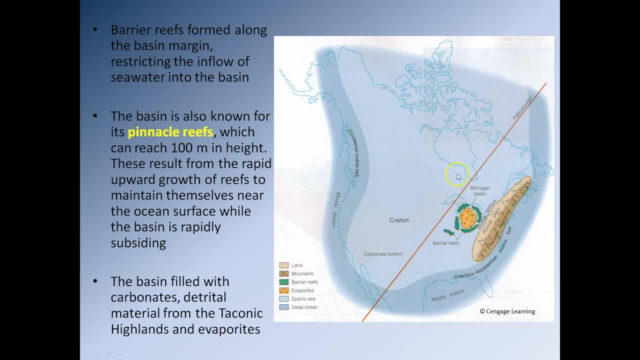 around the margin of the Michigan Basin, essentially isolating it from the rest of the Epiric Sea, And that's going to become very, very important Because it's going to restrict the inflow of seawater into this basin. So the basin is also known for its pinnacle reefs. 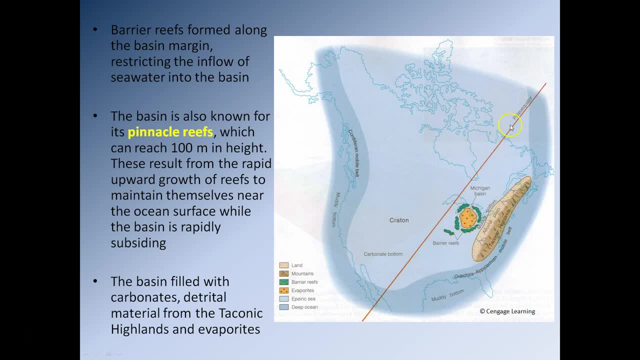 So these are very, very small reefs that occur within the basin itself And if you remember from the previous video, these basins that form, they are not. Sorry, it wasn't the previous video, it was the video before. They are not produced by tectonic shifts. 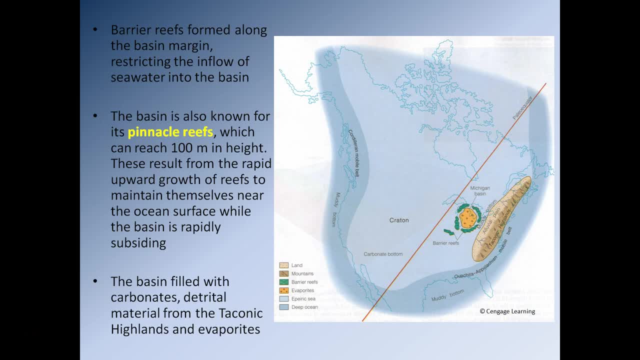 in the kind of, you know, plate tectonic fashion. They are produced by subsidence, So faults on the seafloor begin to move, creating a depression. That depression fills with sediment. The weight of that depression pushes the fault blocks down even further. 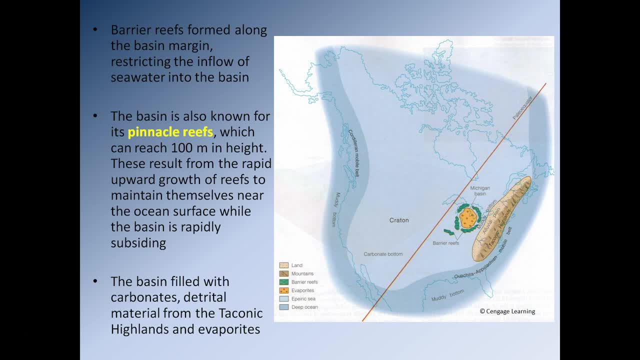 making the basin even deeper so it fills up with more sediment That weighs even more, pushing the fault blocks down even further, so the basin gets deeper, and so on. And so this meant as the Michigan Basin started to fill up with more and more sediment. 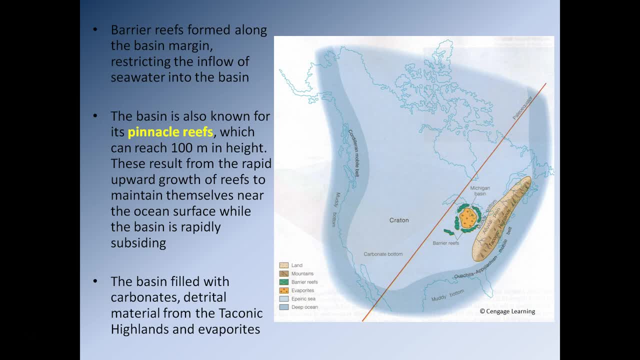 the floor of the basin started to get pushed further down and down and down. So this means that the reefs within the basin- well, the reefs obviously need to keep themselves. typically, you know within about, you know, minimum 200 metres. 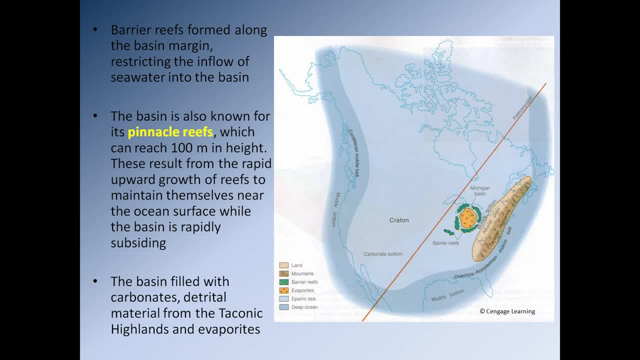 of the surface of the sea. So this meant that, as the seafloor subsided, the reefs had to grow upwards in order to stay within this 200 metre limit, And so what happens is the reefs within the Michigan Basin form these very, very large columns. 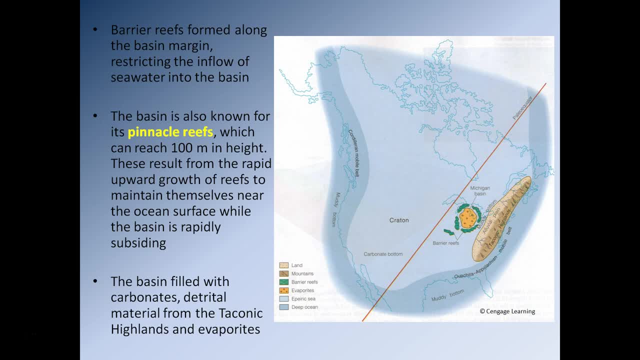 which we refer to as pinnacle reefs, because the reefs themselves are just growing upwards very, very quickly, and so they form this very, very distinct columnar form, and some of them can reach up to 100 metres in height, And so that's showing you that the basin is subsiding. 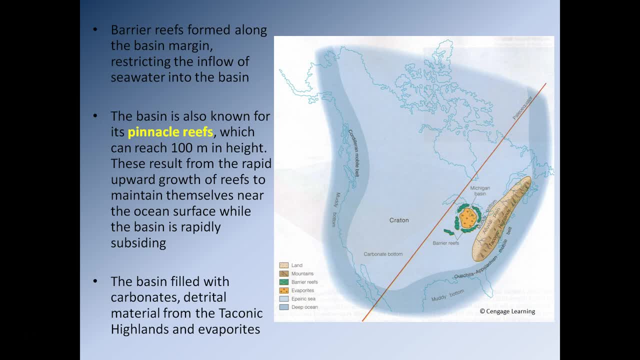 That's a good indicator that the floor of the Michigan Basin is dropping down Now, in terms of the basin itself, it filled with carbonates, but it also filled with detrital material coming off the Taconic Highlands. The Taconic Highlands is right here. 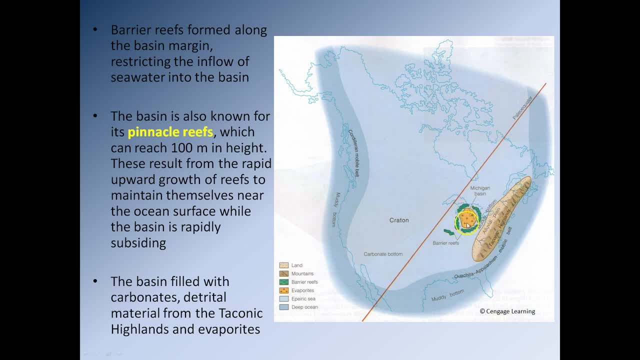 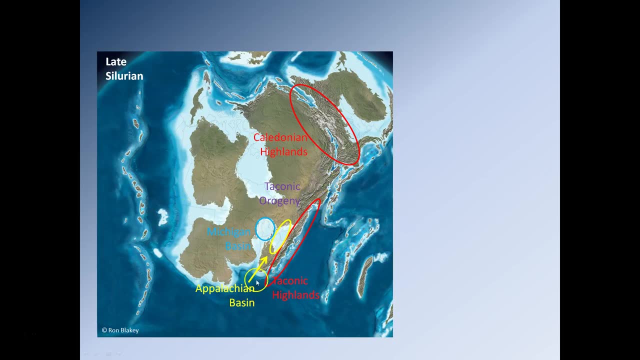 producing lots and lots of clastic material, and some of that made its way into the Michigan Basin as well. So here we go. so this is our situation. so this is the Lake Silurian. we have Taconic Highlands here. 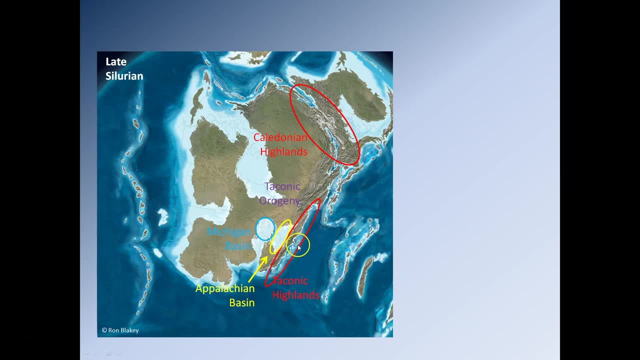 we have the Caledonian Highlands up here where Baltica's hitting Laurentia, we have the Appalachian Basin here, directly behind the Taconic Highlands, and we have the Michigan Basin right here, And so we have sediment coming off the Taconic Highlands. 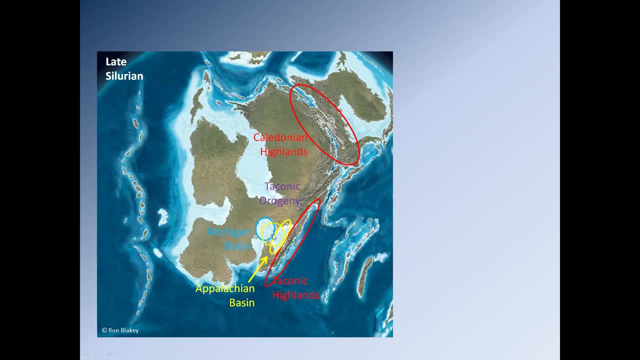 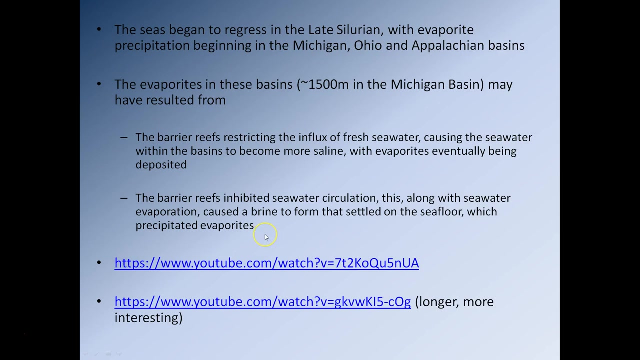 coming across and entering into the Michigan Basin. but you can see the Michigan Basin itself is isolated and it's being cut off by a ring of reefs that form along the margin of the basin, So the sea begins to regress in the Lake Silurian. 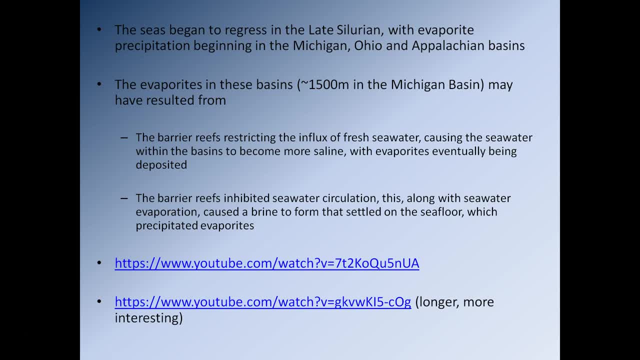 with evaporite precipitation beginning in the Michigan, Ohio and Appalachian Basins. So as the sea begins to regress, essentially the basin itself begins to become cut off. And so this means that as the basin begins to become cut off, you all of a sudden 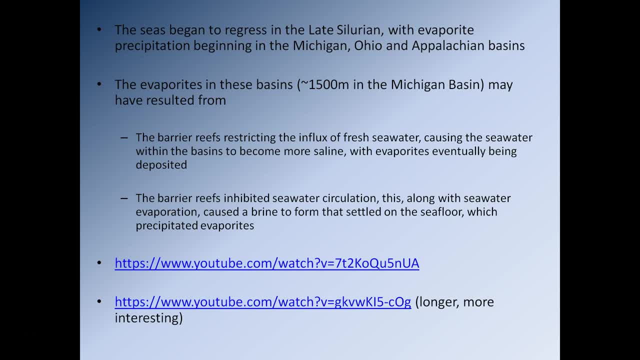 begin to end up with an isolated body of water in a hot environment, and so you begin to get the formation of evaporites, And the evaporites in the Michigan Basin form a layer that's approximately 1,500 metres thick, so one and a half kilometres give or take a little bit. 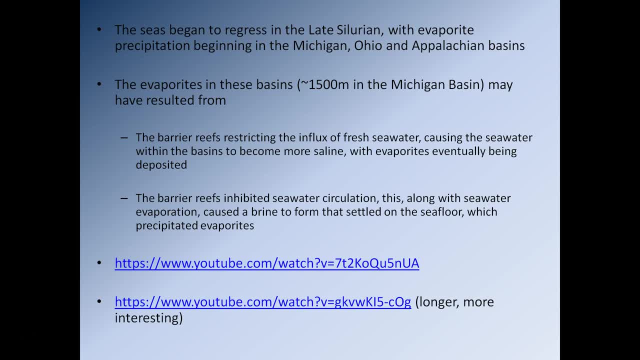 So, in terms of the actual formation of the evaporite layer, it could have occurred in one of two ways. The first way is simply the barrier reef restricted the influx of fresh sea water into the basin. That obviously meant the basin became restricted. the water evaporated. 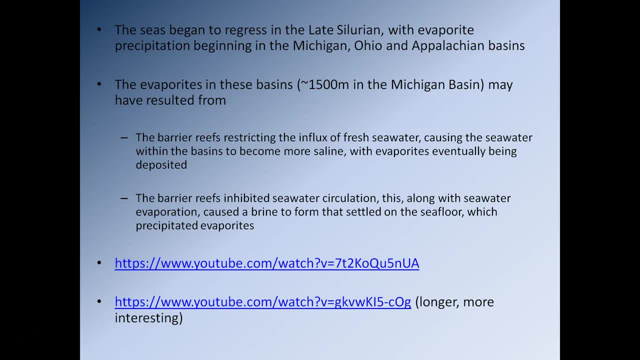 away, the water became more saline and eventually that led to the deposition of evaporites. as you know, essentially the water became saturated with respect to minerals like gypsum and salt, Or should I say halite. So that's one way that it could have formed. 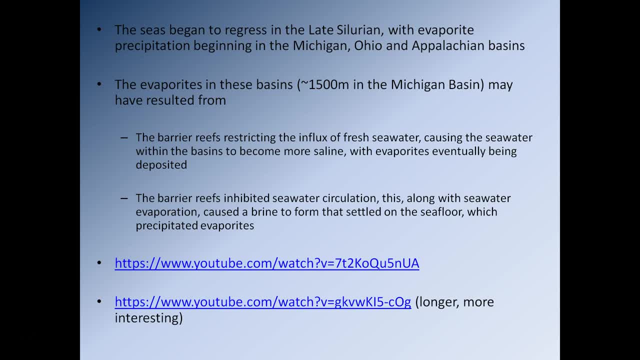 The other way that these evaporite layers could have formed is once again same situation. the basin becomes isolated due to the reefs, the water begins to evaporate away, and so that means the water steadily becomes more and more salt rich. for instance, It becomes more and more rich in dissolved 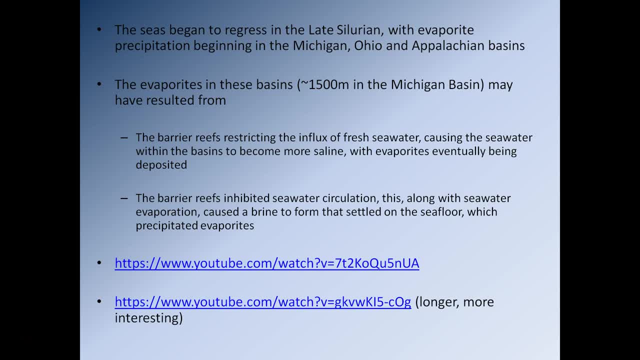 minerals, as more and more of the water is lost. Now this means that some of the water in the basin is going to become very, very heavy, because it has lots and lots of dissolved constituents in it, and so this heavy water is going to naturally sink to the bottom. 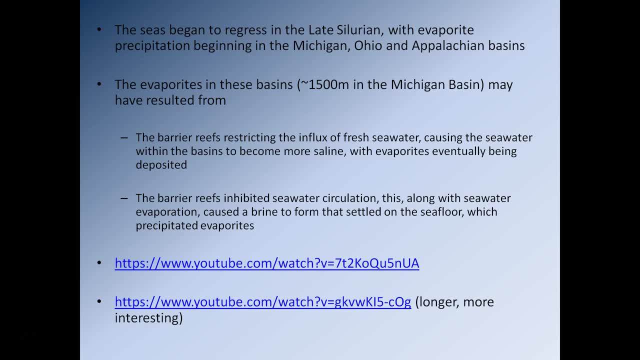 of the basin where it forms a brine, And this brine can then directly precipitate evaporate minerals onto the seafloor. So you have this layer of brine sitting at the bottom of the Michigan basin and that will be directly precipitating. 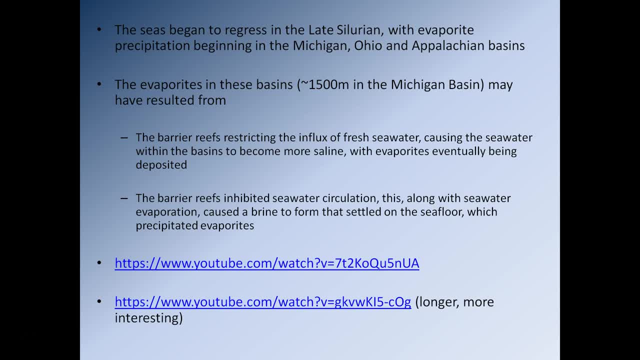 evaporate minerals onto the seafloor, So that's another way this could have happened. Now, as part of the lab, we are going to watch these videos here together and we're going to discuss what you can see, If you want to watch them beforehand, that's. 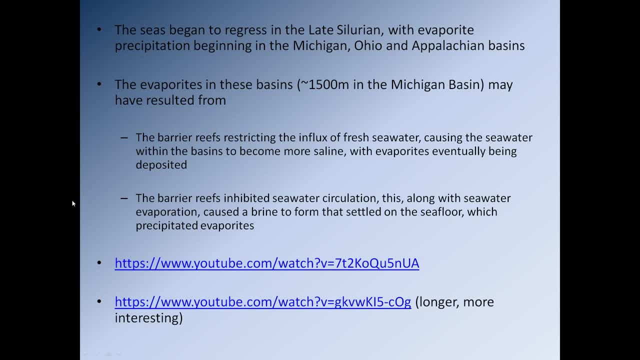 fine. What you're going to see is you're going to see a group of scientists. they're on the floor of the Gulf of Mexico, they've got a rover and they're going around looking at the brines that are forming in the Gulf of Mexico. This one here. 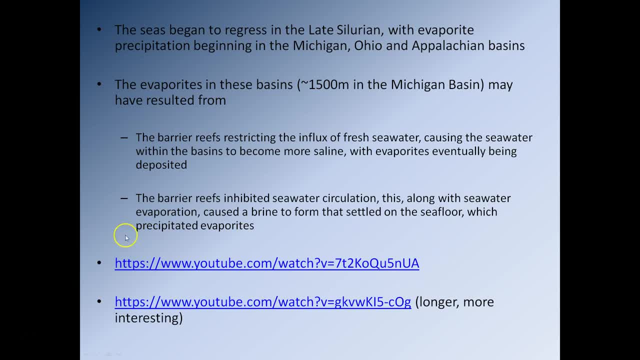 is going to essentially allow you to look at the density difference between the standard sea water and the brine, And this one here is going to show you an area of brine that essentially is producing its own evaporite minerals on the seafloor, despite being several. 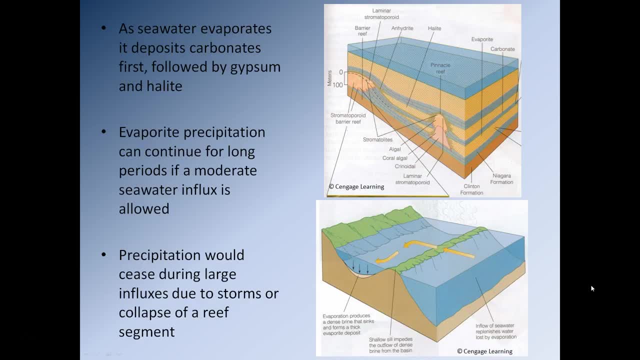 hundred metres under water. So, regardless of how the evaporite is actually formed, as the sea water evaporated away, we would get deposits of carbonate, initially followed by gypsum and then followed by halite. So we're going to get a layer of carbonate and then a layer of gypsum. 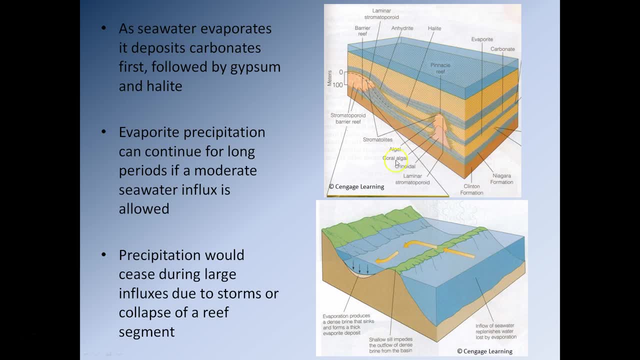 and a layer of gypsum and halite over the top, Then what's going to happen is, every once in a while, the reef is going to fail and that's going to allow a sudden influx of fresh sea water into the basin. That's going to stop evaporite precipitation. 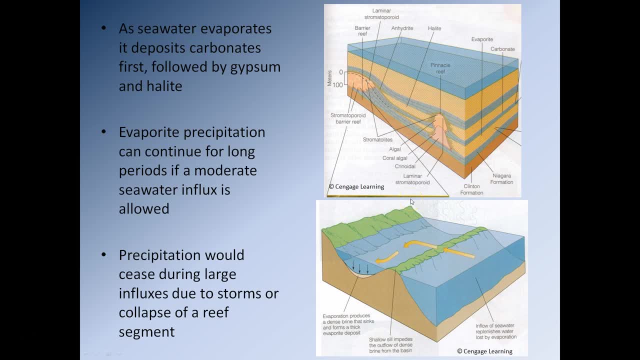 At that point we're going to go back into carbonate deposition And then, obviously, the reef's going to repair itself. the fresh sea water can no longer come in. That's going to mean eventually we're going to get back to the point where we get evaporite. 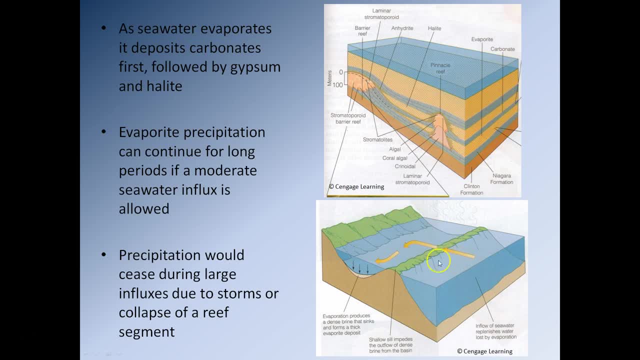 precipitation: again The reef's going to fail. new sea water comes in, stops evaporite deposition, so we're back to carbonate deposition And then eventually the reef's going to repair itself. large scale evaporation: again, that's going to lead to the formation. 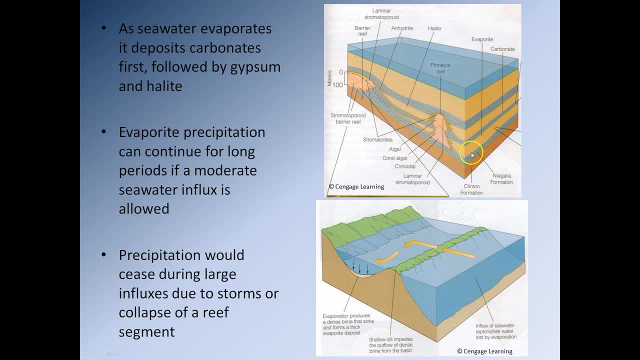 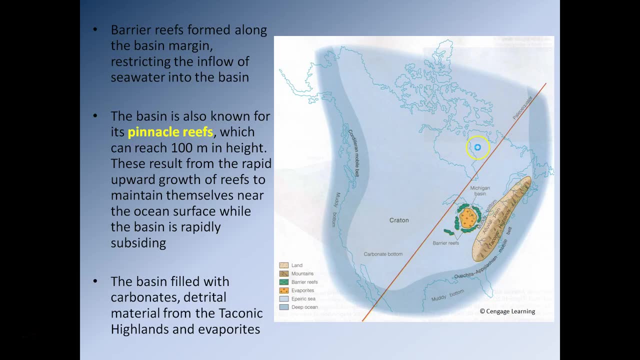 of evaporites. And so if we look at the Michigan Basin sequence, we have layers of carbonates followed by evaporite carbonate, evaporite carbonate, evaporite, obviously with layers of sandstone and mudstone mixed into the sequence coming from the 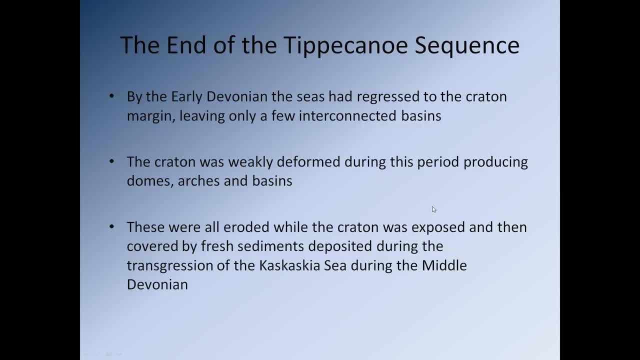 erosion of the Taconic Highlands. So what happens at the end of the Tippecanoe sequence? Well, by the early Devonian, the sea had regressed to the Craton margin, leaving only a few interconnected basins. So the Craton 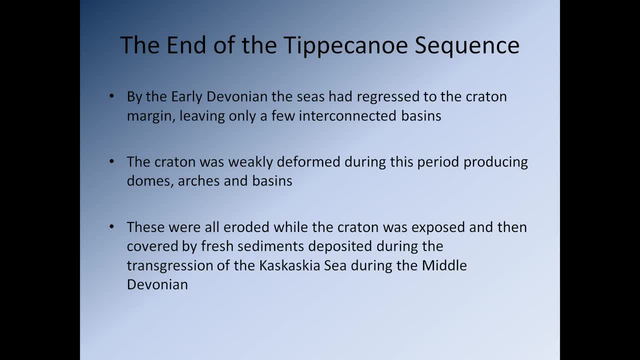 was weakly deformed during this period, producing domes, arches and basins. so during this time frame, the Craton is getting very, very weakly deformed, producing very, very large, broad anticlines and synclines. 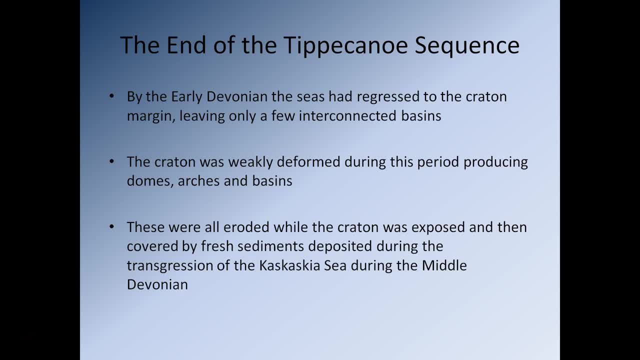 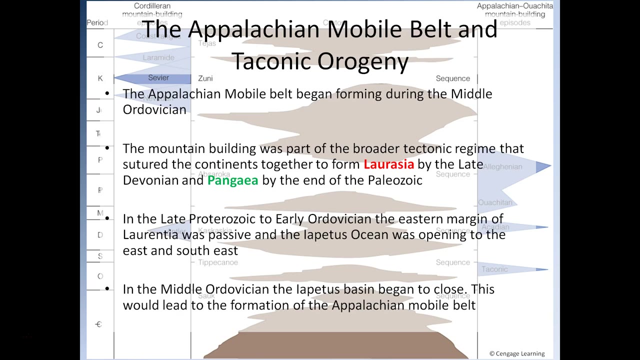 And these anticlines especially, were eroded, while the Craton was exposed and then covered by fresh sediments deposited during the transgression of the Kaskaskia Sea during the Middle Devonian. Okay, so let's have a moment. let's take a moment to actually 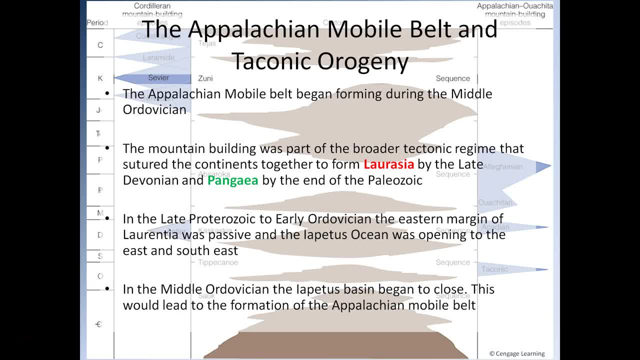 take a break because I have run long. I apologise for that. So let's stop the presentation here. take a couple of minutes, get up, have a walk around, go and get a glass of water and please return, Alright, so during. 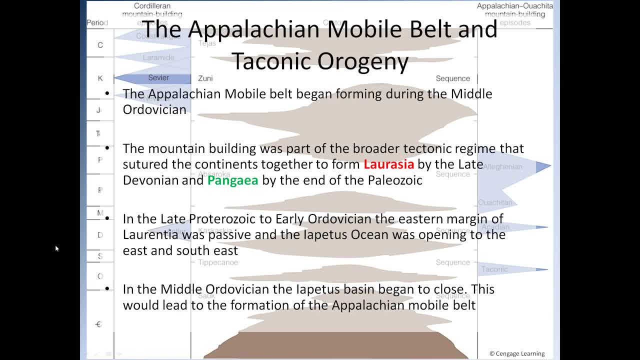 the Paleozoic, we begin to see the formation of the Appalachian Mobile Belt on what is now the modern eastern side of North America. So the Appalachian Mobile Belt began to form during the Middle Ordovician. Now it's not just one event, it actually consists of, you know, 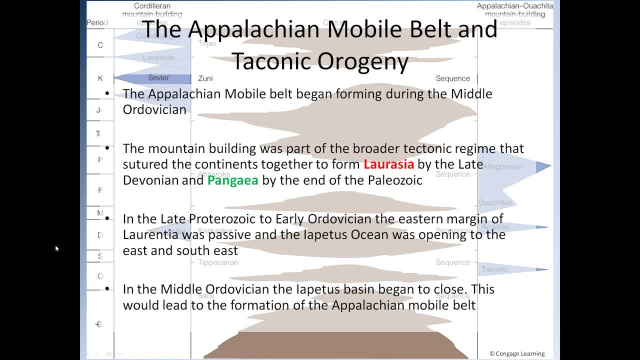 arguably three, maybe four separate orogenic events that all combine together to give us the Appalachian Mobile Belt. So you know, that's another reason why it's referred to as the Appalachian Mobile Belt, because it's not one event. it occurs in, you know, several different events. 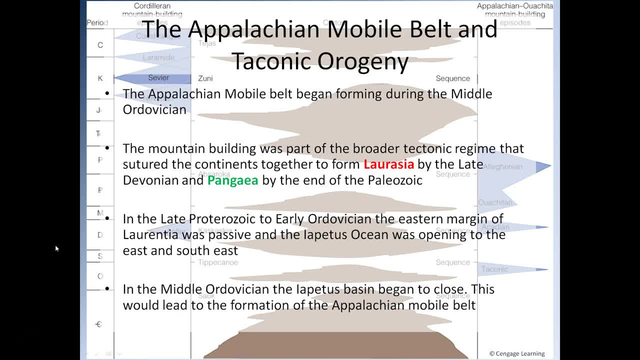 occurring in slightly different locations, meaning the belt isn't actually 100% stationary. So the mountain building was part of the broader tectonic regime that sutured the continents together to form Laurasia by the late Devonian and Pangaea by the end of the Paleozoic. 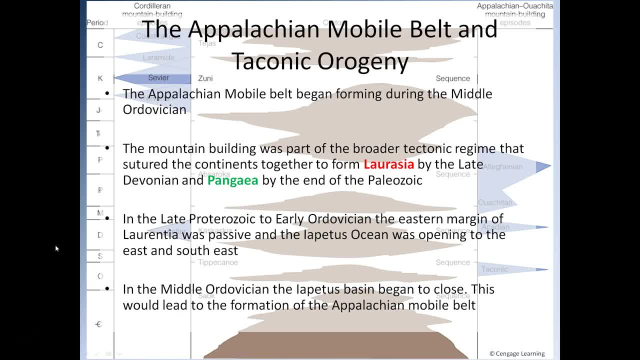 So Laurasia forms when we have the collision of Laurentia and Baltica. So Laurentia and Baltica and, to be honest, Avalonia, combined together gives us Laurasia, And then that's formed by the late Devonian, And then after that we then 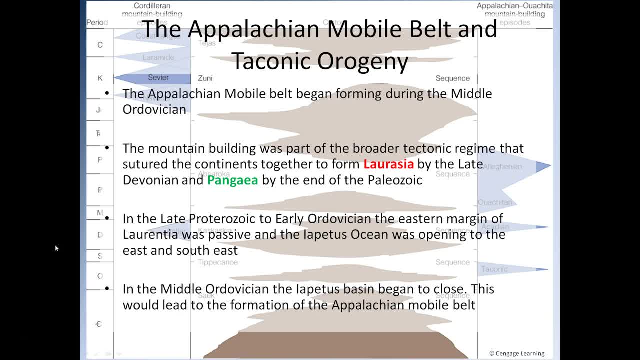 have the collision of Laurasia with Gondwana and that gives us the supercontinent Pangaea. So in the late Proterozoic to early Ordovician the eastern margin of Laurentia was passive and the Iapetus Ocean was opening to the 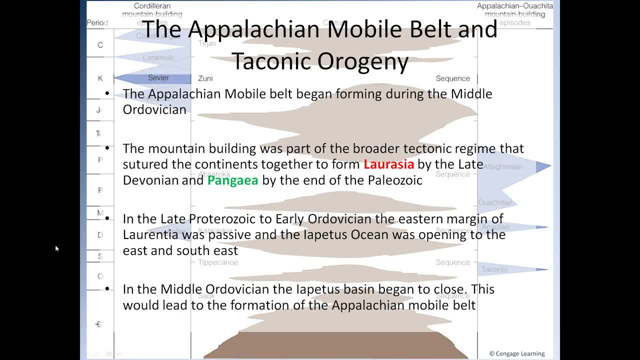 east and to the south, So by all the way through to the early Ordovician along what is now the modern east coast of North America. we had a nice big ocean basin there called the Iapetus Ocean, Not as big as the Atlantic but still pretty. 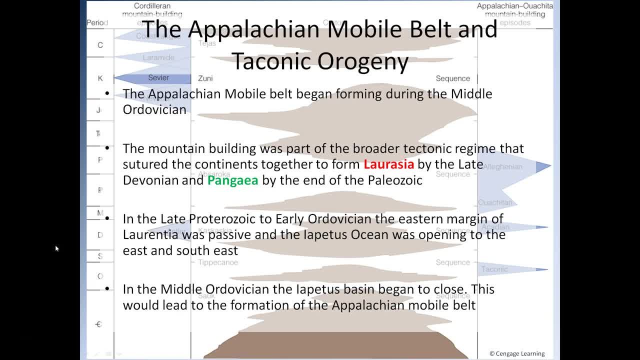 big. So in the middle Ordovician the Iapetus Ocean began to close, So a subduction zone opens up and the sea floor of the Iapetus Ocean begins to be destroyed And so that begins to bring Laurentia and Baltica towards. 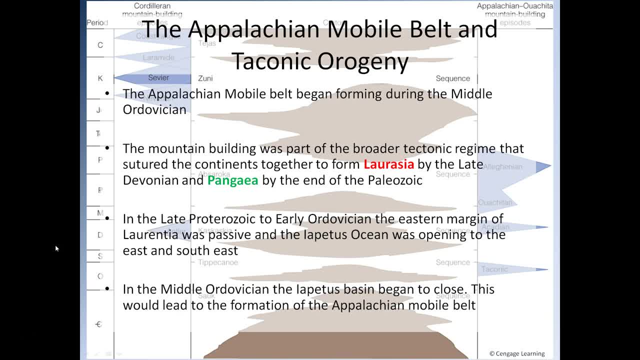 each other. They start moving towards each other as the ocean crusts between them begins to become destroyed. So this collision, initially, is going to lead to the early stages of the formation of the Appalachian Mobile Belt, And so you can see it here. so these 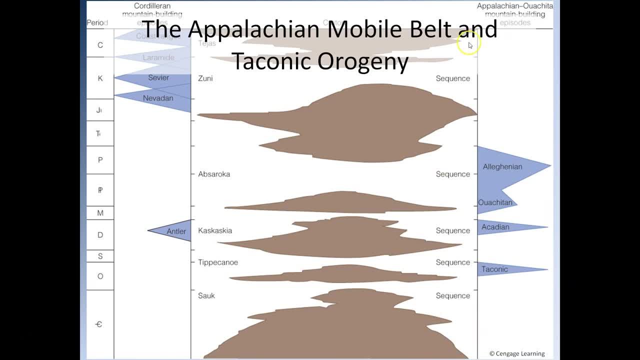 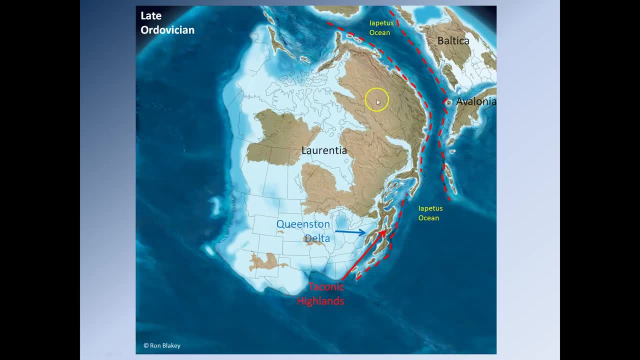 essentially, these orogenies combined are going to end up giving us the Appalachian Mobile Belt, Alright. so here's the basic situation in later Ordovician. So here's the Iapetus Ocean and we have subduction, and subduction is destroying the Iapetus Ocean and it's bringing 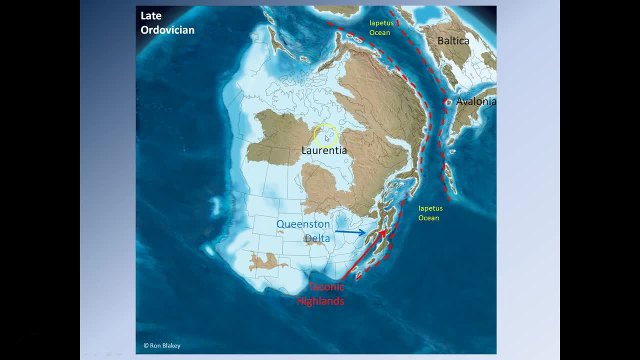 Baltica and Avalonia towards Laurentia And obviously there is going to be a collision. So along here we're going to end up with the Caledonian Orogeny and down here we're going to end up with the Taconic Highlands. 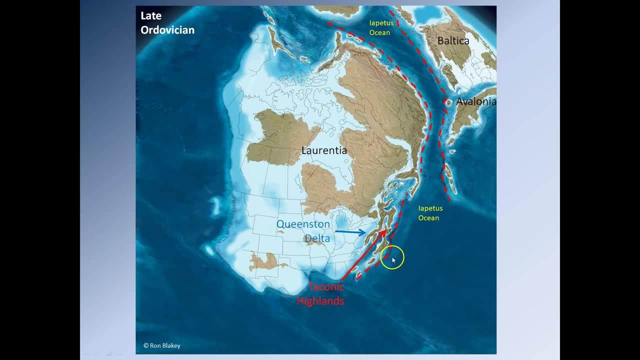 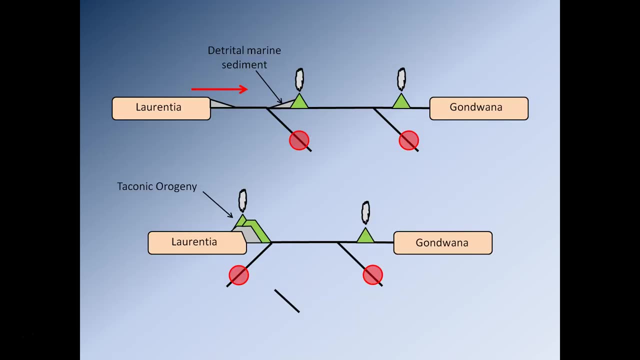 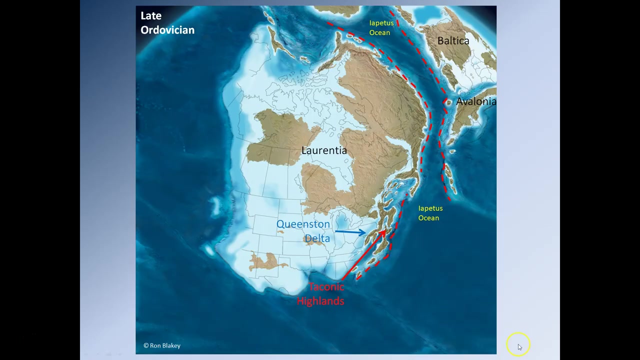 The Taconic Highlands is the opening stage, essentially, of the Appalachian Mobile Belt formation. So what's going on Now? this is a rather complicated situation. So you have to remember down here, down to the southeast, we actually have Gondwana. 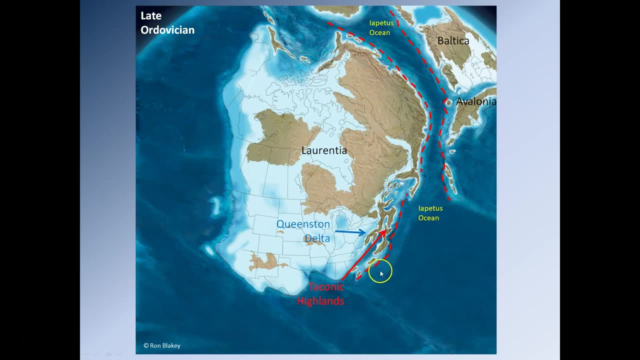 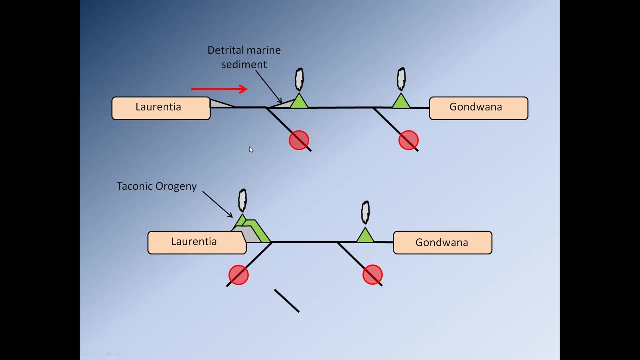 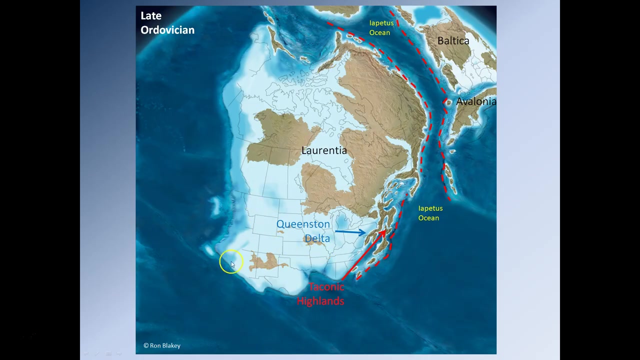 It's just down here, And so what's going on here to actually form the Taconic Highlands. So this rather interesting block diagram, drawn by yours truly, hopefully, will help to summarise what's going on. So here's Laurentia and here's Gondwana. 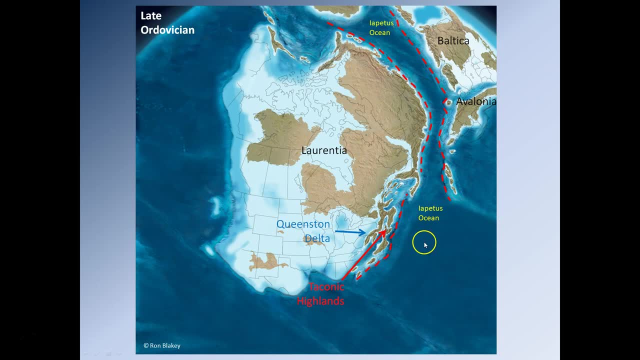 down here and in between we have a rather large body of water and we have a lot of oceanic crust in between. Now you can see Baltica and Avalonia heading this way. that's going to produce the Caledonian Highlands up here. So what's? 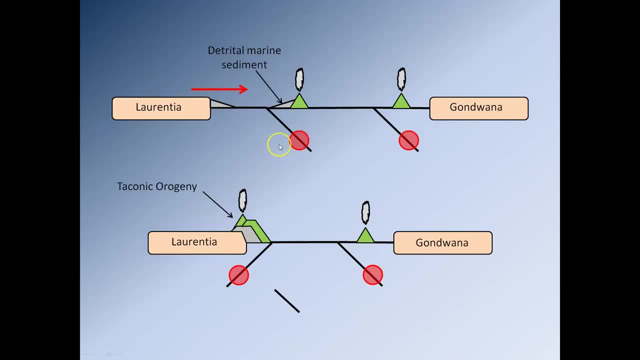 going on down here to give us the Taconic Highlands. Well, what happens is, initially we have Laurentia being eroded, sediment being deposited here along the what is now the eastern margin, and we have the oceanic crust start subducting down underneath. 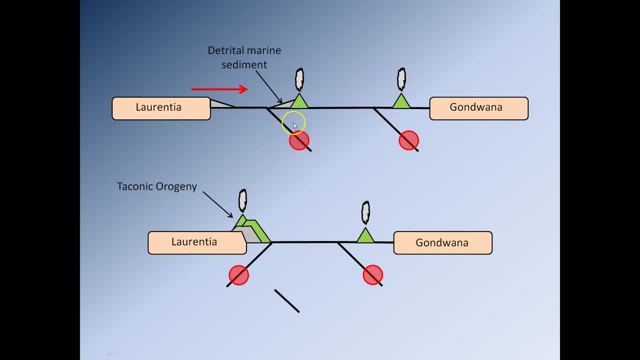 the oceanic crust of the Iapetus Ocean and that creates essentially a chain of volcanic islands sitting just off the coast of Laurentia. Now, because the oceanic crust is subducting down underneath here, it pulls Laurentia in this direction and obviously eventually, 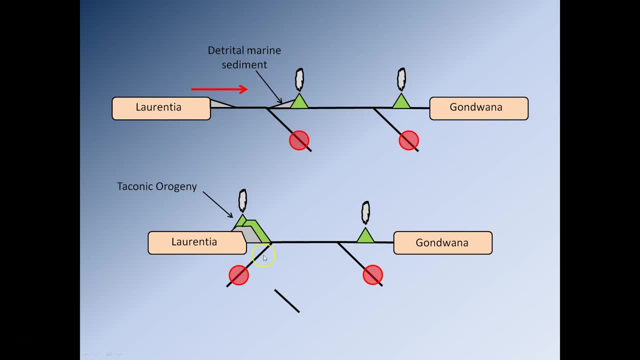 that leads to the collision of Laurentia with this island arc and that leads to the formation of the Taconic Highlands. Now, once this collision takes place, the direction of subduction shifts, so it was initially coming down towards what is now considered to be approximately the south. 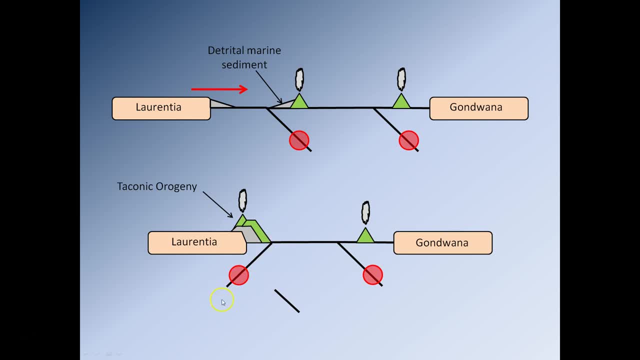 the direction of subduction shifts towards the north and that, of course, produces magma that rises up feeding volcanoes which are part of the Taconic Highlands, At the same time, towards Gondwana. we have a situation where we have subduction starting just in front of Gondwana. 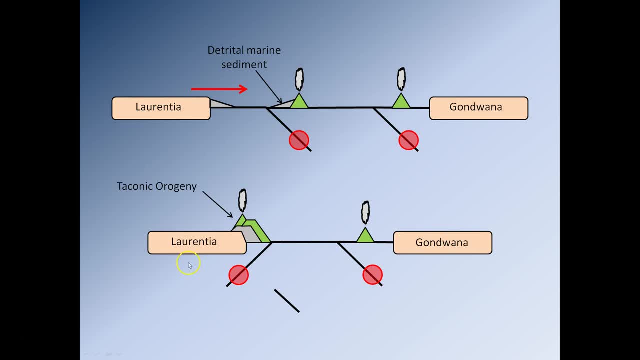 and that's also helping to destroy the oceanic crust that separates Laurentia and Gondwana and essentially it's leading to the eventual collision which is going to give us the complete Appalachian mobile belt. So it's not an easy one to understand. it's a rather 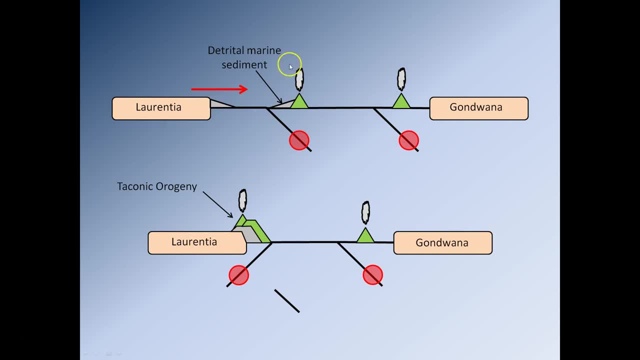 complicated orogeny. Essentially, all you need to understand is subduction produces a volcanic island arc sitting off the coast of Laurentia. Eventually, that subduction causes Laurentia to crash into the island arc, forming the Taconic Highlands, and then the direction of subduction shifts. 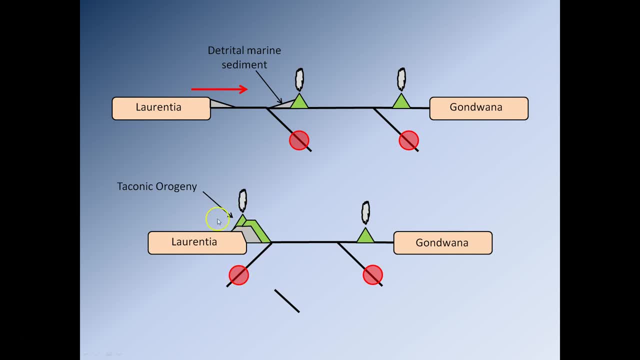 and then that creates magma that then feeds volcanoes within the Taconic Highlands. At the same time, we also have subduction on the other side of the ocean basin that's destroying oceanic crust over here by Gondwana and that's helping to destroy the oceanic crust. 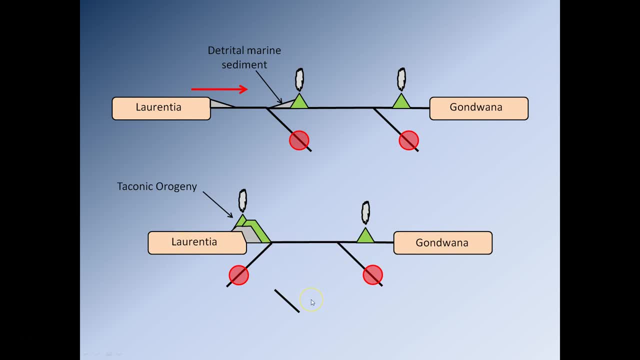 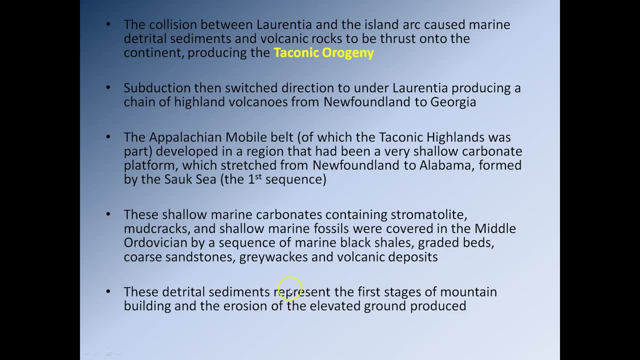 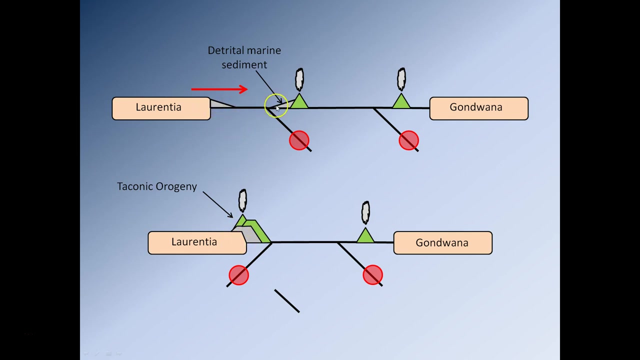 meaning that Gondwana is now on a collision course with Laurentia. So the collision between Laurentia and the island arc caused marine detrital sediments and volcanic rocks to be thrust onto the continent. So this grey block here is all the volcanic and detrital 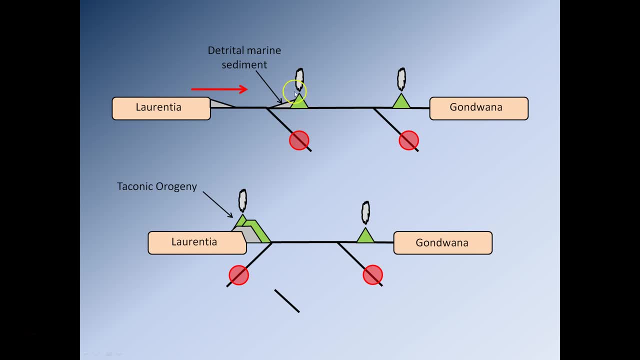 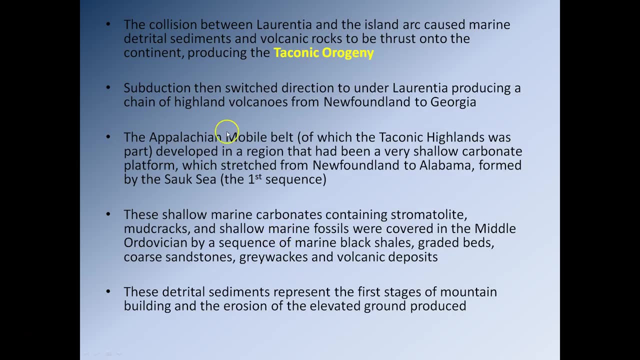 sediments that were in the ocean basin between Laurentia and the island arc. they get compressed and they get forced onto Laurentia, producing the Taconic Highlands. So subduction then switched direction to under Laurentia, producing a chain of highland volcanoes from Newfoundland to Georgia. 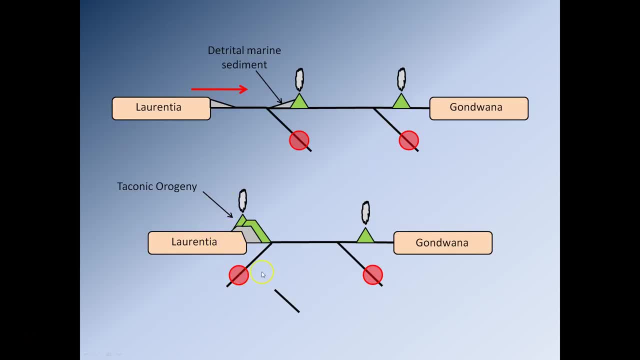 And so then, what happens is, once we have the initial highlands, we then have subduction shifts. magma is produced down here. that magma rises up, feeds volcanoes on the surface, so the Taconic Orogeny grows even larger as all of these volcanoes start putting. 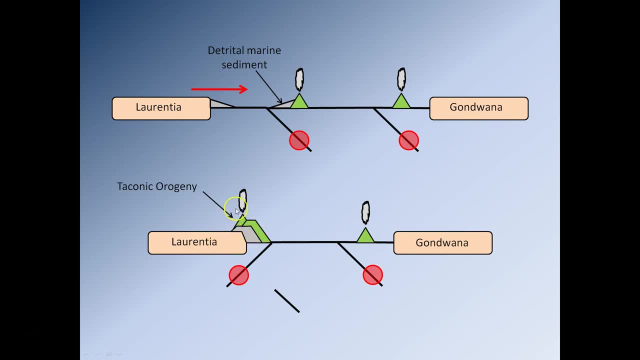 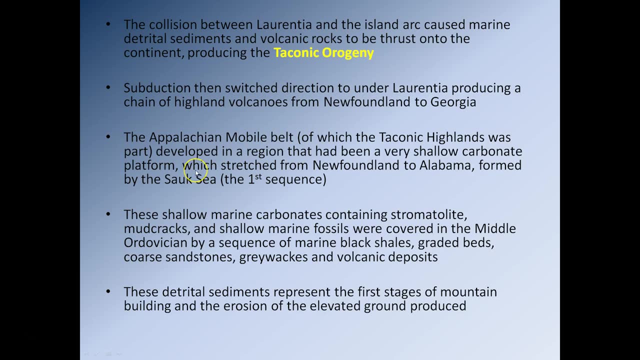 volcanic rocks into the highlands as well, helping to make them larger. So the Appalachian Mobile Belt, of which the Taconic Highlands was the first part, developed in a region that had been a relatively shallow carbonate platform, which stretched from Newfoundland to Alabama, and that was formed by the first 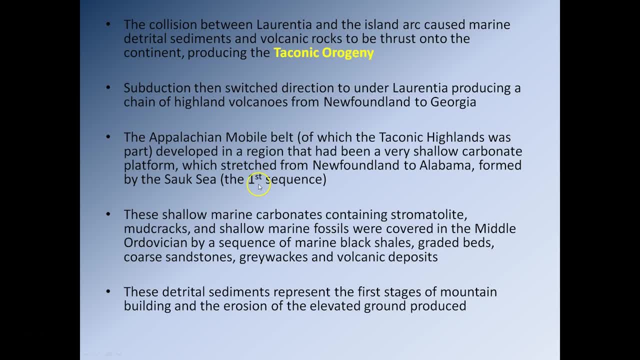 the first silk sea, the first marine transgression, and the shallow marine carbonates contained stromatolites, mud cracks and shallow marine fossils, and they were then covered in the middle Ordovician by a sequence of marine black shales, graded beds, coarse sandstones, grey wackies. 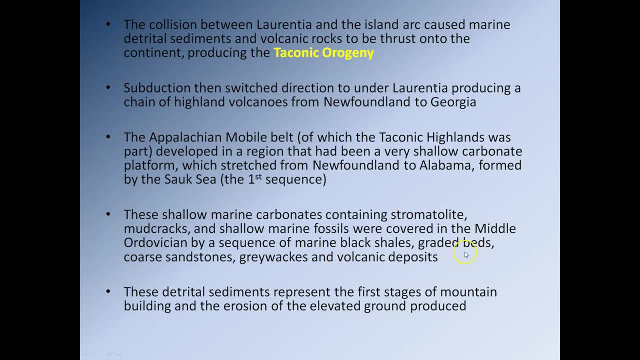 and volcanic deposits. So this is important. So what we've got is we have, essentially, a sequence of shallow marine carbonates that are forming in the early portion of the Paleozoic. so all the way through, from the middle Cambrian, all the way through, 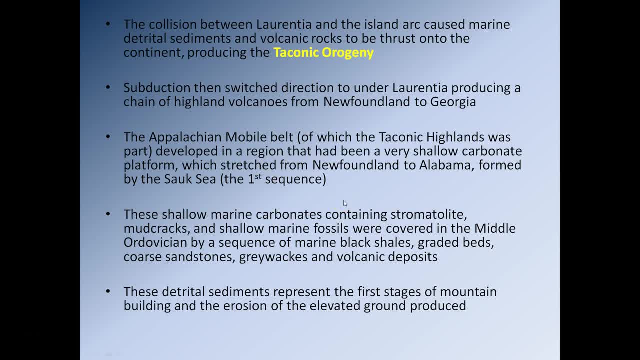 to the early Ordovician, that area is covered by a shallow sea, creating lots and lots of carbonates. and then, all of a sudden, in the middle Ordovician, that sequence of carbonates starts getting covered over by large quantities of clastic sediments and volcanic deposits. 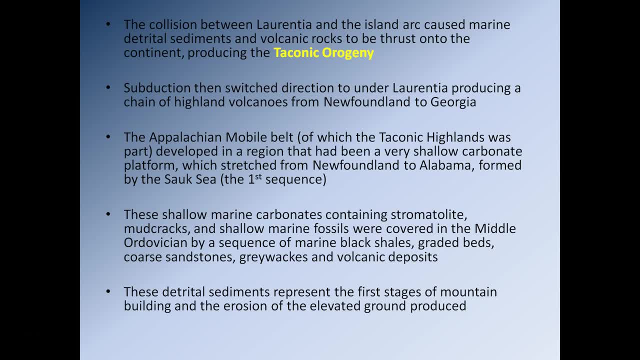 and so that's a very, very clear indicator that all of a sudden we have sediments, we have crust being pushed up above sea level and that crust is being eroded, producing these sandstones and grey wackies, and so that tells us very, very strongly that the 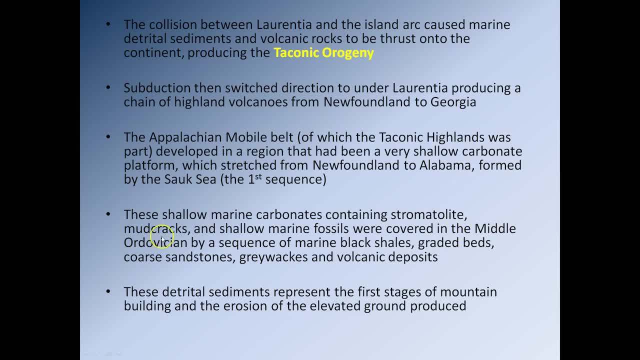 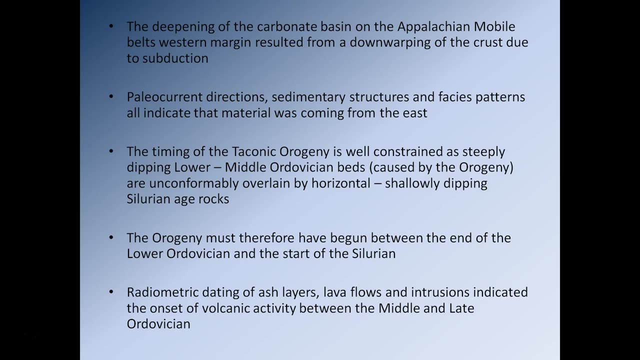 Ticonic Orogeny must have started in the middle Ordovician, So these detrital sediments represent the first stages of mountain building and the erosion of the elevated ground produced by the Ticonic Orogeny. So the deepening of 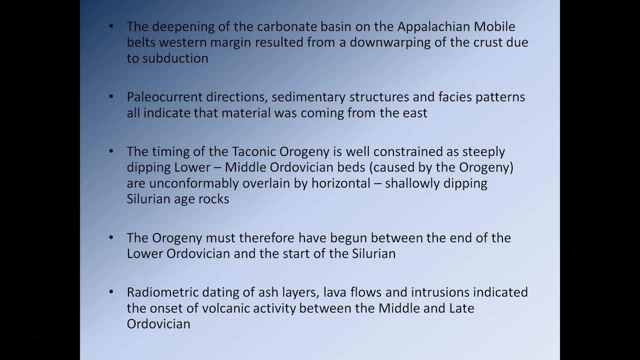 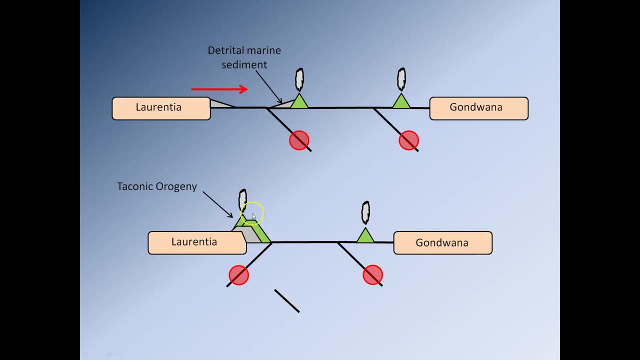 the carbonate basin on the Appalachian Mobile Belt's western margin resulted in a down warping of the crust due to subduction. So what are you talking about there, Chris? Well, the answer, the situation is that, if I just go back to this point here, so 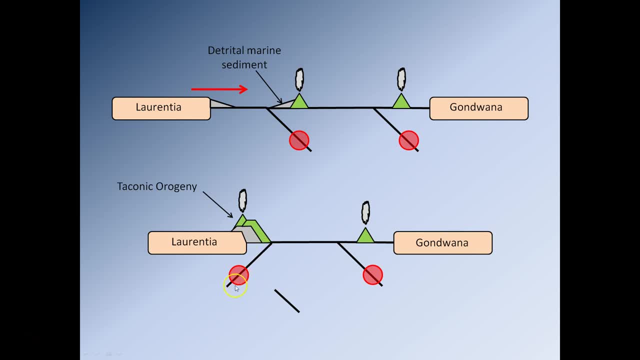 what's happening is that we have subduction now going underneath Laurentia, we have the Ticonic Highlands here and a portion of the crust back here behind the Ticonic Orogeny starts to essentially undergo warping. So it starts to warp downwards. so essentially you create. 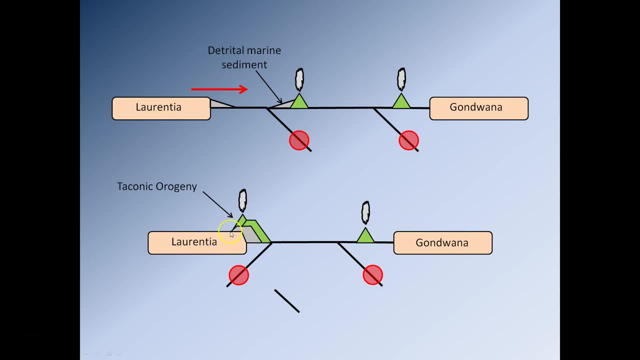 a depression here on the backside of the Ticonic Orogeny and that's going to become a basin, It's fault controlled, and so sediments are going to be eroded off the Ticonic Highlands here and they're going to enter this basin back. 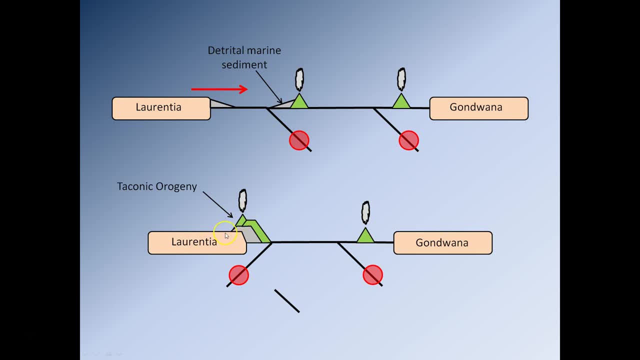 here and obviously, as we've discussed, as more and more sediment comes into the basin, that puts more weight on the basin floor, pushing the basin floor down, creating more room for more sediment to be added, which pushes the basin floor down further, and so on, And so this is what we begin to. 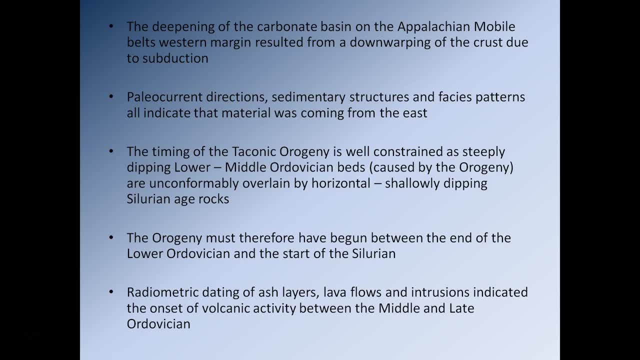 see forming on this rear side of the Ticonic Mobile Belt. So when we look at these sediments that are forming on what is now what we classify as the western side of the belt, we see paleocurrent directions, sedimentary structures and fasces. 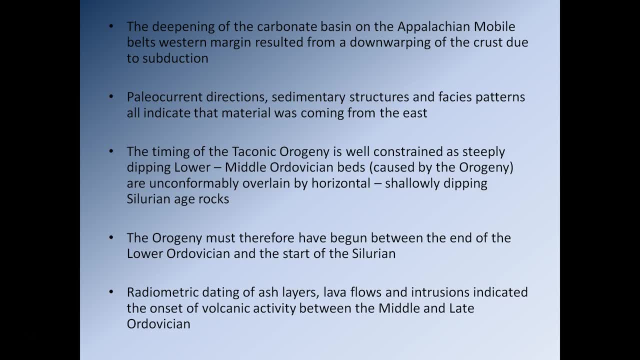 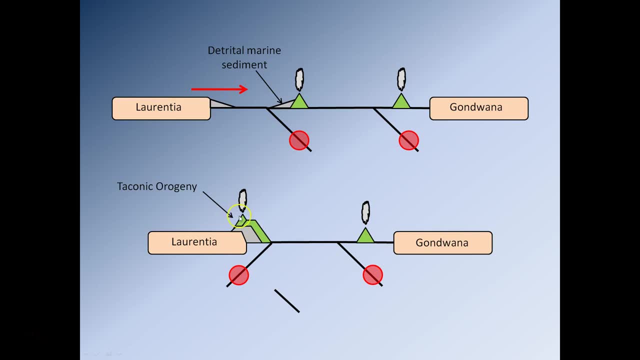 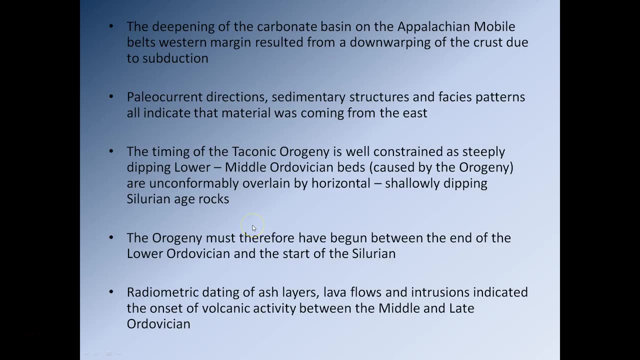 patterns, all indicating that material was coming from the east and coming into the basin. So of course, under modern orientations this is the east coast, so materials coming off the high ground here and entering into the basin coming from east to west. So that makes perfect sense. 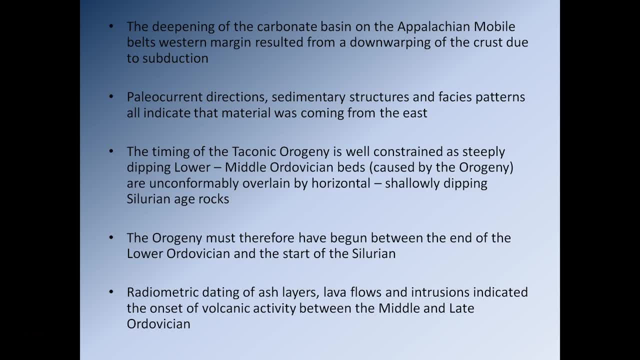 So the timing of this chronic orogeny is well constrained, and steeply dipping lower to middle ordovician beds caused by the orogeny are unconformably overlain by horizontal and shallow dipping silurian beds. So this gives us excellent timing dating information. 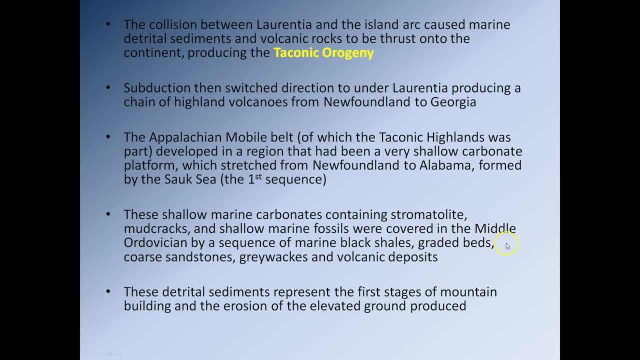 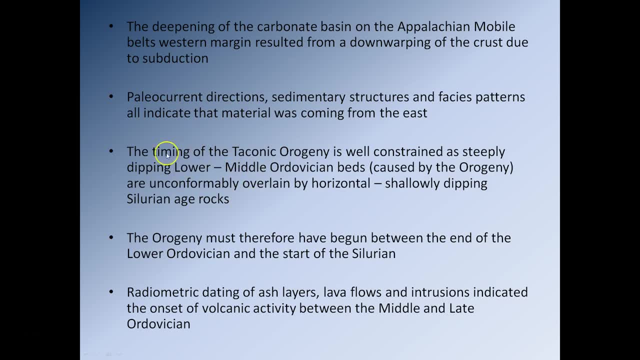 So we know we have these clastic sediments being deposited in the middle ordovician. We have the first indication of deformation actually coming in the lower ordovician, So that means the collision was underway by the lower ordovician. That starts. 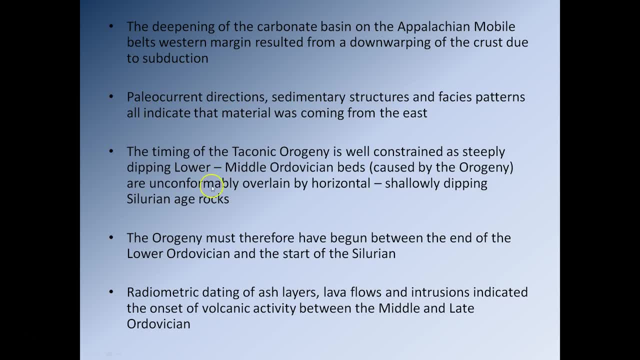 very, very early gentle deformation, and then by the middle ordovician we have the main event producing the ticonic highlands, and then, by the time we're into the silurian, the event has finished, because we now return to the deposition of nice shallow, almost horizontally dipping. 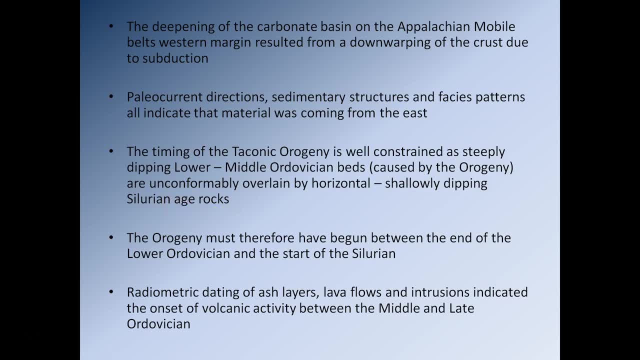 silurian age rocks, And so we have a very, very nice set of dating evidence for the timing of the ticonic orogeny. So the orogeny must therefore have begun between the end of the lower ordovician and the start of the silurian. 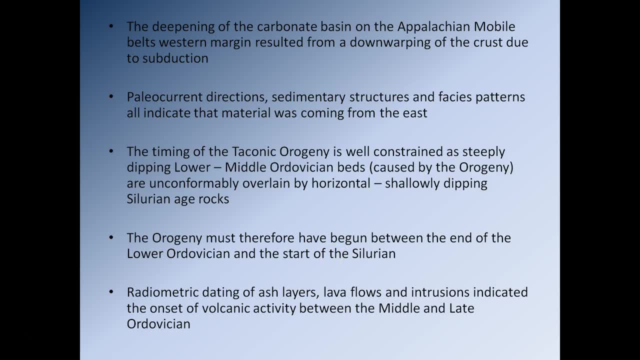 That's the range of time in which the ticonic orogeny occurred And we're lucky because the ticonic orogeny was associated with the formation of volcanic rocks. We can date those volcanic rocks and the volcanic rocks date essentially the ticonic orogeny. 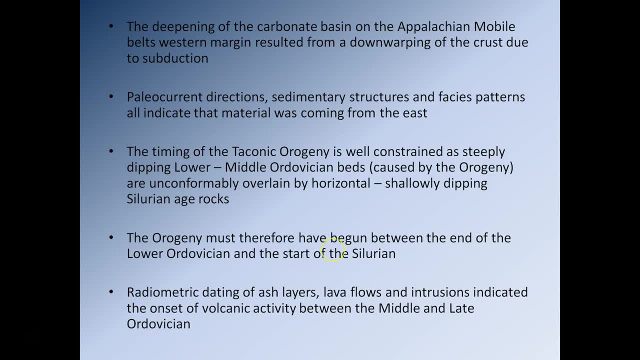 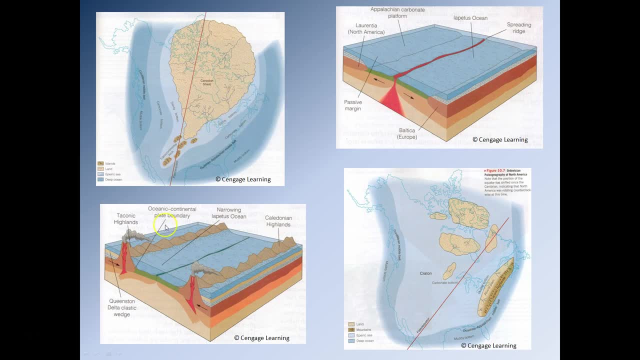 between the middle and late ordovician. So this kind of gives you some idea of what's going on here. So this is our situation. So this covers the formation of actually the closure of the Iapetus ocean. So now this diagram isn't 100% correct. 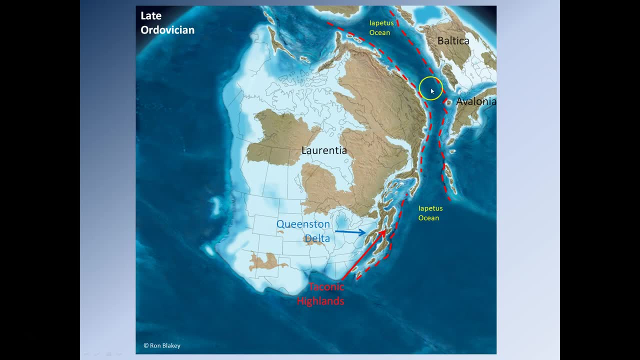 So if we look at this diagram up here, what we can see is the Caledonian highlands are actually forming up here. The ticonic highlands are probably more associated with the impact of this island arc, So this diagram here isn't quite right. 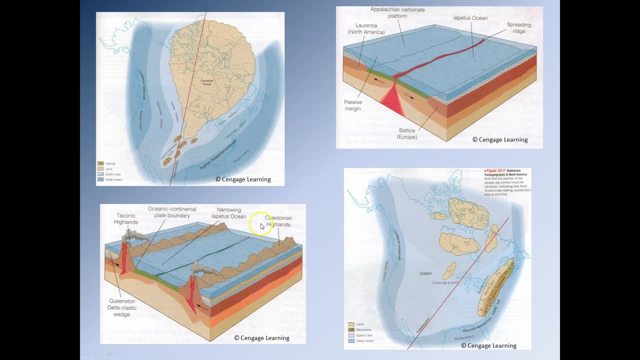 this diagram here suggests the ticonic highlands is actually being produced by the collision of Laurentia with Baltica and Avalonia over here. That's not quite correct, But the diagram itself is actually correct. We do have this body of water here. 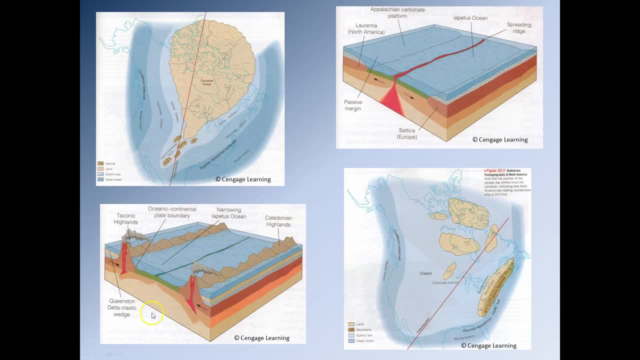 that separated essentially Laurentia from this volcanic island arc. Essentially the oceanic crust in between them was destroyed and eventually the two of them ran into each other, producing the ticonic highlands, And so the ticonic highlands are associated down here. 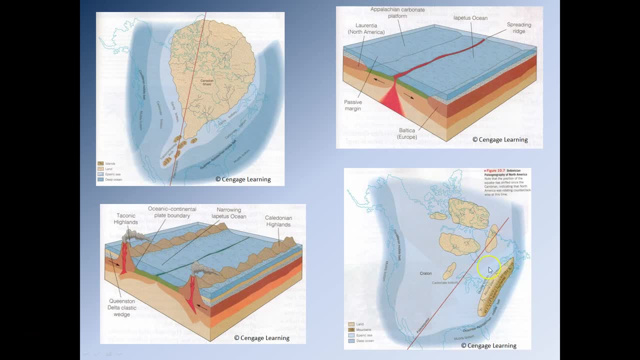 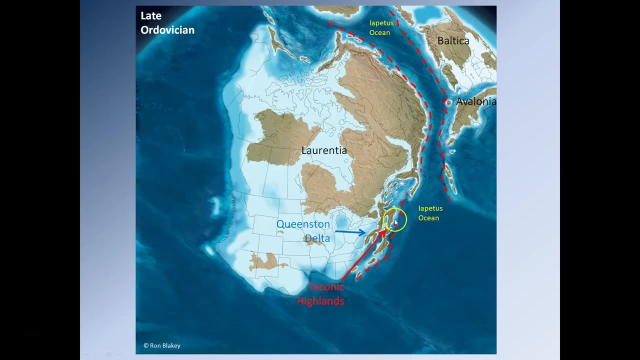 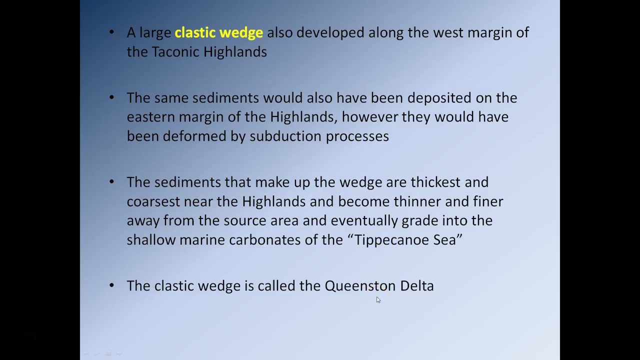 So we have the Caledonian mountains forming up here. The ticonic highlands are more associated with the collision of Laurentia, with essentially a smaller island arc forming down here off the east coast, So within this basin that forms along the western side of the ticonic highlands. 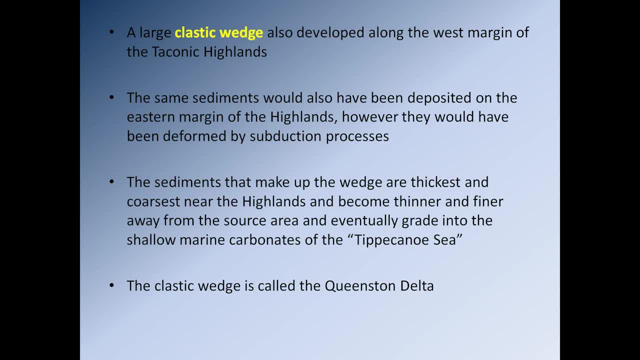 as you remember, the crust is being down, warped by all the sediment That leads to the formation of what we refer to as a clastic wedge. So a clastic wedge essentially is a wedge shaped package of sediments, And we see the same sediments that would have 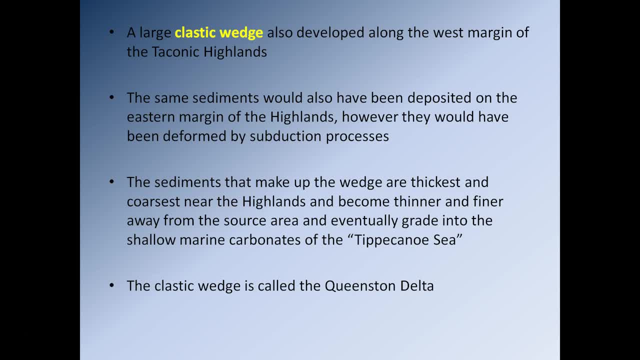 been deposited on the eastern margin of the highlands. However, sorry, the same sediments would have been deposited on the eastern side of the highlands as well. However, they were obviously destroyed by subduction. So we have a package. we have the clastic wedge forming. 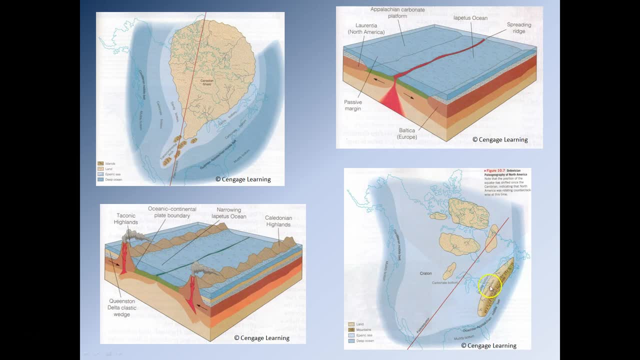 here on the western side, That's, from material being eroded off the highlands and moving into the Appalachian basin. here Now, we would have had the same sediments being deposited here on the eastern side, However, because this area here is an active subduction zone undergoing 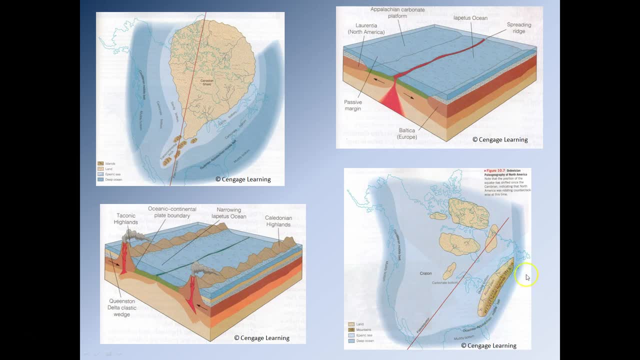 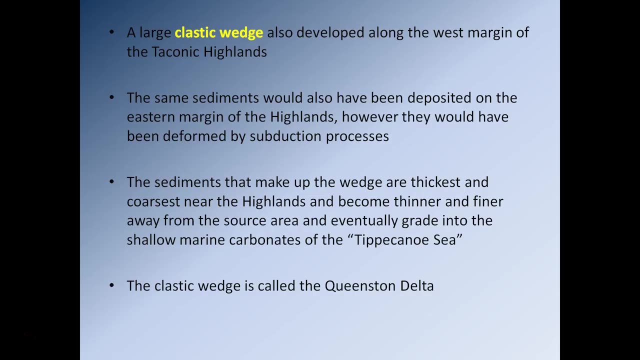 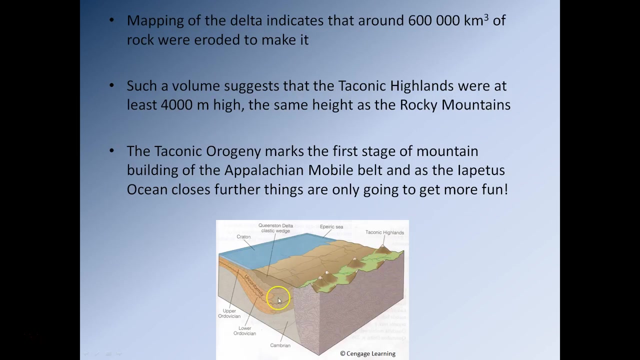 active deformation. those sediments just get mixed in and mucked around with as part of the subduction process, so we don't really see them that well. So the clastic wedge that forms is referred to as the Queenston Delta, And what we see is: 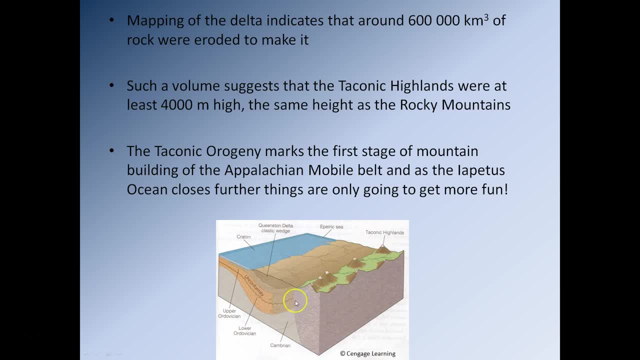 so these are the ticonic highlands here. The Queenston Delta essentially forms a sequence of sediments of the thickest closest to the highlands, and the layers of sediment get slightly thinner as you move towards the west, So that's why it has this distinctive. 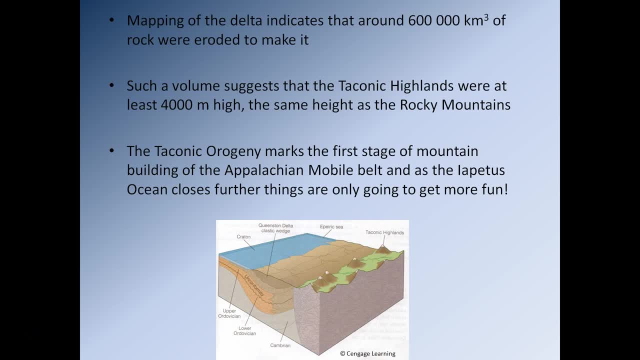 wedge shape. So mapping of the delta indicates that around 600,000 cubic kilometres of rock were eroded to make it, And such a volume suggests that the ticonic highlands were at at least 4,000 metres high, which puts them about the same height as the rocky. 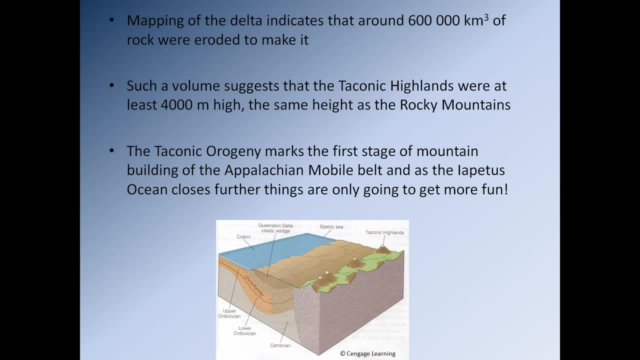 mountains. So they were a pretty substantial mountain range And the ticonic orogeny, of course, as said, marks the first stage of the mountain building that produced the Appalachian mobile belt. And as the Apatis Ocean closes further, things are only going to. 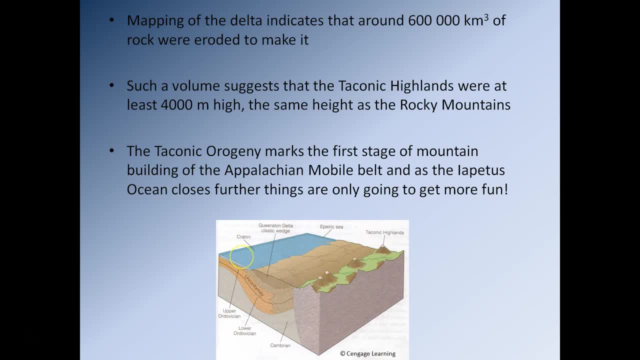 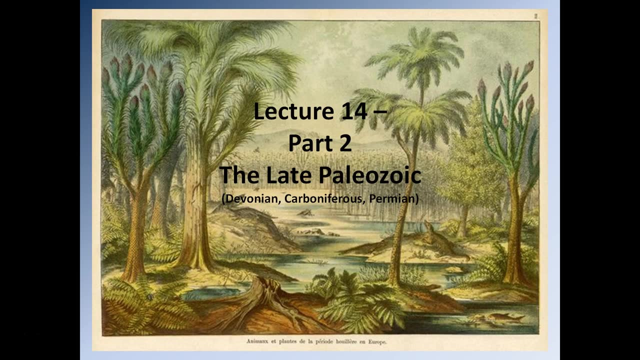 get more fun as Gondwana begins to get closer and closer. Okay, so this is where today's, this is where the second presentation, or the first presentation, ends. So the code word for this presentation is unicorn, as in the mythical beast. so that's unicorn. 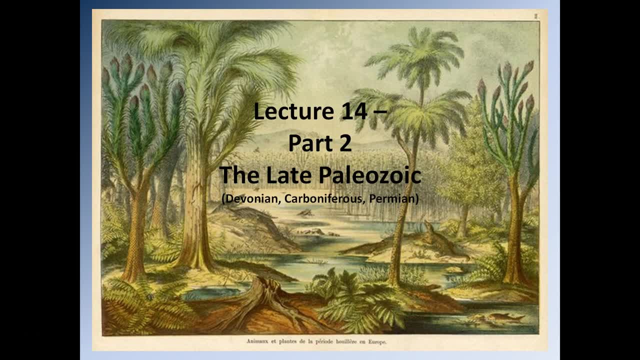 So keep an eye out for the second presentation coming. Alright, take care everyone.